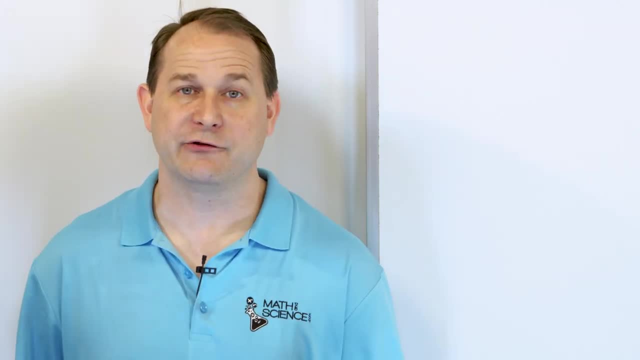 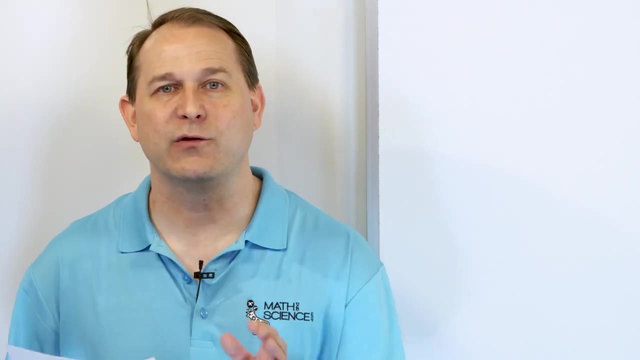 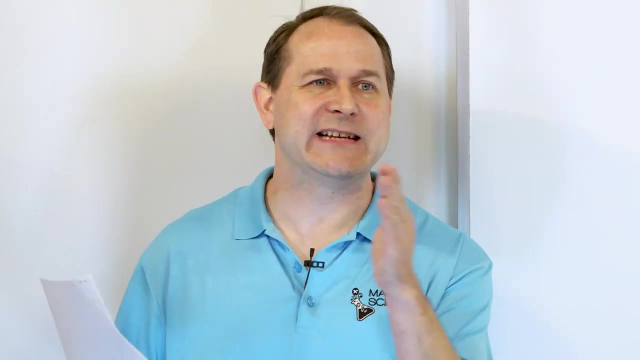 you will use this stuff all throughout algebra, all throughout trig and precalculus, all throughout calculus and definitely all throughout physics and engineering. So take a moment here and listen to what we're talking about, so you understand exactly how these things behave. Okay, Up until now we have been taking the sine, the cosine, the tangent, whatever. 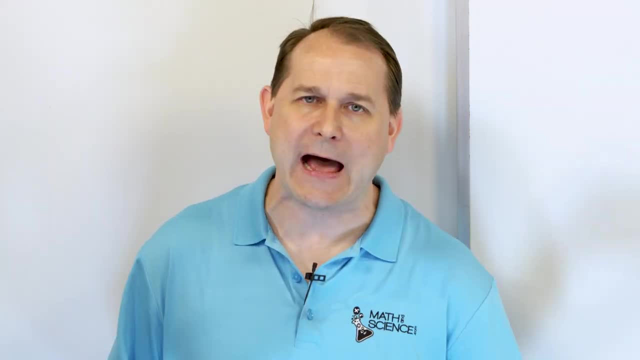 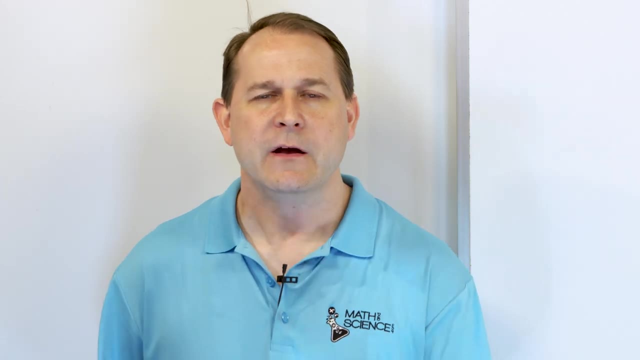 of an angle. So, for instance, sine of 30 is one half, which is the same thing as sine of pi over six radians is one half, because pi over six radians is 30 degrees. Okay, So in your mind think, sine of pi over six is one half, sine of 30 is one half. That's the direction we've been. 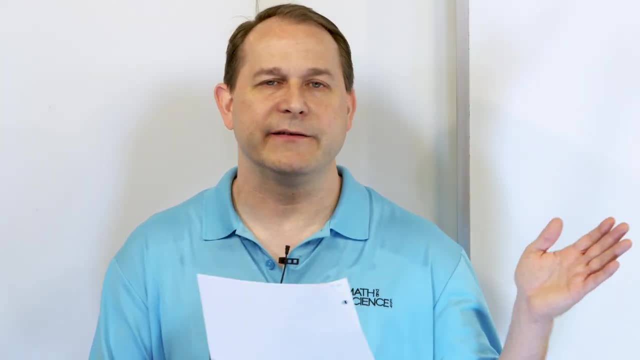 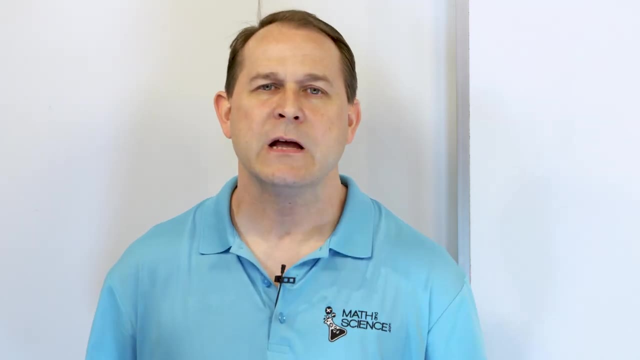 going. So there is an opposite operation to all of this And that's the direction we've been going. All of these functions called the inverse- Remember the inverse of a function just does the opposite. It kind of undoes the original function, right. So basically, the arc sine does. 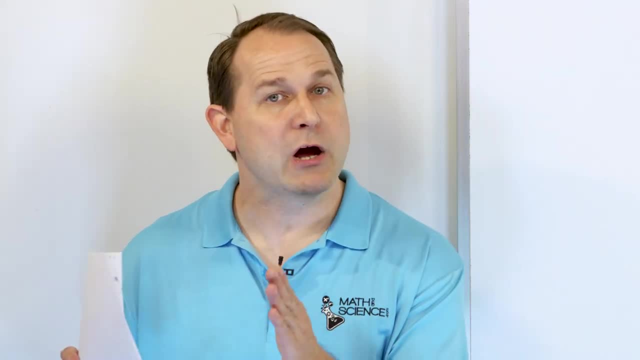 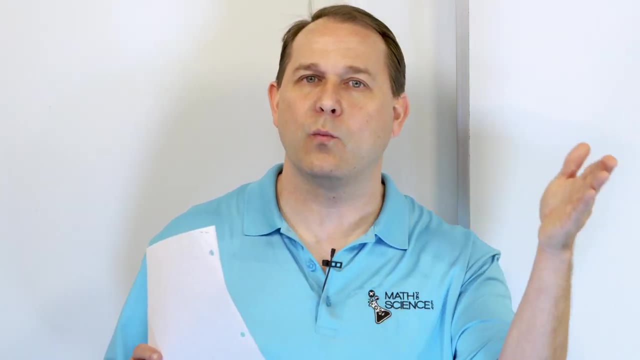 the opposite operation of the sine. So for instance, if you know- and I'm going to write all this on the board, so don't stress out here in the beginning, but verbally just follow me here- If you know that the sine of pi over six is one half, then you know that the arc sine of one half 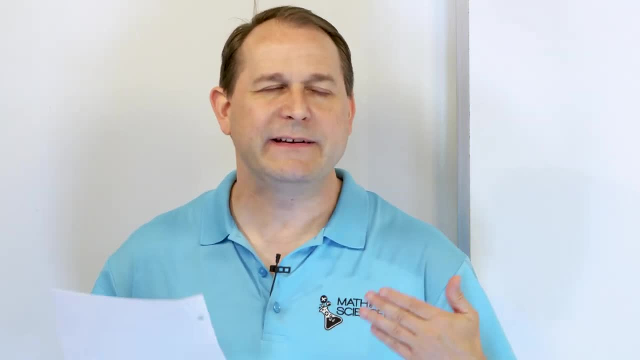 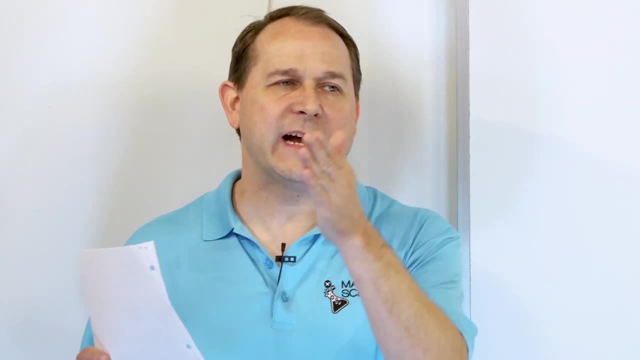 is giving you back an angle of pi over six. Let me say that one more time: When you do the arc sine operation of a number, you're asking for the angle back. So instead of taking the sine of an angle to get a number, we're going to take the arc sine of some number and get the 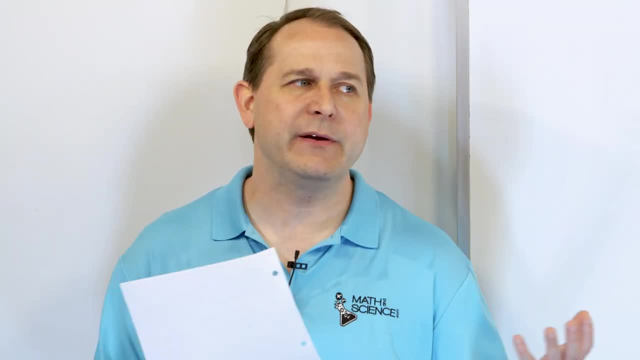 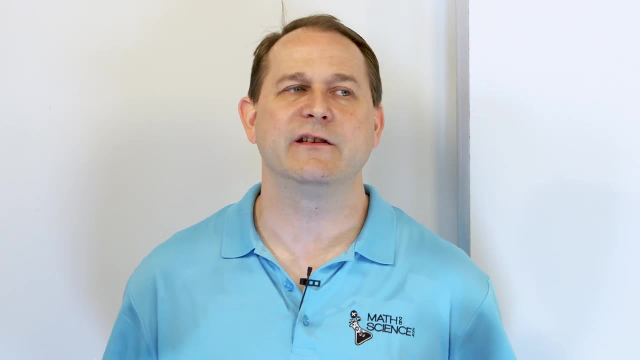 angle back. So it's the way that we find the angles, how we reverse, solve for the angles in a triangle or in an equation or whatever is going to be. basically the arc sine, the arc cosine, the arc tangent. It goes the opposite direction. So we're going to be taking the arc cosine. 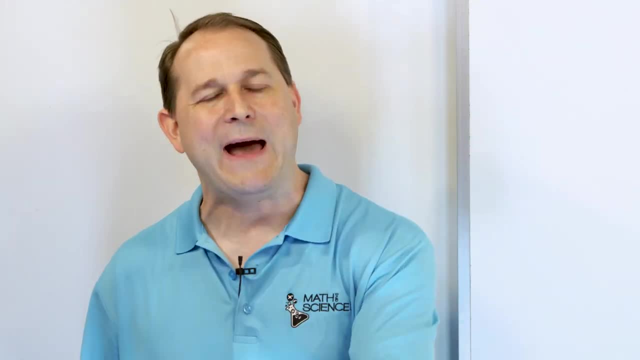 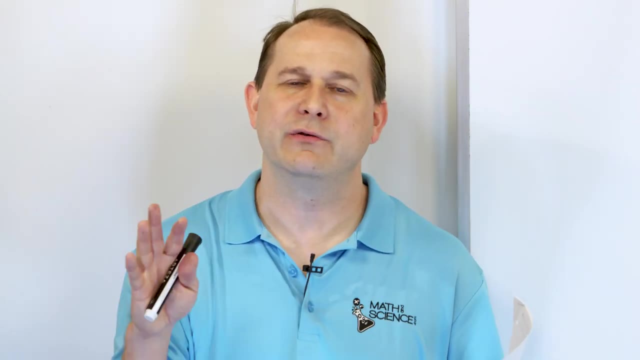 the arc tangent, the arc sine of some number and getting an angle back from it. However, as I mentioned, you need to trochę知 here, and that is the way the unit circle works. There will always multiple angles around the unit circle That can give you the same sine. 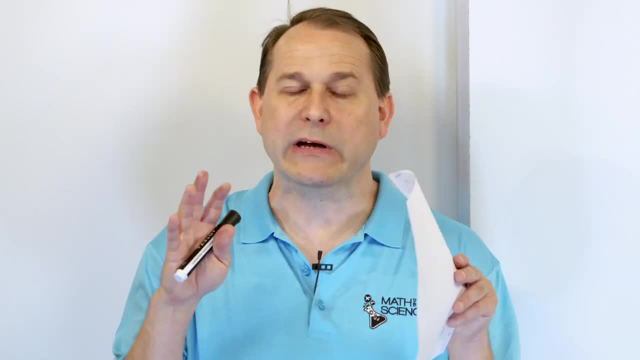 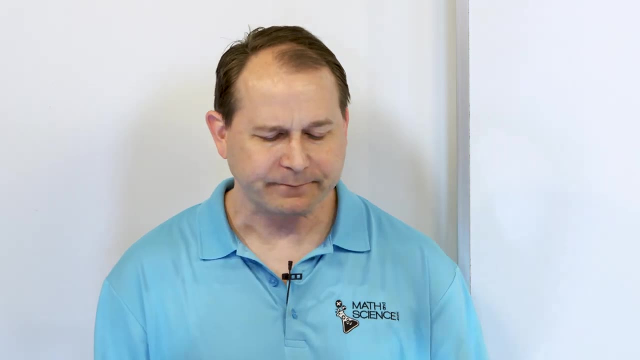 So there's always going to be multiple choices. So we have in your books you'll see exactly how we lock it down and to know what angles the calculator or the computer is going to give back to you. So we have to talk through that. So again, let me give you the punchline, then we're 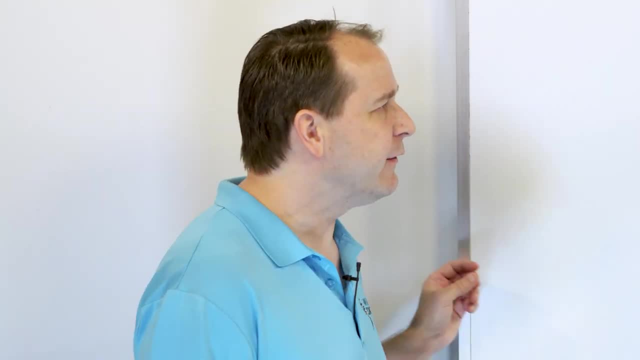 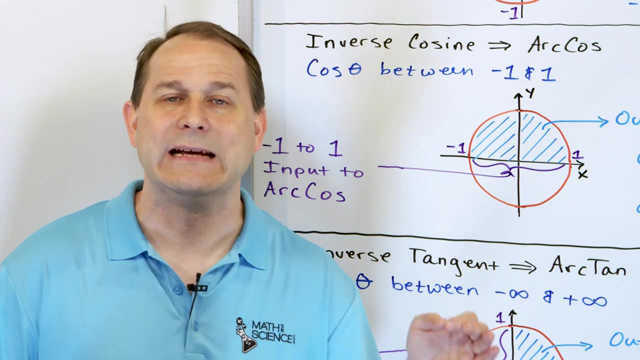 going to go through quite a detailed set of problems so that you understand exactly where it's coming from. want to know the punchline? I am not going to go through all of this right now because I'm going to go through it in detail in the lesson. But we have this function called the inverse sine, also called 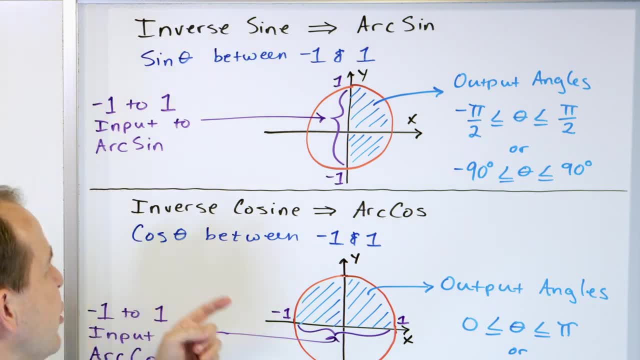 the arc sine. It is the opposite operation of a sine. You feed numbers into the arc sine operation and you get angles back. The numbers that you feed into the arc sine can only be from plus one to minus one. I'll explain why later. You put those numbers into the arc sine, you press the button. 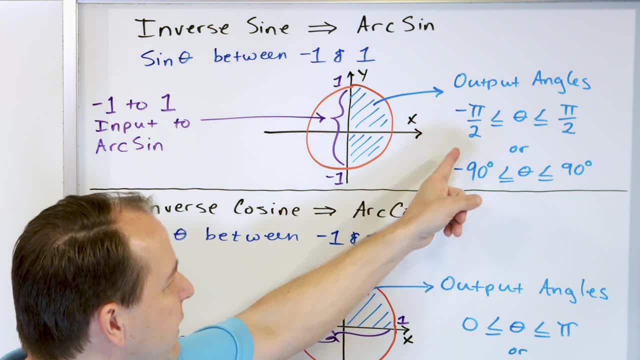 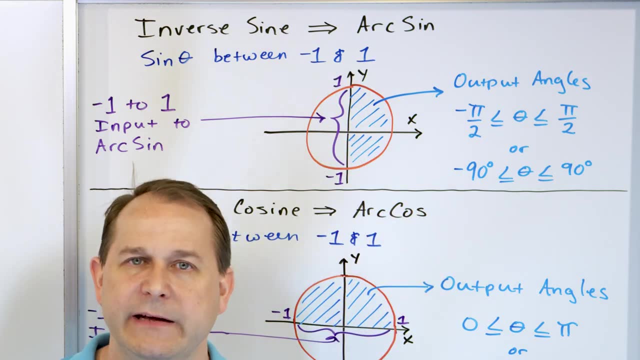 on your calculator out comes an angle, But the calculator will only give you angles from negative pi over two to pi over two. these angles over here. If you hit any inverse sine of anything on the calculator when it gives you an answer back, it will never be outside of this range: negative 90. 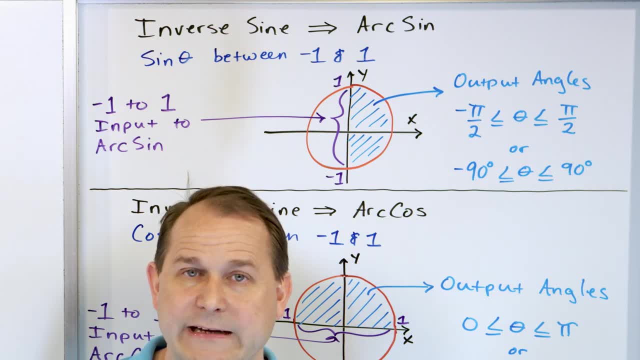 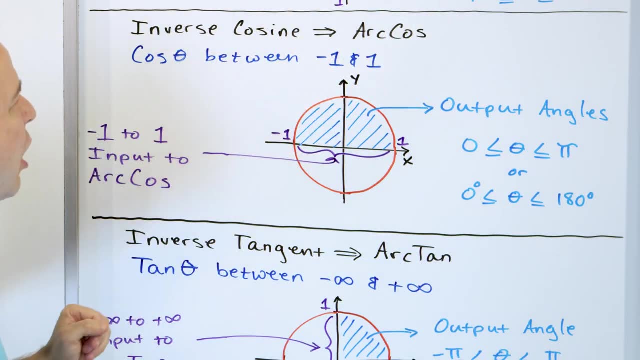 to 90 degrees, or negative pi over two to pi over two radians. I will explain exactly why as we go through the lecture here. Then we have an inverse cosine operation, also called arc cosine, Because the cosine can only be between negative pi over two and pi over two. it will only give you angles from negative pi over two to pi over two. 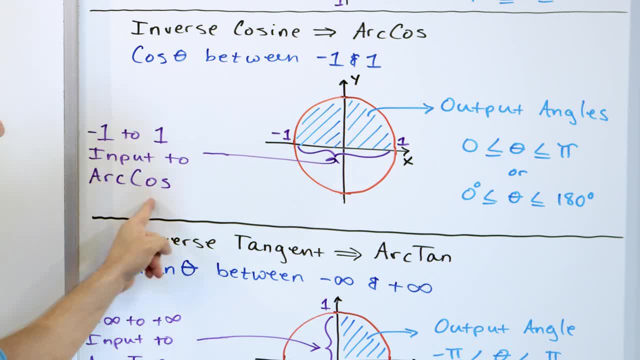 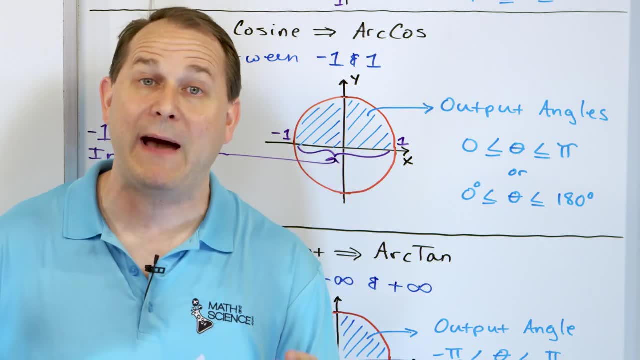 Negative one and one. I'll explain why in a minute. Then the input to the arc cosine function can only be between negative one and positive one, And because of that the angles that the calculator will give back as the baseline angles can only fall between zero and pi. 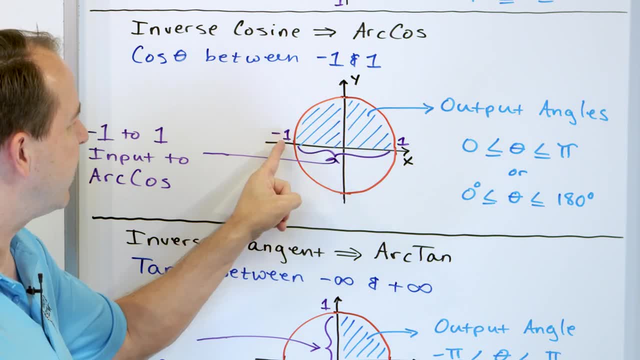 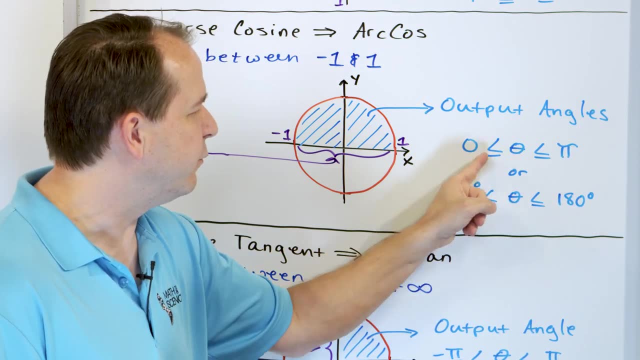 You see negative one, and one fall on the x-axis here. so the angles that you will get back will only be up here, in the top half of the unit circle: Zero to pi or zero to 180. That's what this means, But greater than zero less than pi. greater than zero, less than 180.. 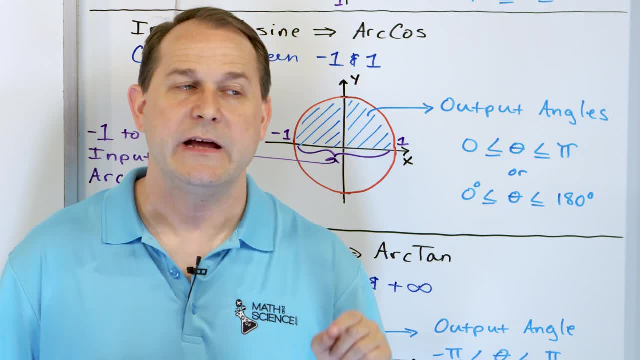 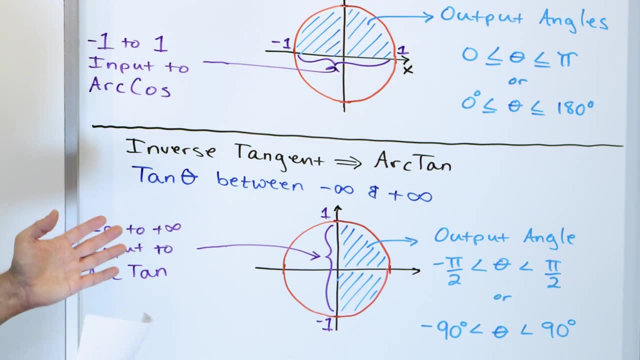 If you stick a number in your calculator and hit arc cosine, inverse cosine, you will never get an angle outside of that range. Arc tangent is the one that's really bizarre and weird and hard to understand at first. There's an inverse tangent called arc tangent operation. The inputs to the 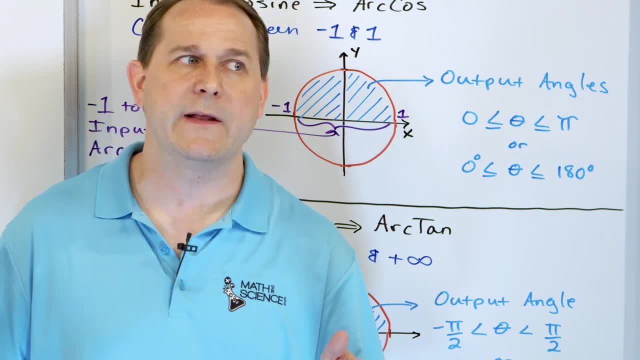 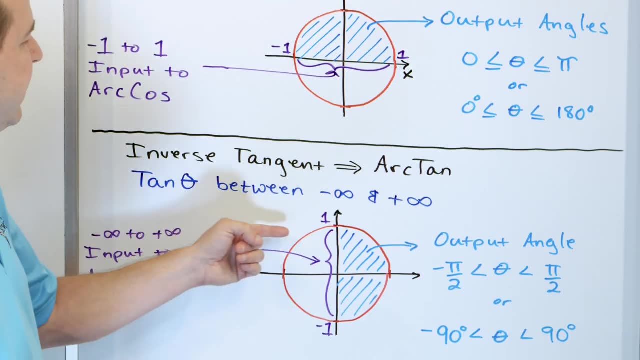 arc tangent can be way outside of the range of negative one to positive one. They can be negative infinity up to positive infinity. I will explain as we go through the lesson why that's the case. The numbers that you can feed into this operator: this is like a function, essentially here. 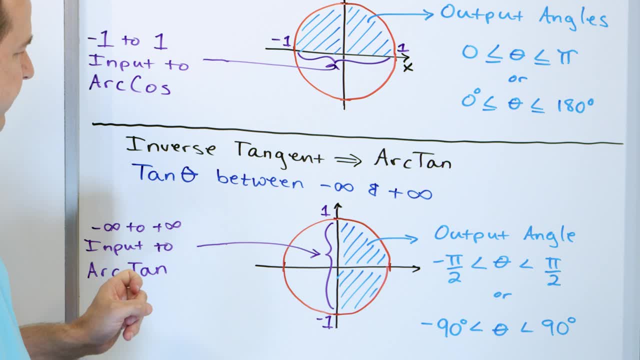 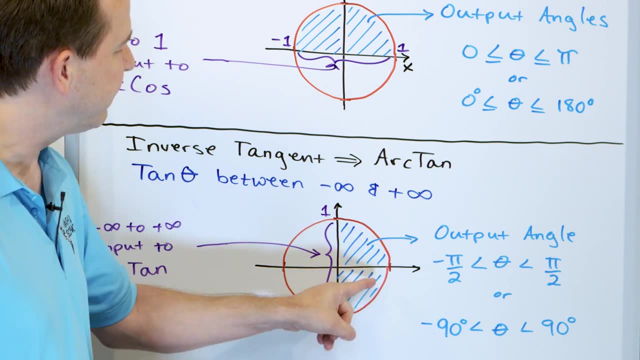 that you can put into. there can be any number at all, from negative infinity to positive infinity, but the angles that you get out of the arc tangent operation will only be between negative pi over two and pi over two, negative pi over two to pi over two or negative 90 to. 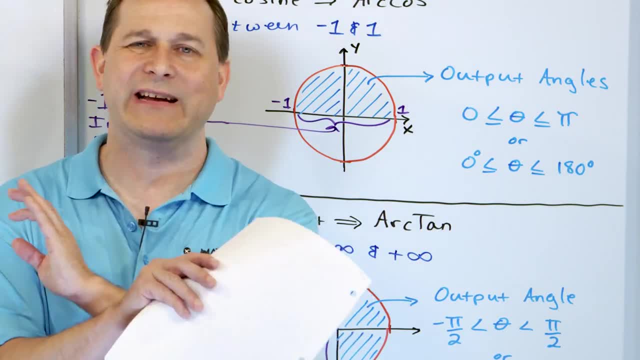 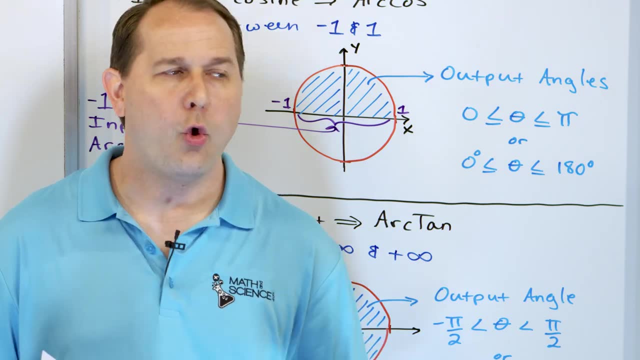 positive 90.. So this is the punchline. I don't expect you to understand anything other than the fact that when you do an arc sine operation, or you do an arc cosine operation, or you do an arc tangent operation, what you're getting out as an answer is an angle. 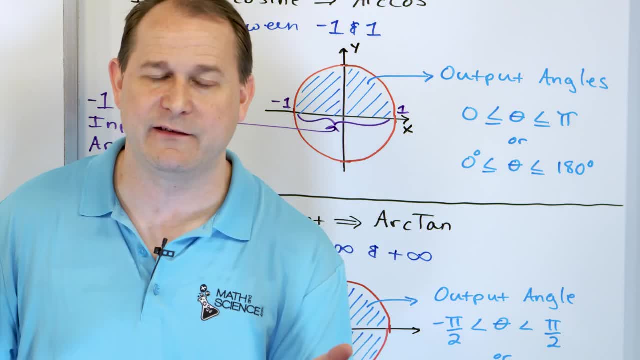 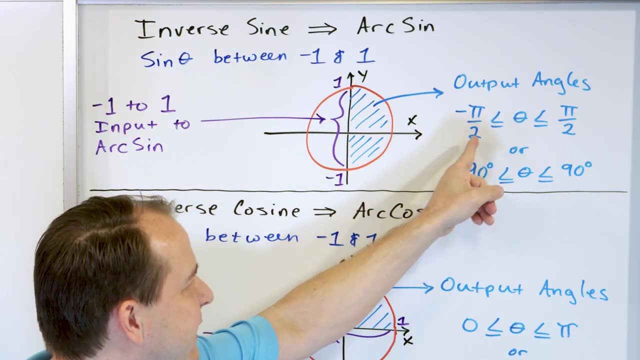 The angle that you get back out of each one of those operations has limits to it. Your calculator or computer will never give you an angle outside of those limits For an arc sine. you will always get an angle between negative pi over two or pi over two back, which is negative 90 to positive 90.. 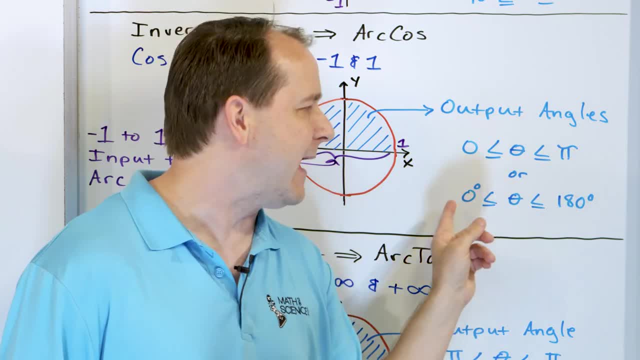 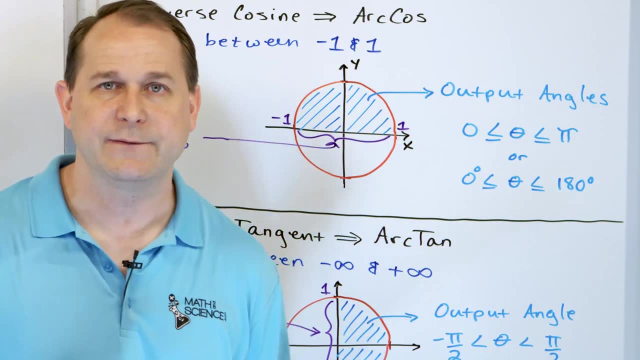 For an arc cosine, you will always get an angle between zero and pi, which means zero and 180.. For an arc tangent, you will always get an angle between negative pi over two to pi over two, which is negative 90 to positive 90 degrees. That's the punchline. 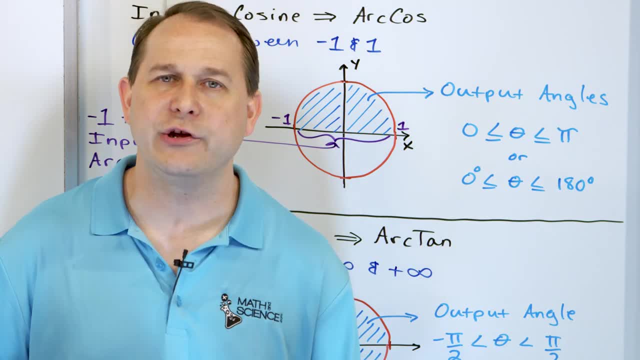 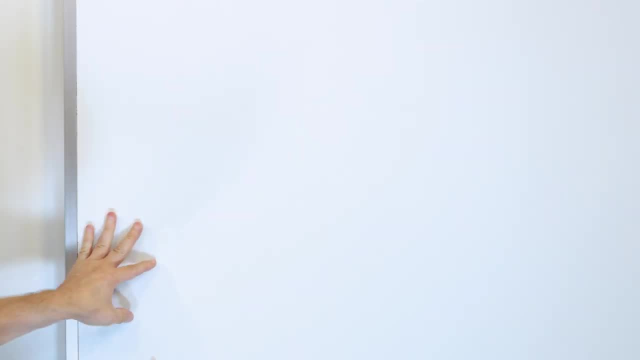 The question is: why is that? We have to dive into it? I don't want you to just memorize things, I want you to understand things. So let's cover this up. We will revisit this in great detail, I promise you, And let's go down and talk exactly through the logic of why all this works. It is more. 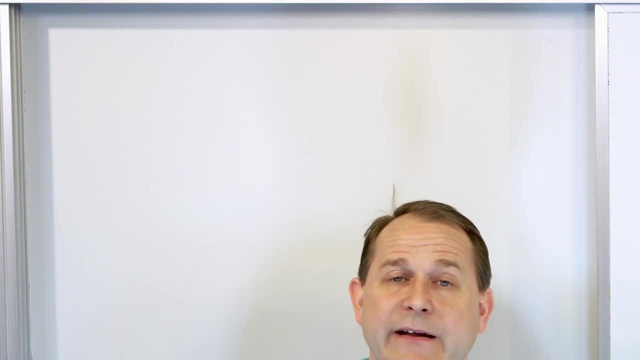 than a one or two minute thing. I can't compress it into three minutes, So please watch the whole thing and you will understand exactly the reasons why. All right, So we know. we know, for instance, that the sine of pi over six, which is 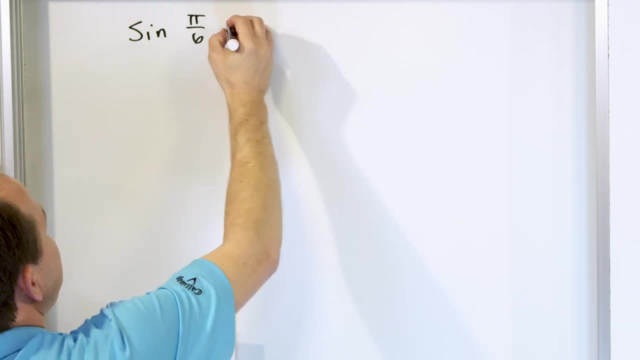 30 degrees. right, Remember, pi over six is 30 degrees is what You should all remember. sine of 30 is the famous one half. I've been telling you: sine of 30 is one half, sine of 30 is one half. 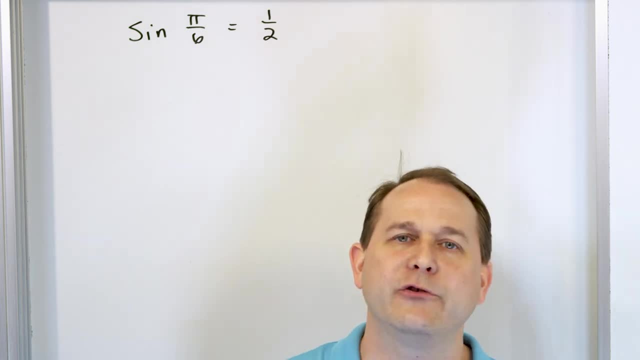 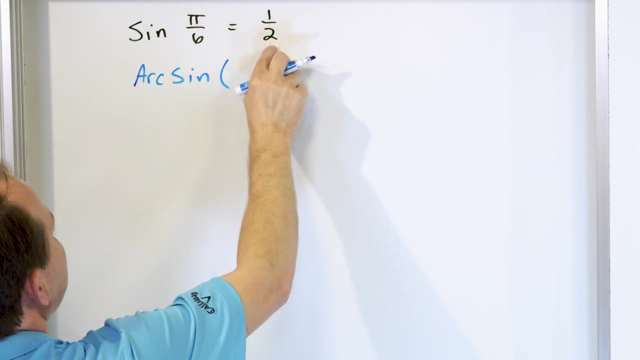 Now that we know radian sine of pi over six is one half. So how do we go backwards? If we know the sine of pi over six is one half, then we should be able to say the following thing: Arc sine, which is inverse sine, or the opposite operation of the sine of. whatever the kind of the answer is. 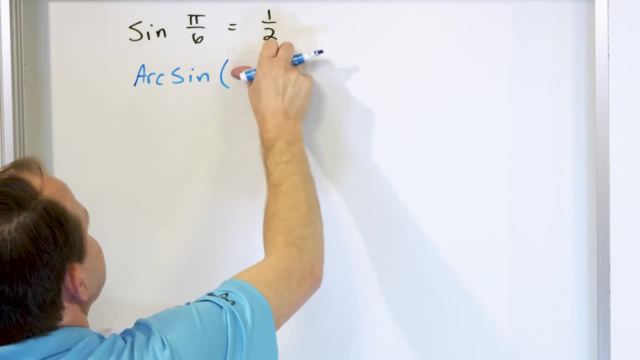 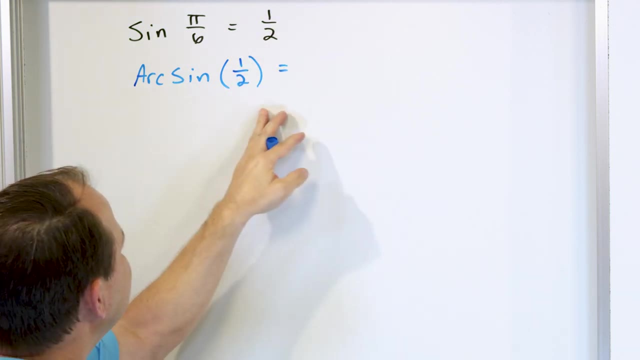 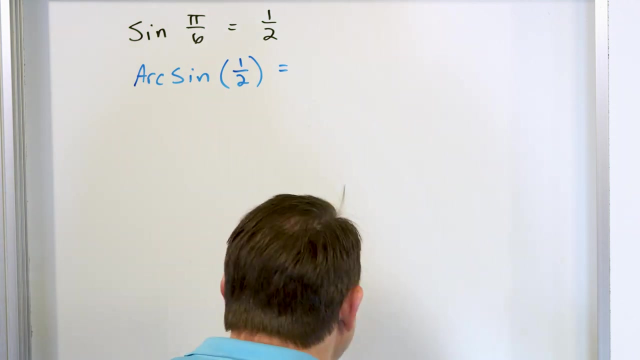 let me do it this way: Arc sine of- yeah, let me do it this way- Arc sine of one half is going to equal what angle? Like this is what this is basically asking you to do: Arc sine of one half is what angle- Another way to write this- you can kind of translate this problem, I mean. 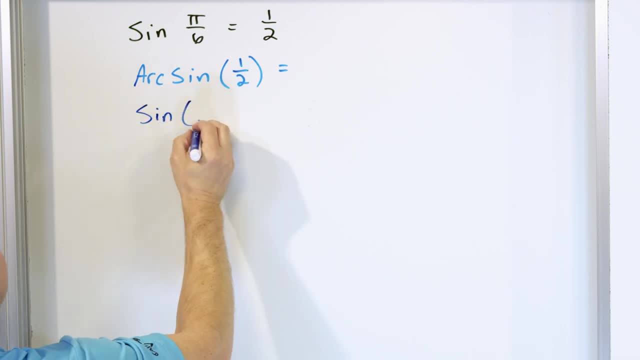 we've written it down here. but it's the same thing as saying the sine of some angle is equal to one half. When you say arc sine of one half, what you're really asking is sine of what known angle is equal to one half. And you know in your mind that sine of 30 is one half. So it 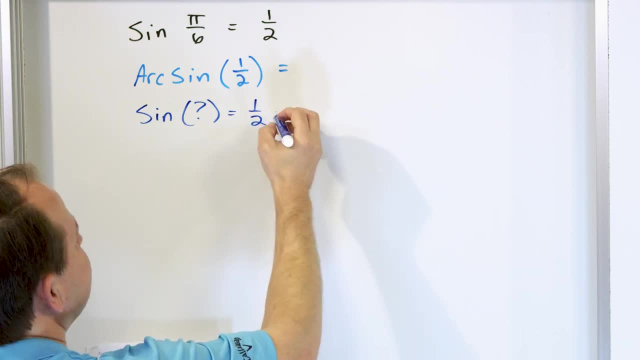 makes sense, right. Sine of 30 is one half 30 degrees, So we can then say that this angle is 30 degrees. but we don't like to talk about degrees too much now. So we say it's actually pi over six radians, right? So one way to write it is called arc sine. That's the cleanest way. 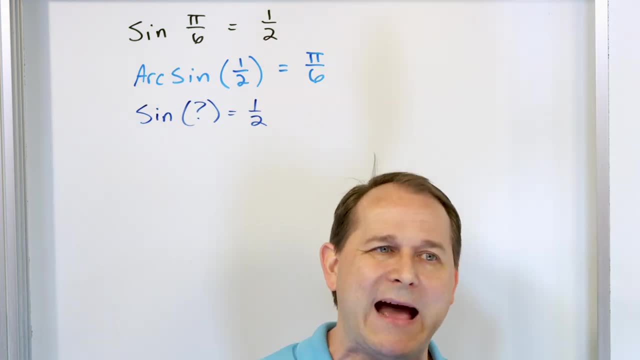 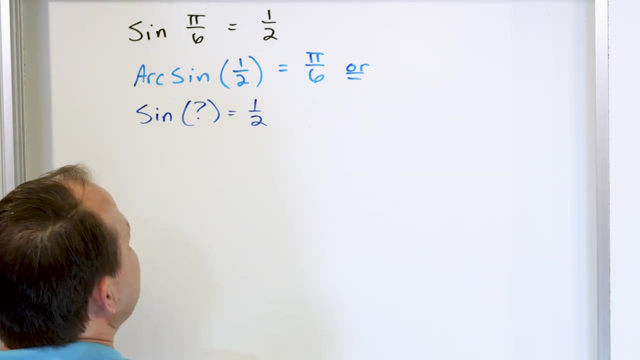 to write it That means inverse of the sine operation, going backwards. Give me the number, I give you the angle. That's what it is right. But you can also write this in the following way: You can write it in a different way and sometimes you'll see it. 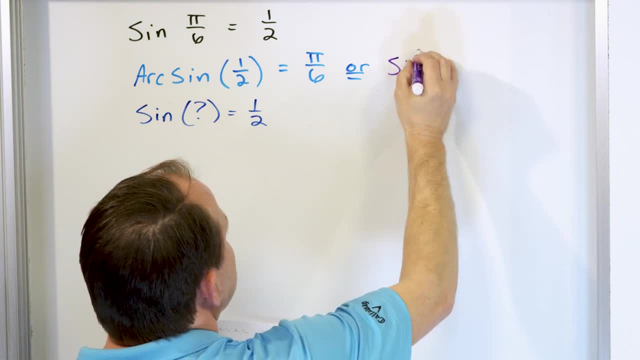 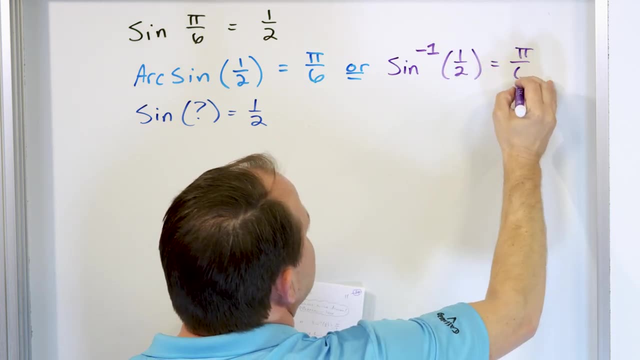 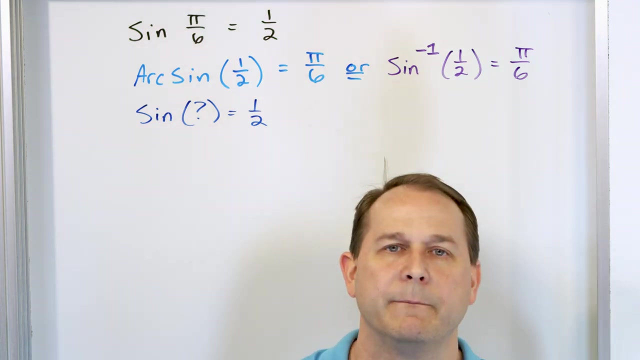 written like this in different books. You might see it written as the following: Sine- with a little negative one up here- of one half is equal to pi over six. This representation is exactly the same as this representation. So when you see sine to the negative one, power, it does not mean. 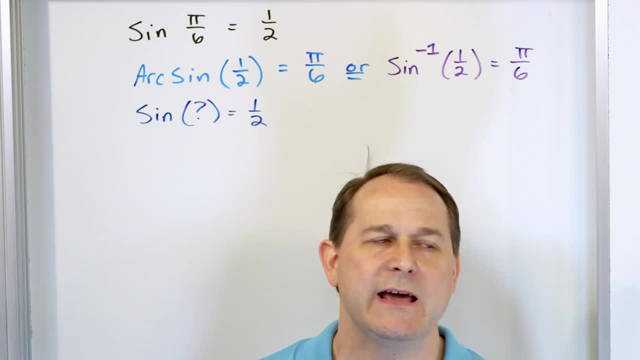 that it's raised to the negative one: power. It doesn't okay. It does not mean one over sine, okay. It doesn't mean that The negative one is not an exponent. The negative one is: if you remember back, we talked about inverse functions a long time ago. We said that negative. 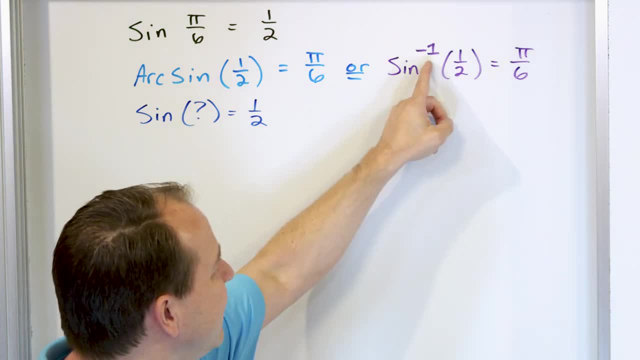 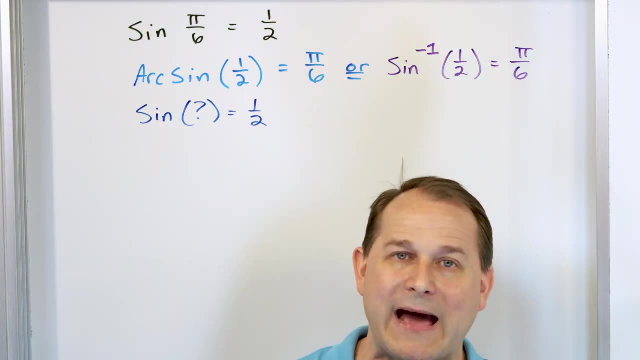 one up there can mean inverse function. So this literally means inverse function of the sine function. So this is the inverse sine of some number. gives me some angle Again going backwards. This is very confusing to write down because the negative one looks like an exponent. 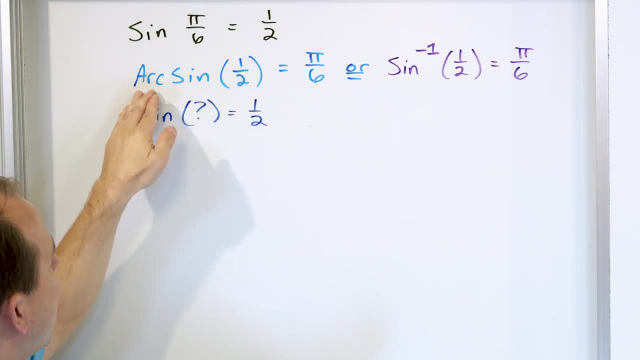 so it confuses a lot of people. So it's much more clean to say arc sine. but you can write it either way and you'll see it either way in lots of books You'll see in calculus or whatever. you'll see it written both ways, depending on the author. okay, 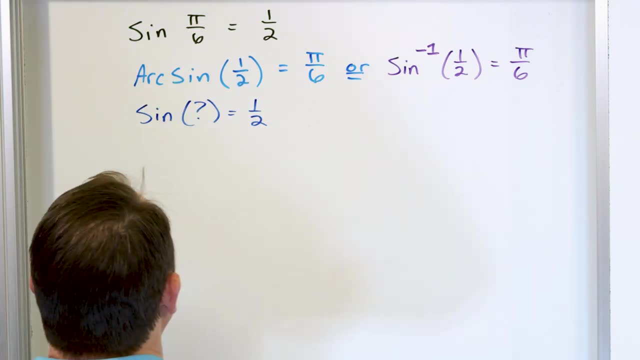 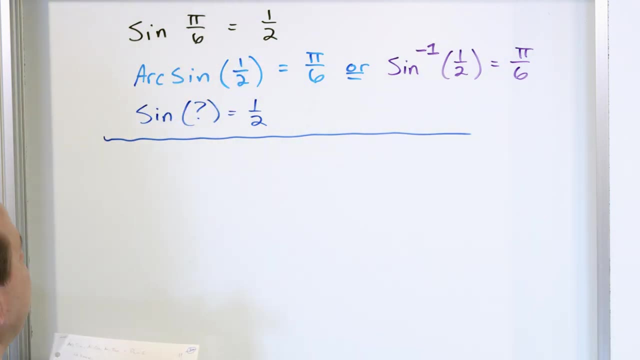 So it returns an angle back. Let's give another quick example, and then I'm going to show you the huge gotcha in here about why it's so confusing in just a second. So let's go and take a look at another one that we know very, very easily or very, very rapidly: What is the arc cosine of? 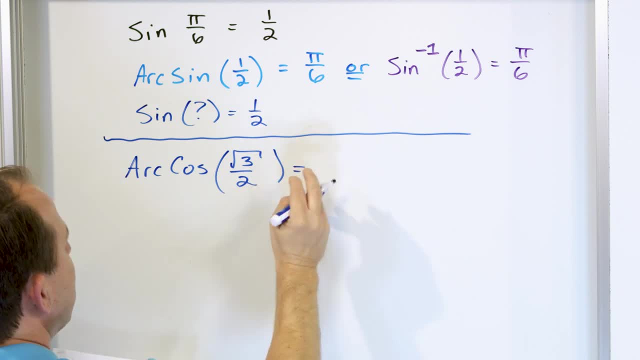 square root of three over two. So we want to figure out we have the inverse of the cosine function. That means we want to take as an input not an angle. We want to take kind of what the unit circle gives you around the outside. 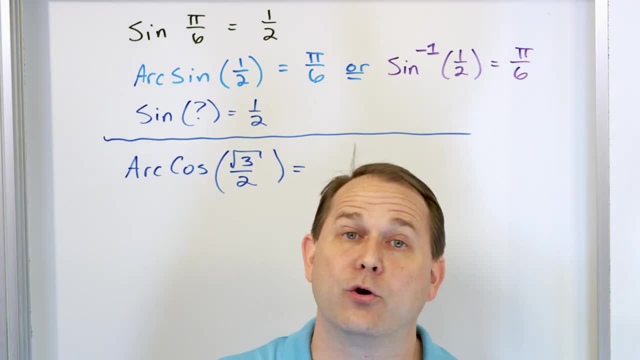 in red, the number coming off the unit circle, and I want to get the angle back. That's what the arc cosine, the arc sine, does for us. So what you can do in order to kind of translate this in your mind, is you can then say that this is the same thing as saying that the cosine of some unknown angle 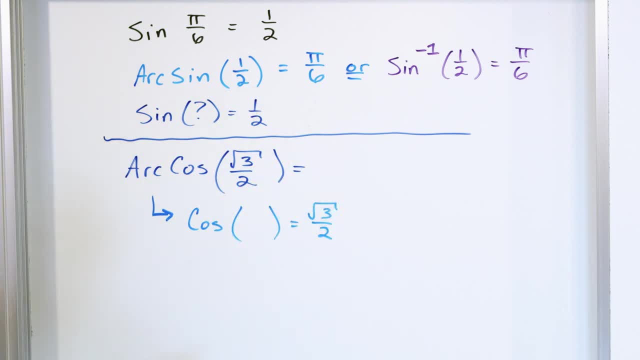 is the square root of three over two. The angle is what you're kind of getting here. So the cosine of what angle here is going to do that. The cosine of pi over six degrees is the square root of three over two, which means that kind of. 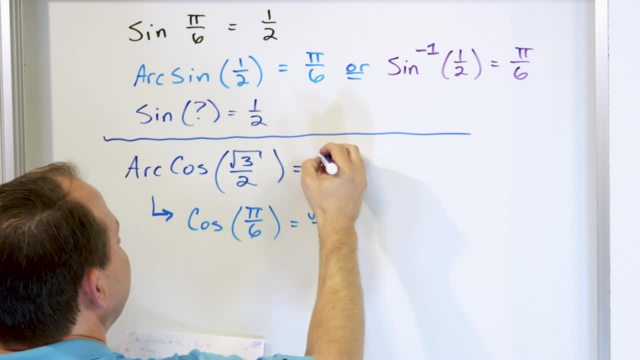 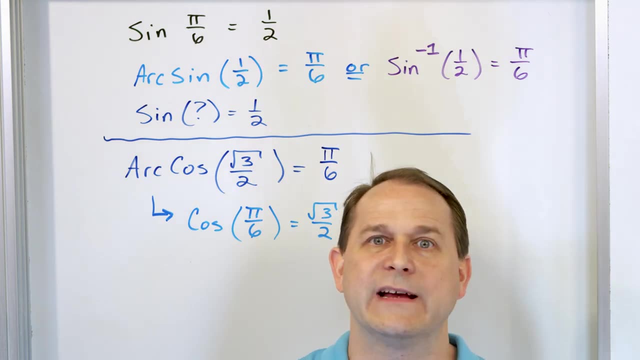 coming up and translating up here: the arc cosine of square root of three over two is the angle pi over six or 30 degrees. How do we know that? Because we know the sine of 30 degrees is one half. The cosine of 30 degrees is the other number, square root of three over two. So the 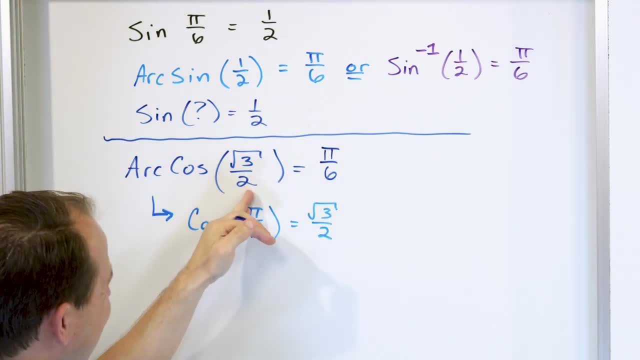 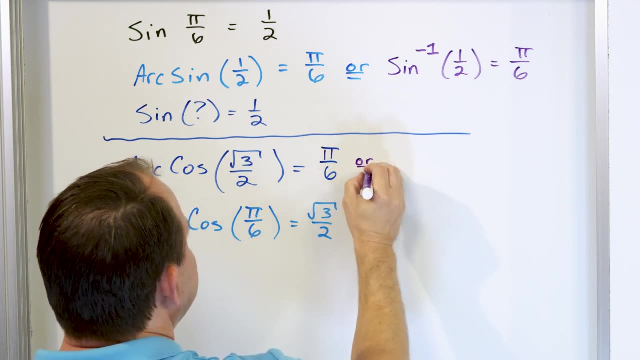 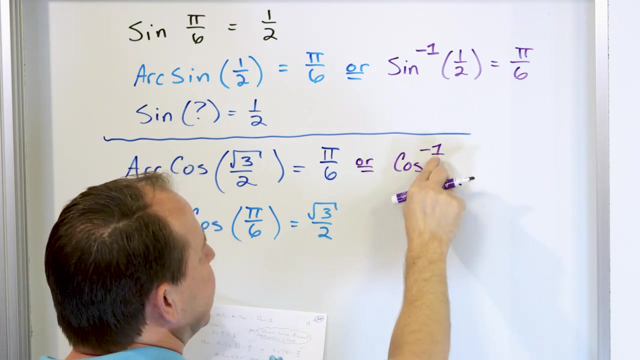 cosine of 30 degrees, square root of three over two, which means the arc cosine of the answer is the angle Coming back. Okay, And of course, another way to write this that you might see in other books down the road. another way to write this is the cosine inverse. This means inverse. cosine does not mean. 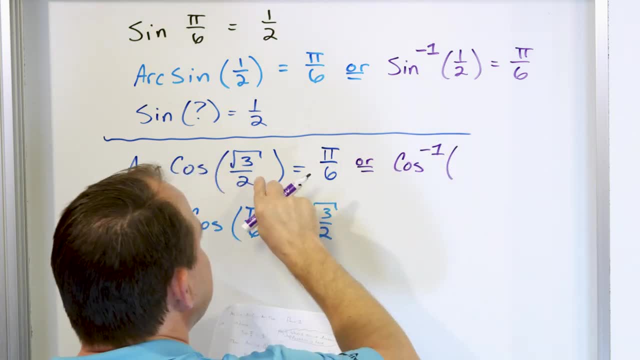 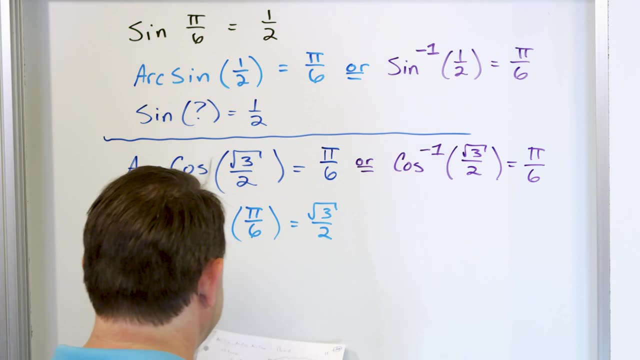 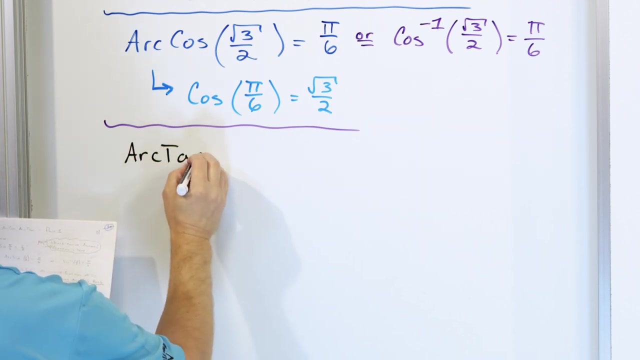 one over cosine or cosine to the negative. one power of the number square root of three over two is the angle coming back, pi over six. Okay, Pi over six. So that's another example. Let's do another quick example here that we can talk about. What about arc tangent of square root of? 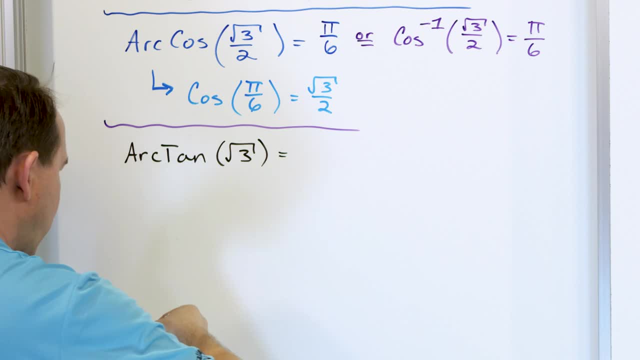 three. Arc tangent of square root of three is equal to what? Another way to do this is to translate it in your mind When you see arc tangent of a number. the way you do it in your mind or on your paper actually is you say the tangent of some unknown angle that I don't know is going to be equal to. 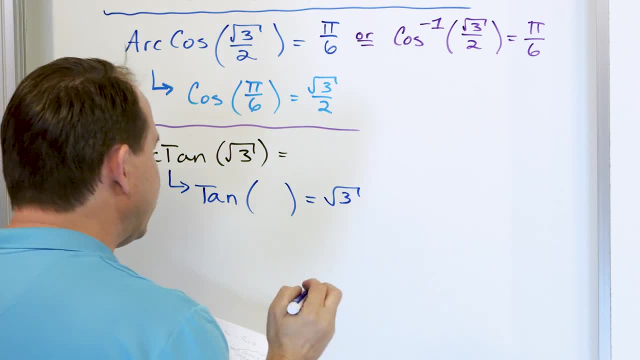 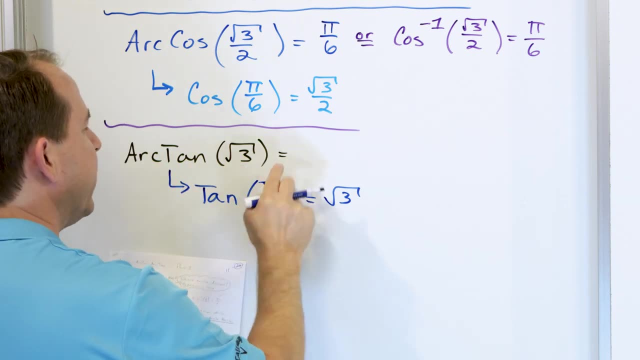 the square root of three. Okay, Now the angle that actually works here is going to be equal to the square root of three. Let me just show you now. So the angle that will work here is pi over whoops, pi over three. So the answer to the arc tangent of this, going backwards, is the angle pi over three. 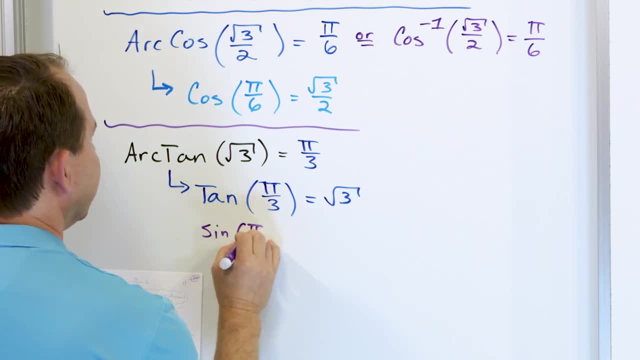 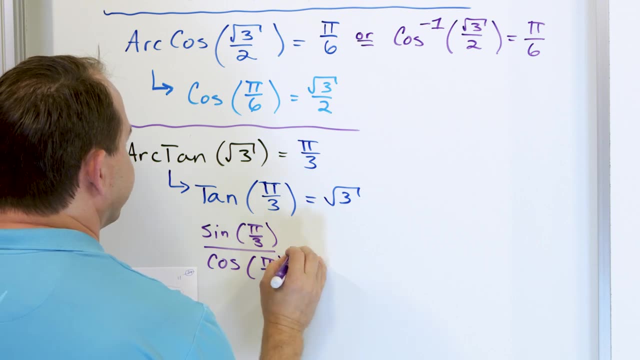 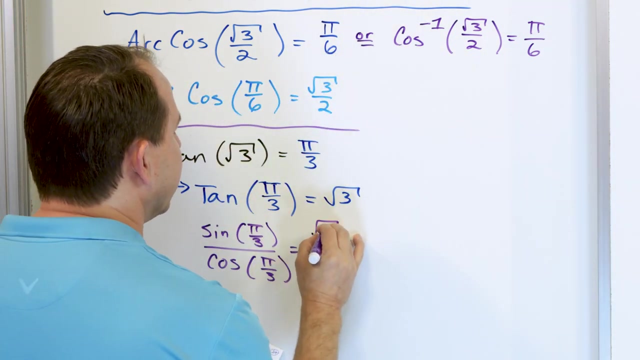 Right. How do I know it's pi over three? Well, I know the answer, but the reason is because the tangent is the same as the sine. So put sine of pi over three over cosine of pi over three. What is cosine of 60 degrees is the square root of three over two, And then the cosine of 60 degrees. 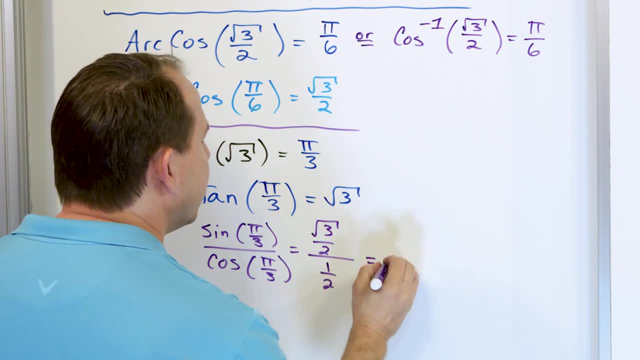 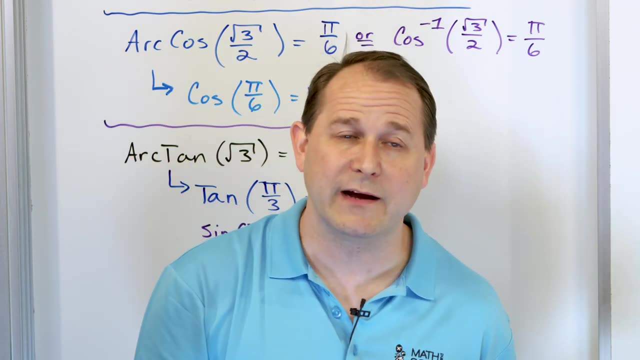 you know, is one half. If you flip and multiply, the twos will cancel And what you get back out of it is the square root of three. So you have to bust this tangent up into a sine and a cosine to figure it out, unless you have it memorized. I don't actually have them memorized, So I have. 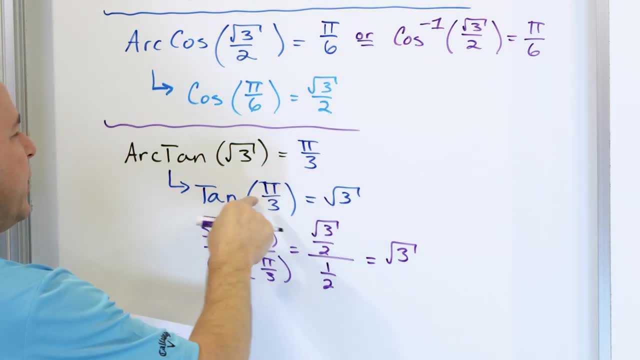 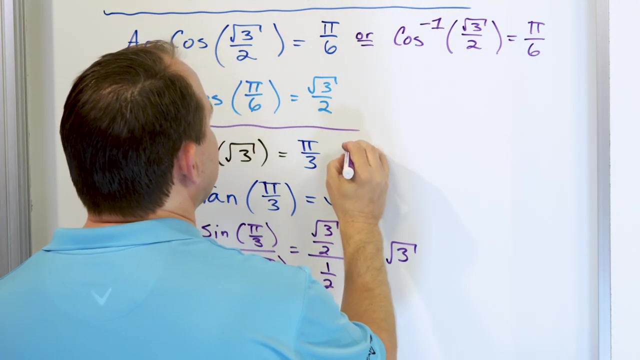 to go figure it out that the square root of three is the result when you take the tangent of pi over three. So because of that, the arc tangent of the pi over the square root of three number is the angle pi over three. All right, And you can also write this in another way. You can write this as: 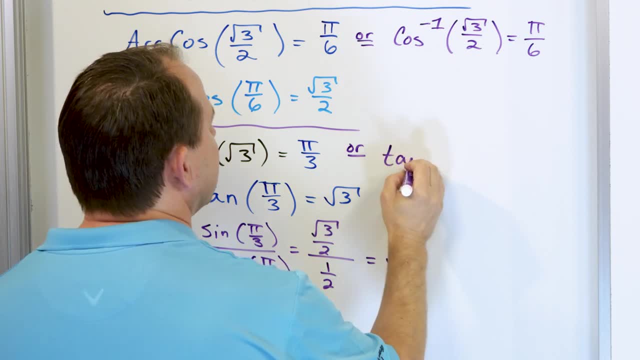 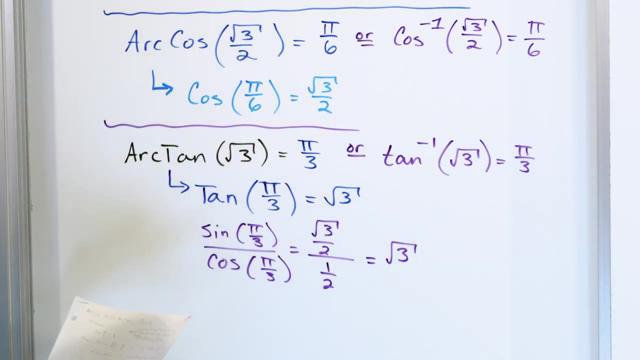 or tangent inverse of square root of three is pi over three, pi over three, All right, So arc tangent square root of three is the same thing as inverse tangent written with a negative one of square root of three. Do not write this or think that the negative one is an exponent. Do. 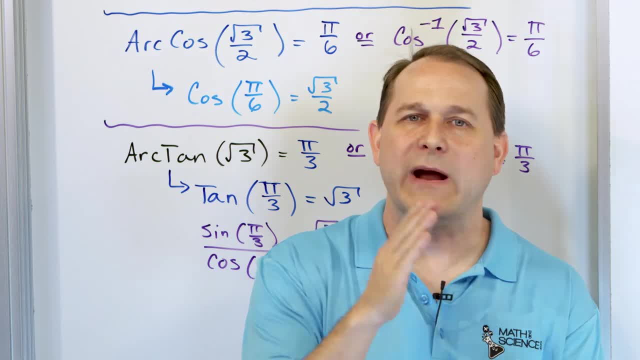 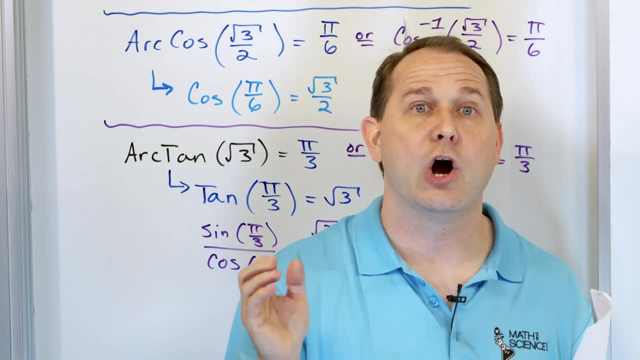 not try to add exponents, Do not try to subtract exponents, Don't raise the exponent to a square root and cancel them. Don't do any of that stuff, because it's not a real exponent, It's just a notation. that means arc tangent or arc sine or arc cosine. That's what it means. Now, the last. 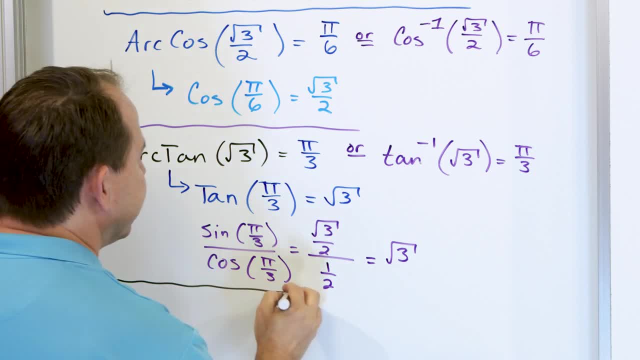 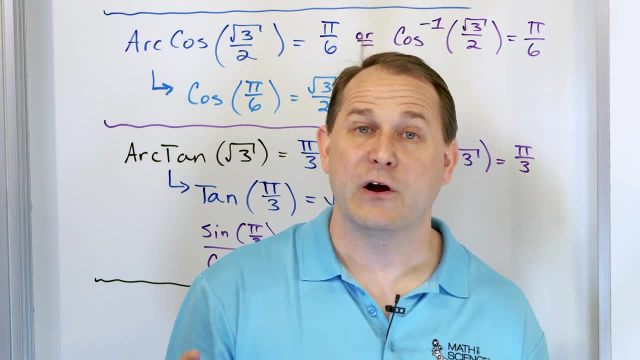 thing I want to leave you with, before we go into the details of why this is kind of so confusing, is the following thing: You know, a long time ago I introduced the concept of a function as a box. A function is a box. You stick numbers coming into this box. 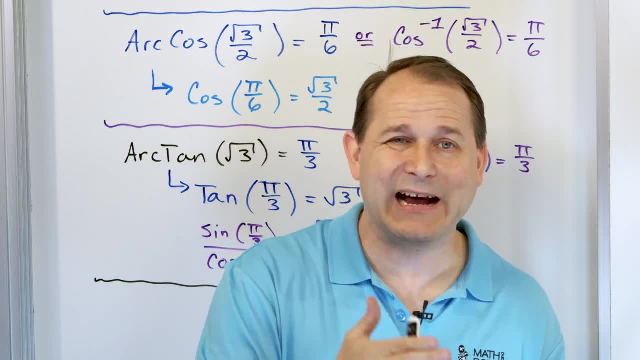 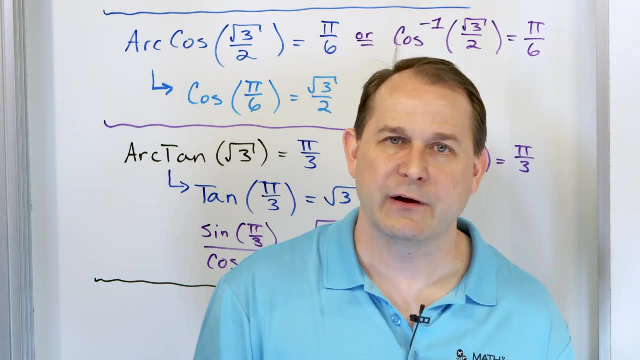 Inside the box is a computation. Could be any kind of function. X squared could be the function, 3x plus four could be the function. Could be a linear function, Could be a quadratic function, Could be a square root as a function. All kinds of things can be in the box. 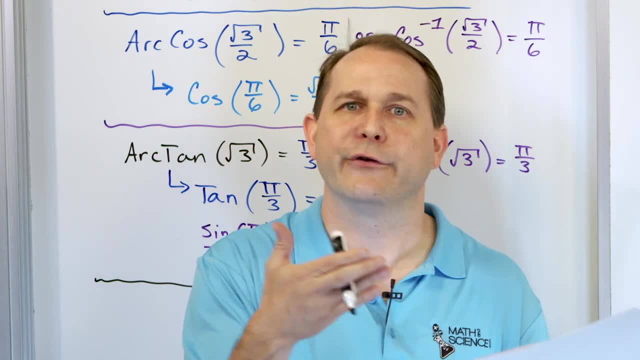 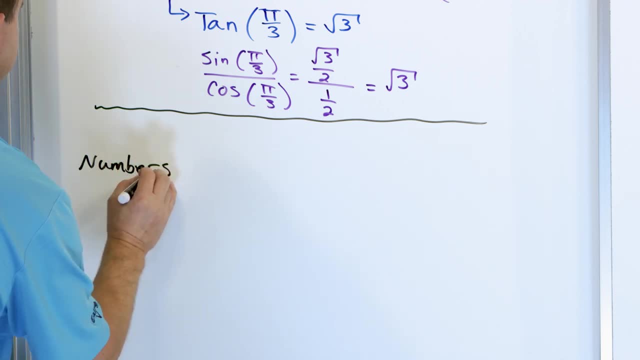 Now we're learning a new kind of function, basically, and it's called the inverse sine or the inverse cosine. So basically, what you have is you feed numbers, not angles, just numbers. You feed numbers into this box, And what is inside of this box, This box that I'm 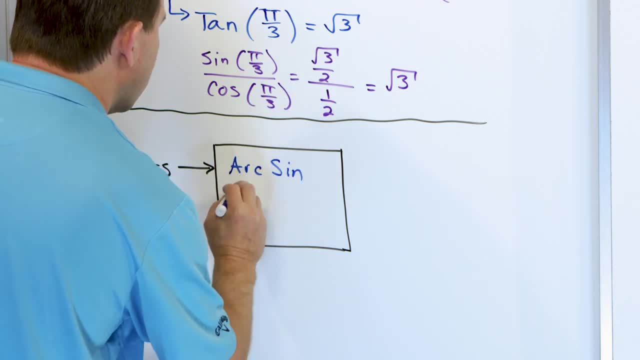 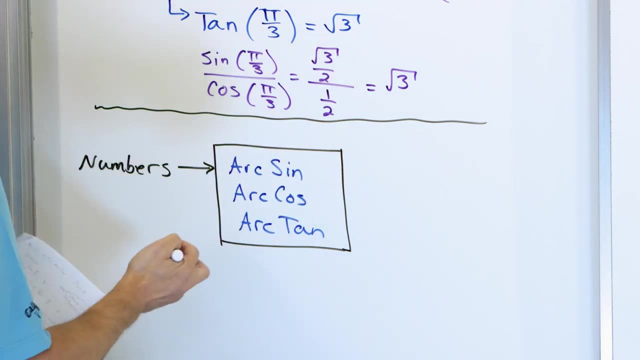 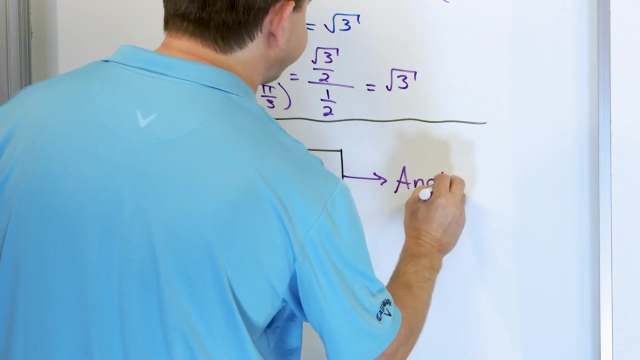 going to represent right now is arc sine or arc cosine or arc tangent. So I'm putting three different functions here as examples, but the punchline is: what comes out of the box? Angles come out of the box. It's actually really easy to get confused. 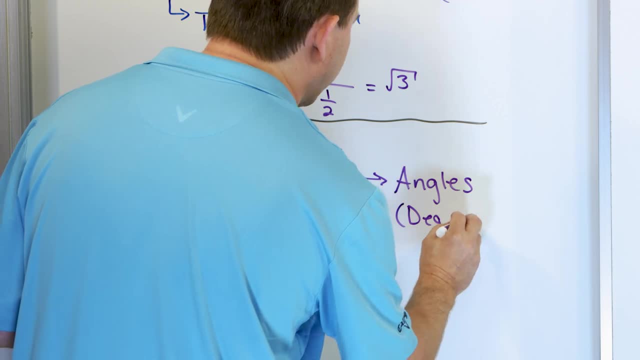 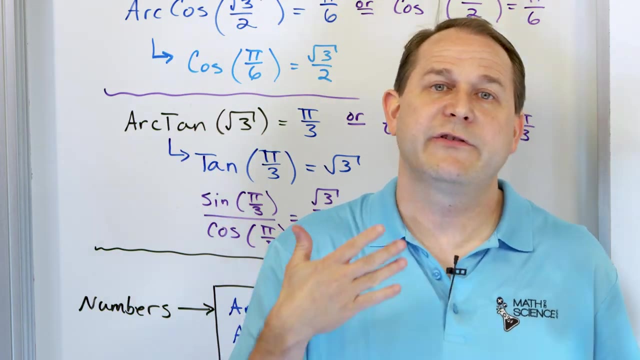 So I'm writing it down here. And of course you can get degrees if you're working in degrees or radians. So when you're taking an arc sine or an arc cosine, you need to expect degrees coming out or you need to expect pi over six, three, pi over four radians coming out. Keep it in your mind. 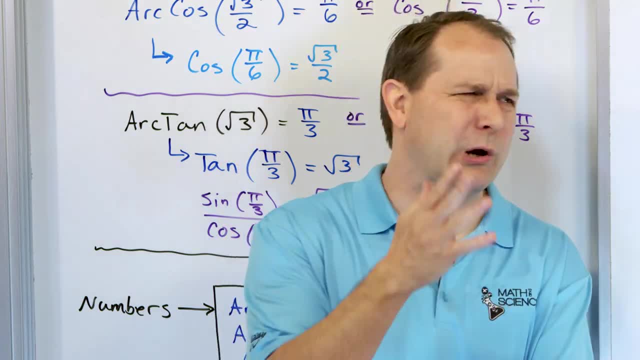 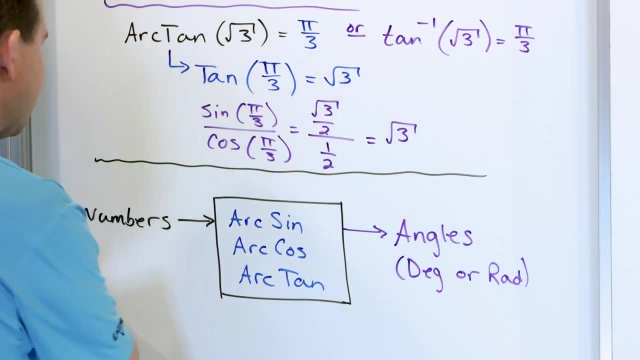 because, even though I know that you know this, it gets confusing when you start doing arc sine, arc cosine, all this stuff, that you expect angles to come out. Sometimes we forget what we're doing. So numbers come in. We're going to talk a lot about the numbers that are allowed to come into. 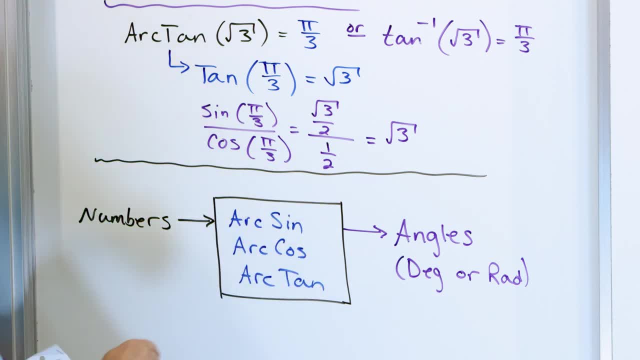 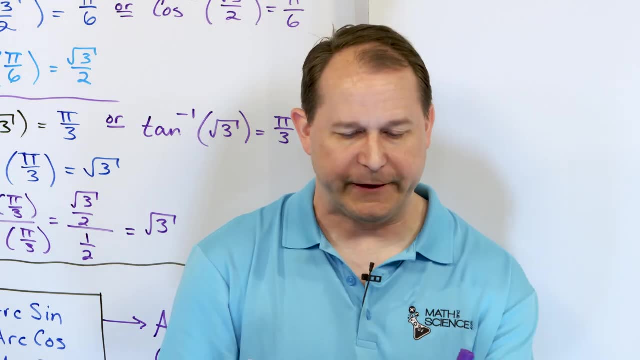 these boxes. Boxes contain arc sine, arc cosine, arc tangent, and the output of these boxes are basically angles. You're getting degrees or radians, All right. So we're done with the first part here. Now the tricky part is what's coming up next, The punchline, the gotcha that I really want. 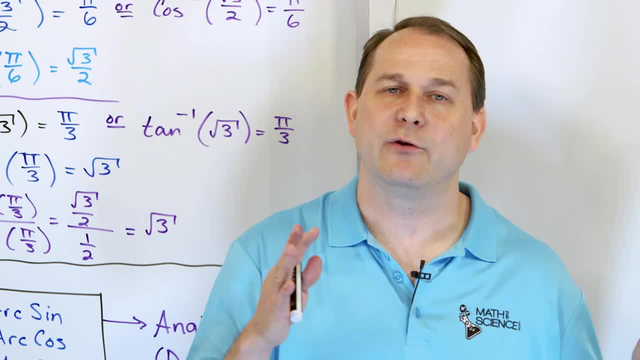 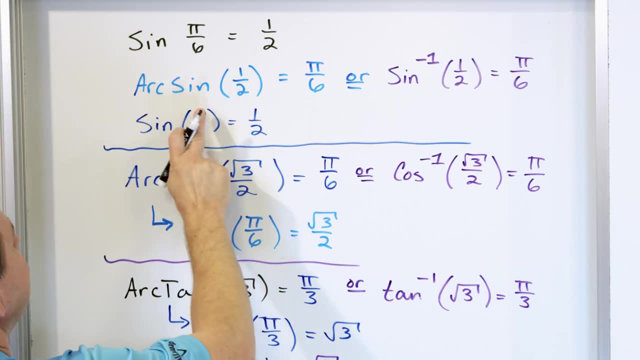 everybody to comprehend. Let's go back to our example. Sine of some angle is one half. We already did it. We said: sine of some angles one half means arc. sine of one half is 30 degrees or pi over six. Okay, So let's go back. 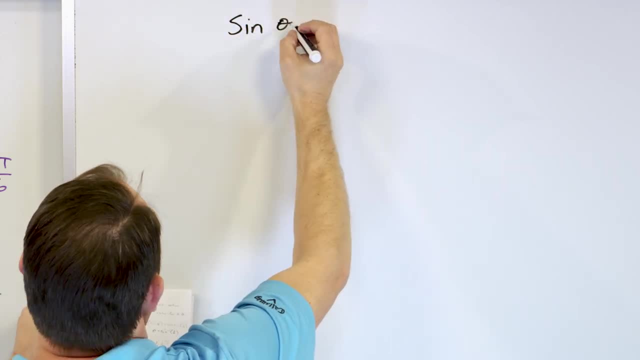 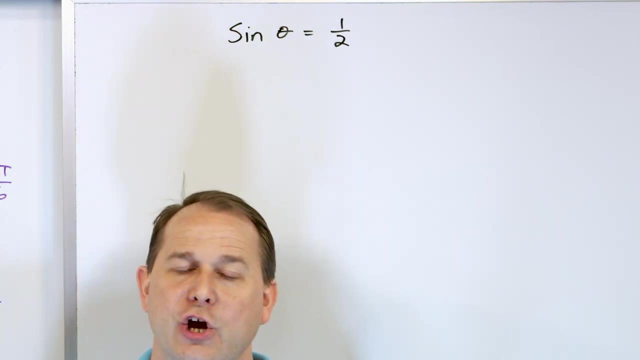 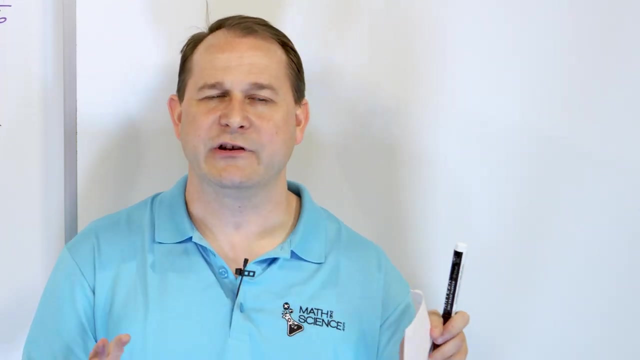 To sine of some angle is equal to one half. Now remember back from basic algebra. you have inverse functions, inverse operations to solve equations, right? So if you have an equation like three X equals six, you're multiplying on the left-hand side by three. So to get rid of it, 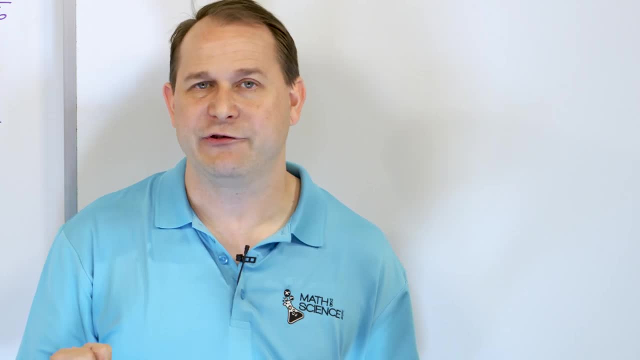 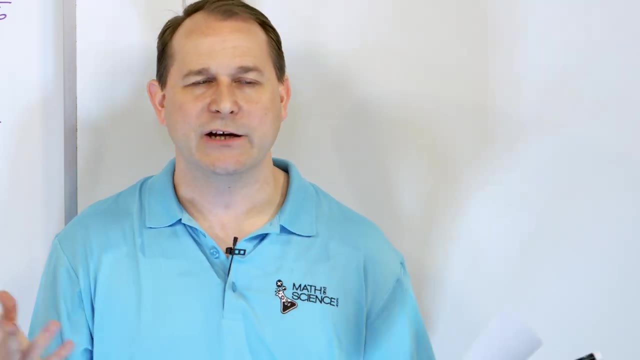 you do kind of the inverse operator and you divide. Opposite of multiplication is division. If you have a square root, you might undo the square root by squaring both sides, So it undoes the square root. I can go on and on. 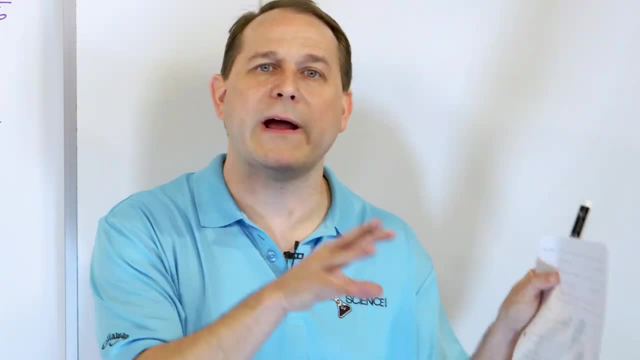 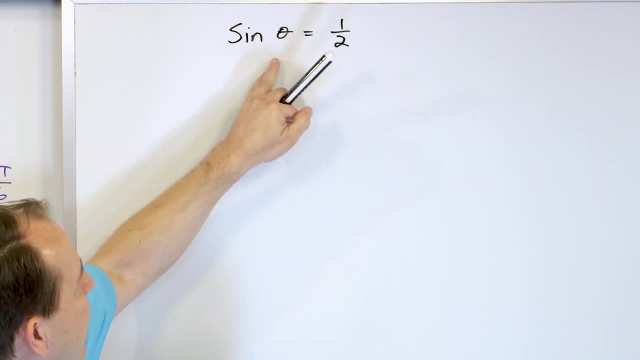 If you have a logarithm on one side, then to undo the logarithm you might raise both sides of the equation to a power of the base of the logarithm to undo the logarithm. So here's kind of a basic equation. I know it looks so simple because we know that sine of 30. 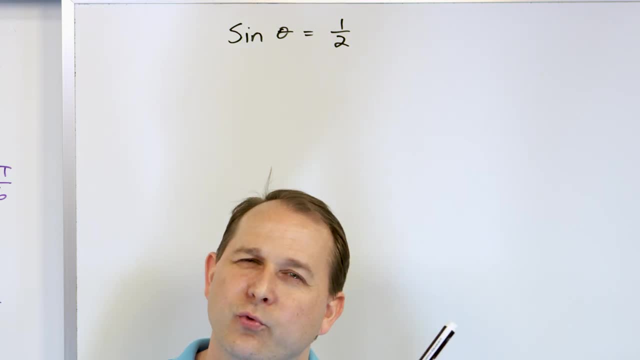 is one half, So we can solve this equation really easily. But really the real way that you solve this equation is you undo the sine function and try to solve for theta and get the function or the, the, the, the variable, theta by itself, and then you should have some kind of angle as a result. We already 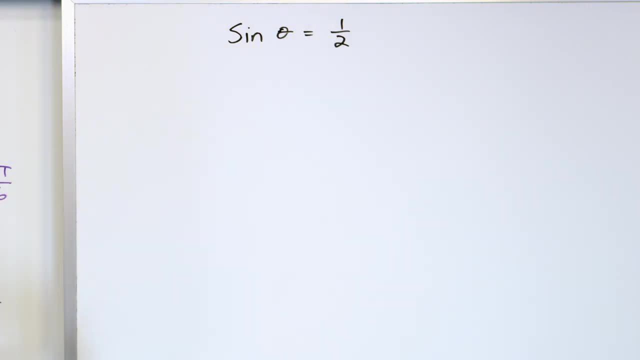 know the answer. The answer is 30 degrees or pi over 6.. But really the way that you solve it is you have to undo the sine operation. How do you undo a sine function? You do the inverse, the arc sine, to both sides of the equation. So to solve this simple equation, what we would do, 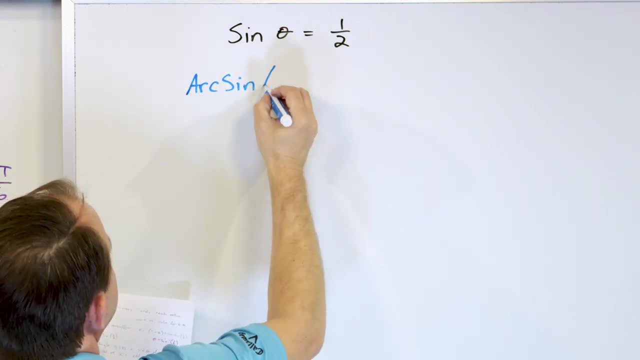 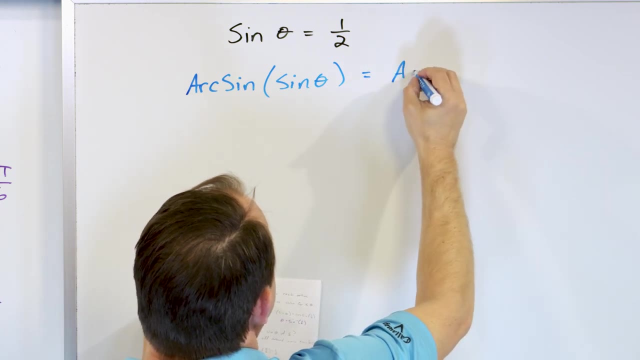 is, apply the arc sine to both sides of the equation. We apply it to the left, which means we're applying the arc sine to the sine guy And on the right. we have to do the same thing to both sides, just like we have to do the same thing to both sides of an equation all the time. 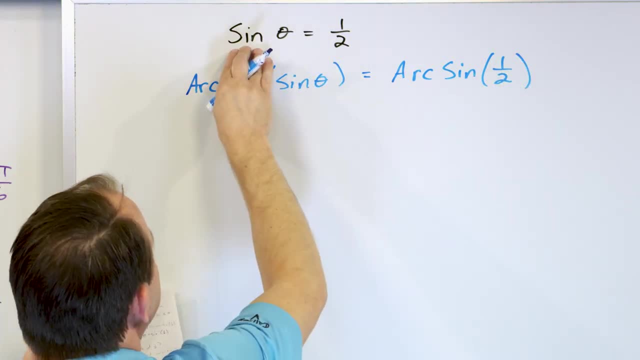 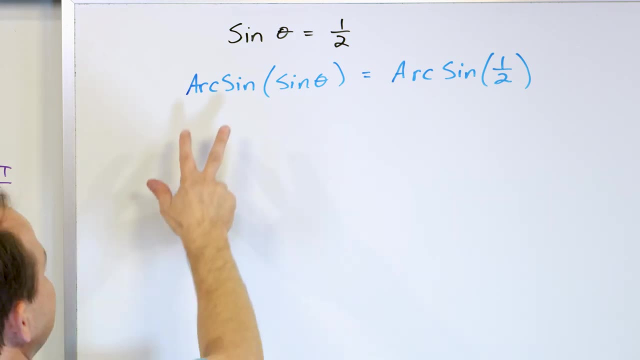 So to solve this equation? we already know the answer, But basically we can apply the opposite function to the left and then apply the opposite function to the right. All right, Now what ends up happening is the arc sine is the exact opposite of the sine, so it undoes the sine. 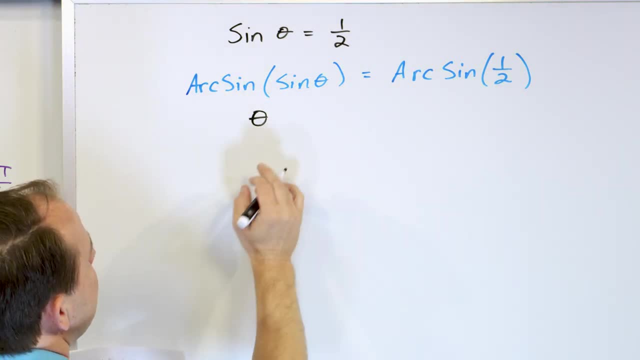 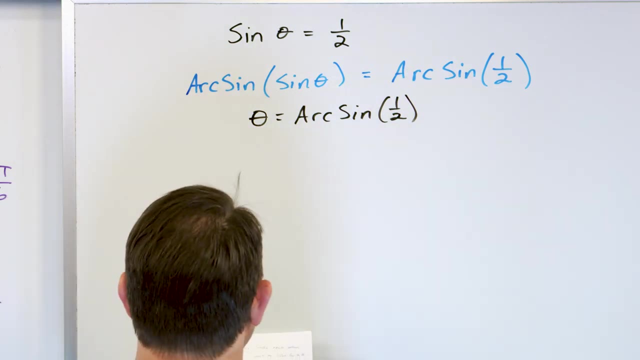 And so all you have left on the left is theta, And on the right you have arc sine, And we already talked about the fact that arc sine of 1 half means that it's a 30-degree angle. so then theta is 30 degrees, or pi over 6, which we've already talked about. So I'm introducing: 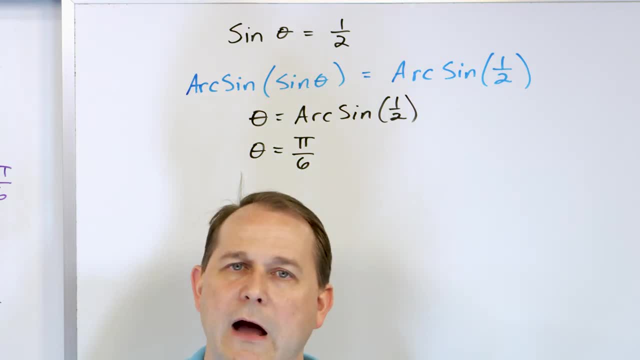 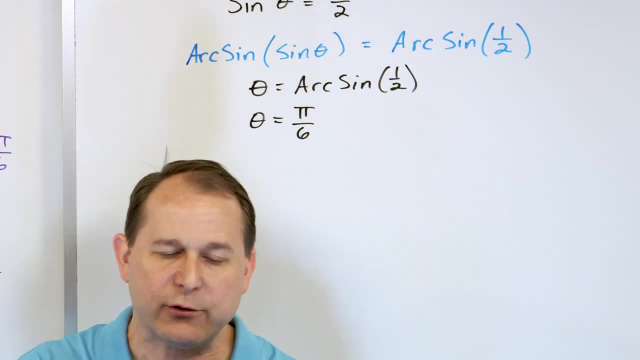 arc sine, arc cosine. but I want you to understand the big picture. We obviously want to go backwards so that we can solve lots of times and we want to figure out what the angle is, But also because later we're going to have trig equations, which are really big equations with trigonometric 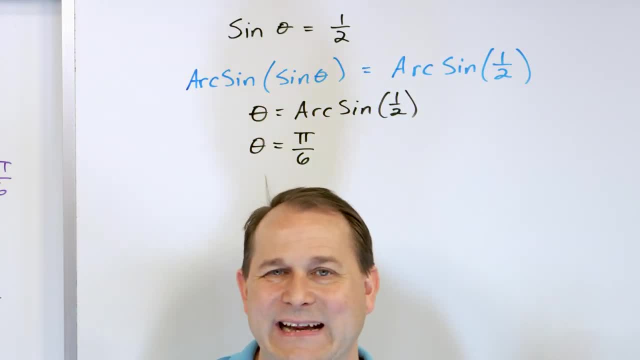 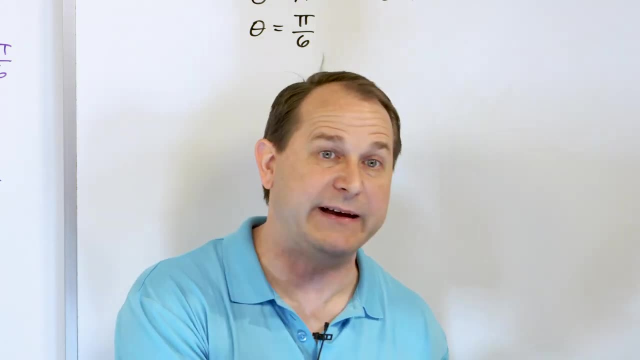 functions. The goal of them is always going to be to figure out what theta is. So you have to have a way to rip open that box and get the theta that's inside, And the way you do it is to basically annihilate the sine with its inverse, which is the. 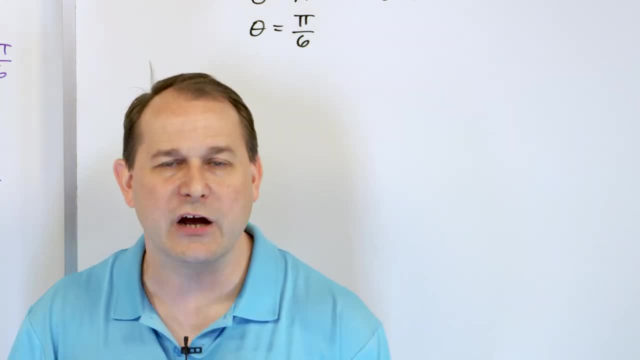 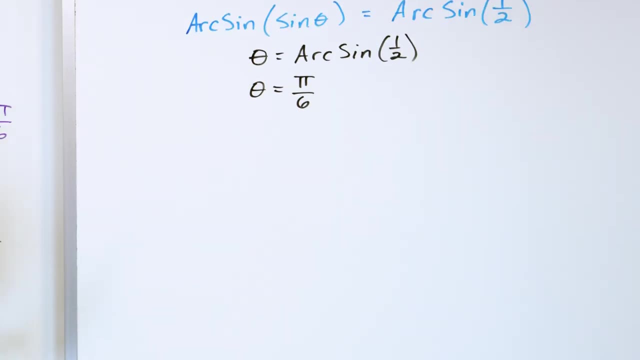 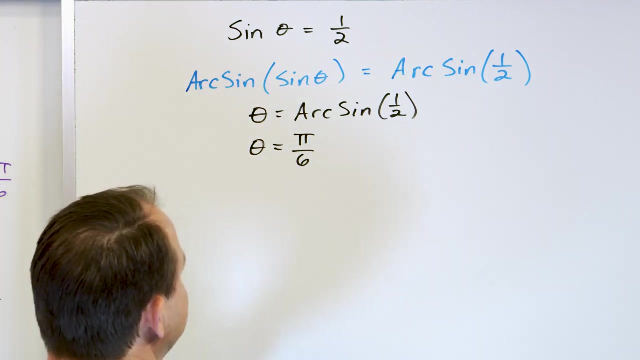 arc sine. To annihilate a cosine, you use an arc cosine function. To annihilate a tangent, you use an arc tangent And we're applying it to both sides like we solve all of these equations here. So we already said the angle here is pi over 6.. So let's draw this and talk about it a little bit. 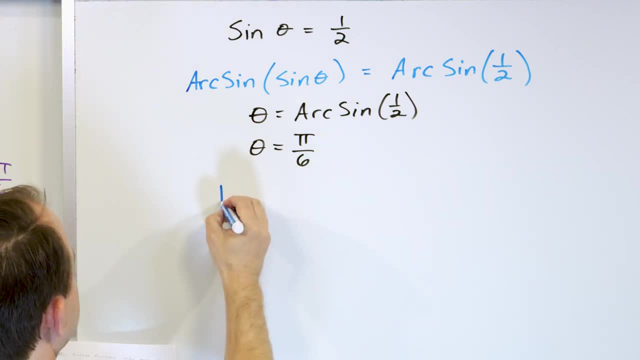 What we're basically saying is that we've got a unit circle that we have on the other board as well. I think I want to do it probably right over here. Let's draw this function right here or this unit circle right here. We'll do a little sketch and I'll also use the real unit circle we have over there. 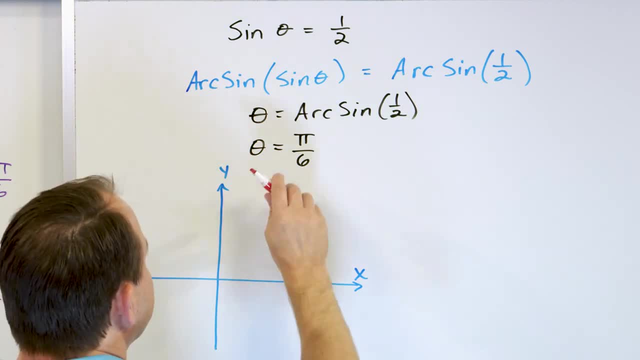 What we're essentially saying is that if we go to pi over 6 here, here is about, roughly speaking, a 30 degree angle. It's not perfect, but this is roughly a 30 degree angle, So I'll put theta: this is pi over 6, which is 30 degrees. 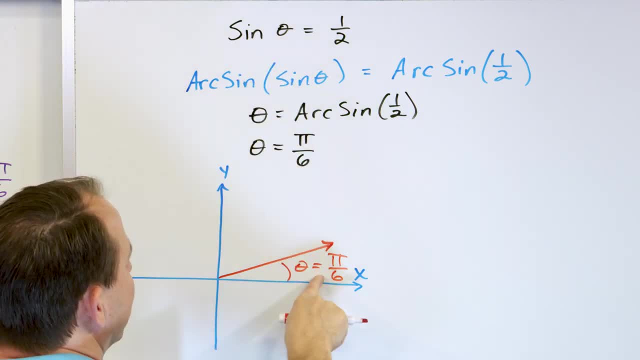 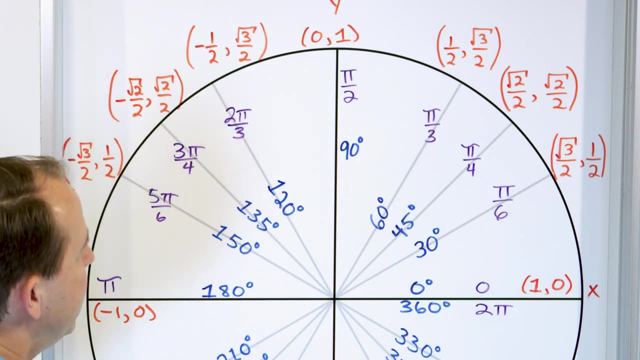 we're saying is that the sine of this angle of pi over six is one half, And that's why it is the solution of the equation. Let's go check it on the unit circle. Here's pi over six, which is 30 degrees. The cosine is the first number, The sine is the second number. So here we're saying the 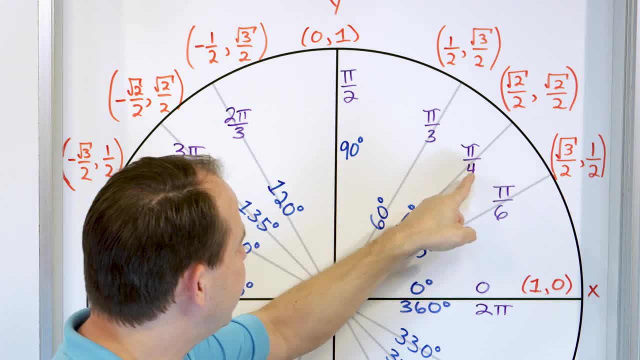 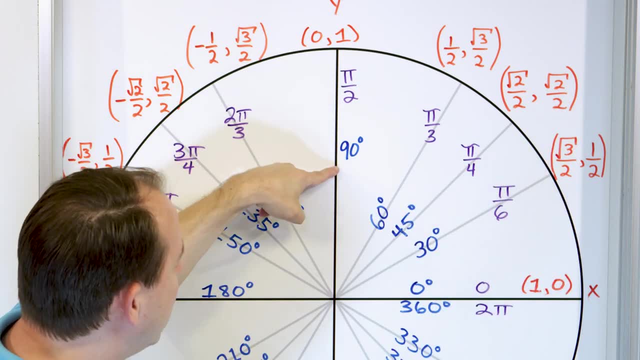 sine of 30 is one half. The sine of pi over six is one half, which means the projection here is right, because we're talking about the sine, The projections on the y-axis, which is exactly in the middle, which means it's at one half. exactly the case. But let me ask you this: Are there any? 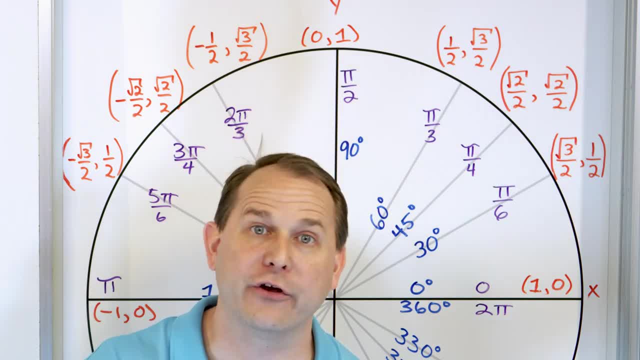 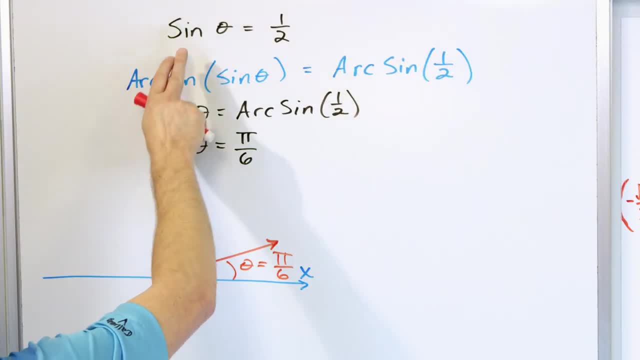 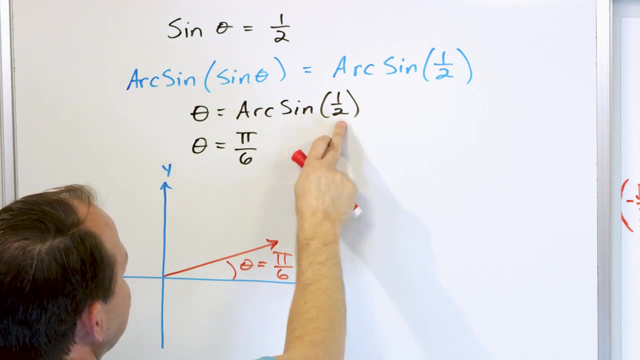 other angles around the unit circle that also have a sine that give you one half. I mean, think about what you're asking yourself. You're over here saying sine of some angle is one half. Give me the angles that work. And we figured out through doing all this arc, sine of one half. we're. 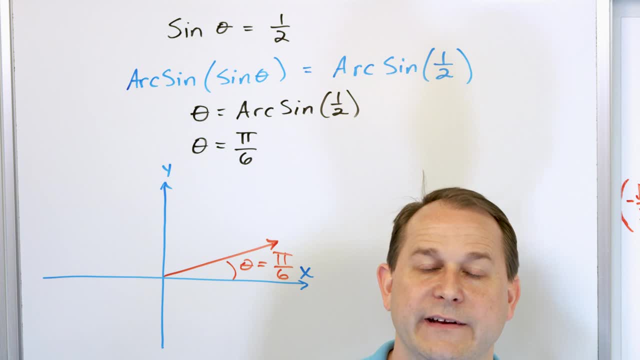 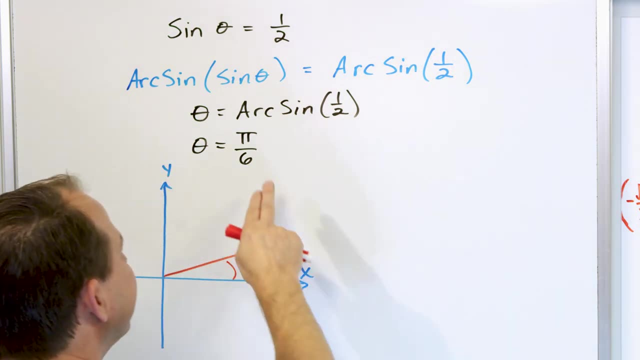 getting the angles right And we got an angle Pi over six. we said, hey, it works, It's the angle, It's the answer. But it turns out there's tons of other answers, There's tons of other angles that work. Because, in order to solve this, 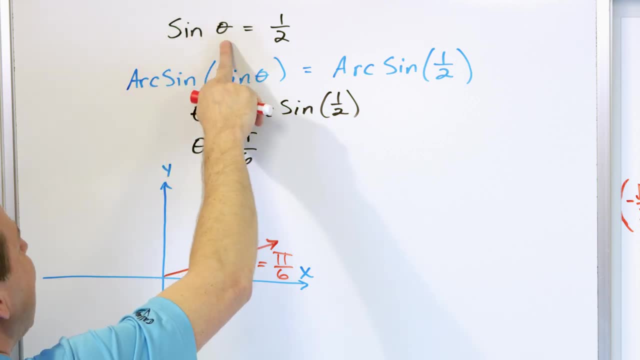 all you need to do is figure out the angles such that the sine of the angle is one half. Here's one of those angles. But walk with me over here and look at this. If this is pi over six, then right here would be two. pi over six, Then here would be three. pi over six, Then here would 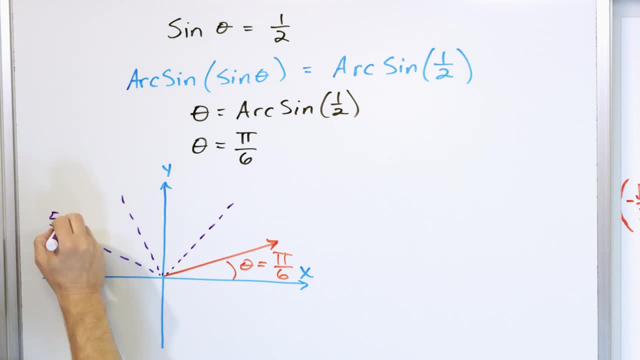 be four pi over six, Then here would be five pi over six. What is the sine of this angle? Five pi over six. It projects onto the y-axis. It projects onto the y-axis. It projects onto the y-axis at exactly the same location. here It's going to be positive one half. So what we have? 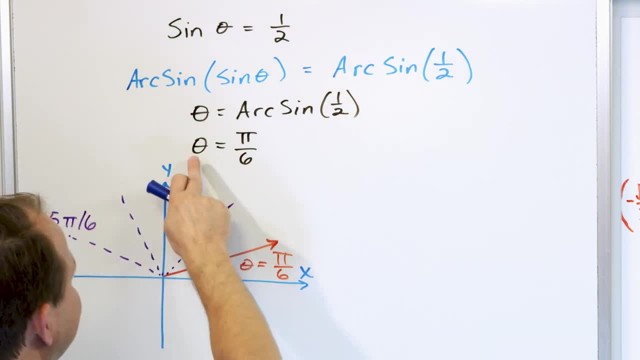 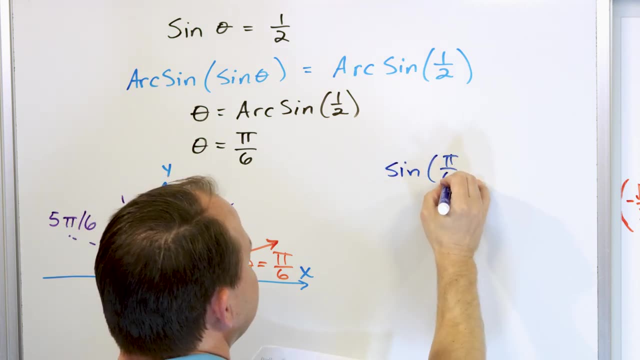 figured out is that there's actually multiple answers to this. Pi over six is not the only answer, But let's just go through it. So the sine of pi over six is indeed one half, So it does satisfy this equation. However, the sine of five, pi over six is actually also equal to one half. So 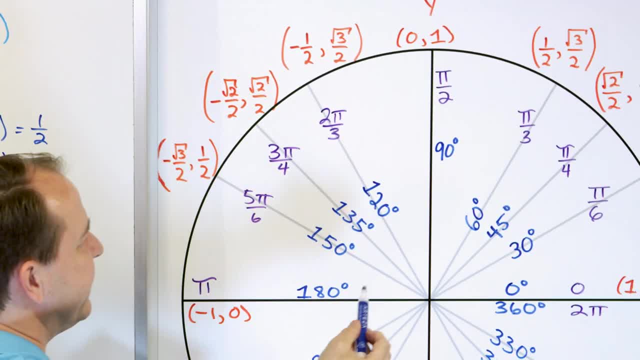 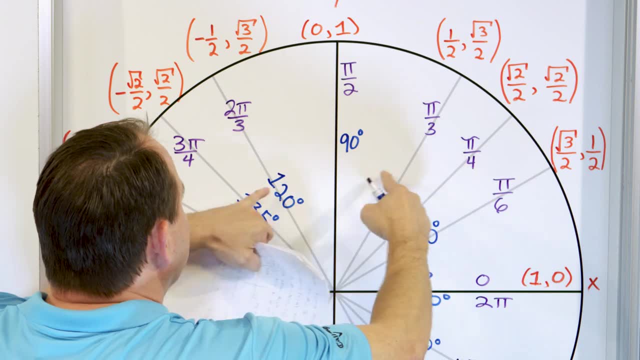 it looks like there's another answer that lives over here. If you go back to the unit circle, the sine of this is one half. But look at this: The sine of this angle is also one half, because both of these angles project onto the exact same location. But wait, there's more, There's possible. 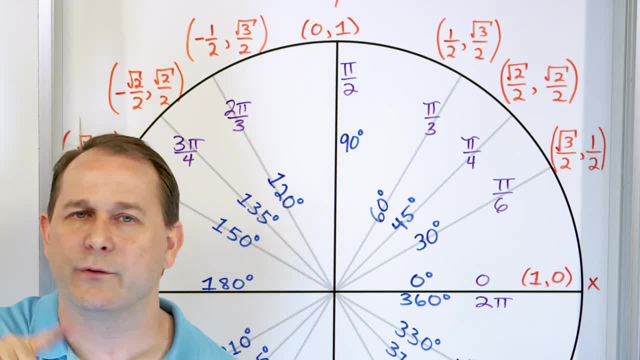 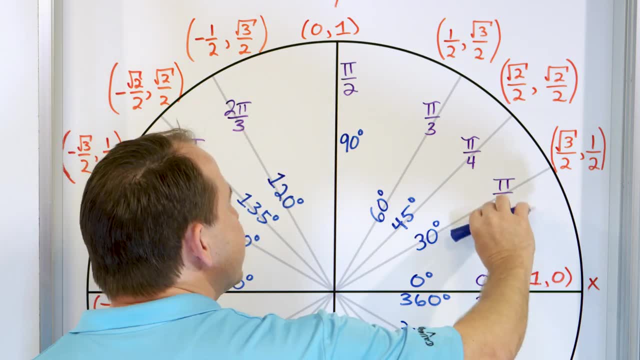 to have more angles. In fact, there's an infinity number of angles that will give you that same sine of one half. What happens if I go all the way around the unit circle and continue counting until I get here? What's going to happen there? Let's just take a look. You have pi over six. 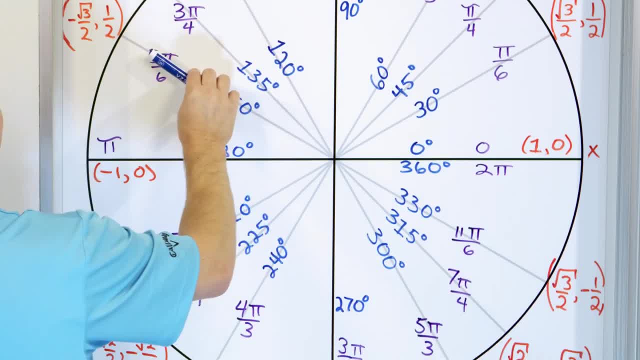 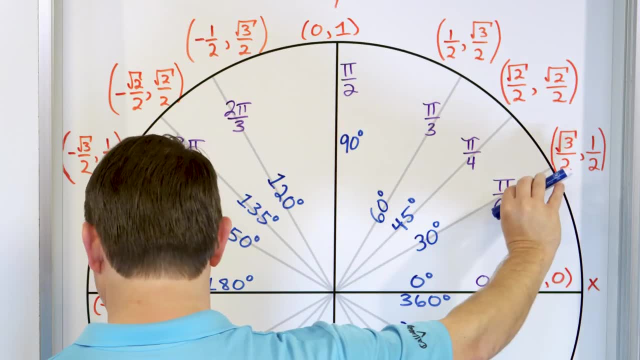 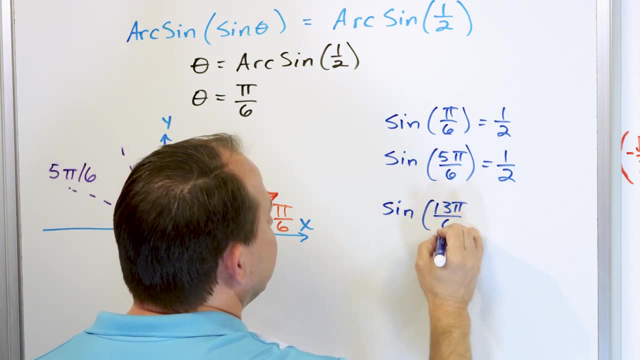 two pi over six, three Then four, then five pi over six, then six, then seven, then eight, then nine, then 10,, then 11,, then 12.. 13 pi over six is right here, 13 pi over six. So we can say that sine of 13 pi over six is also. 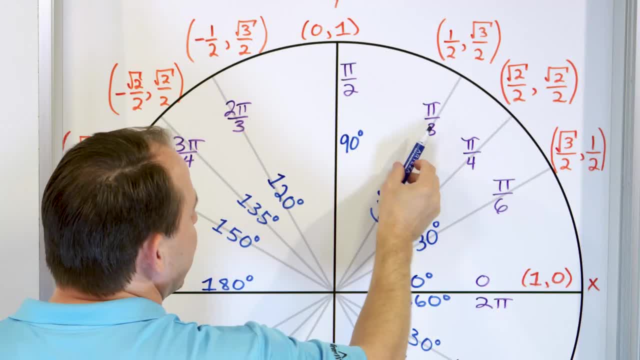 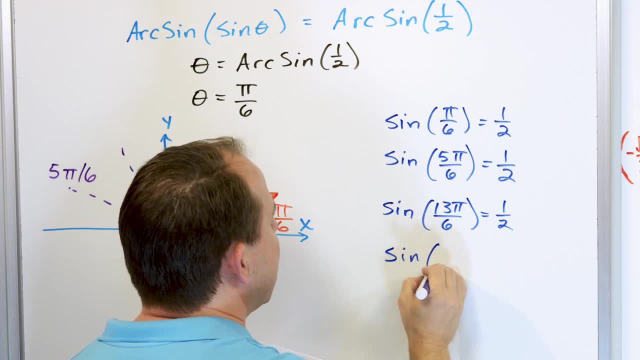 equal to one half. So this is 13 pi over six. Here's 14,, 15,, 16.. Here's 17 pi over six. It gives you the same projection here. So we also know that sine of 17 pi over six is equal to one. 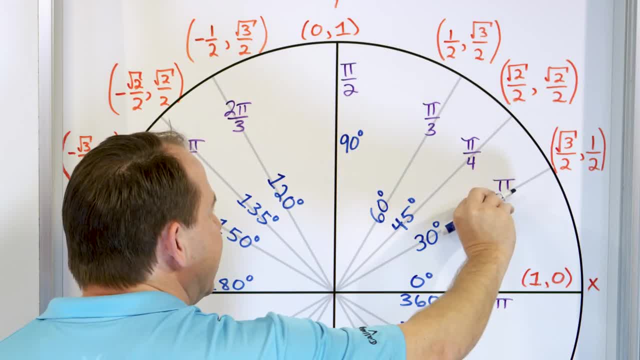 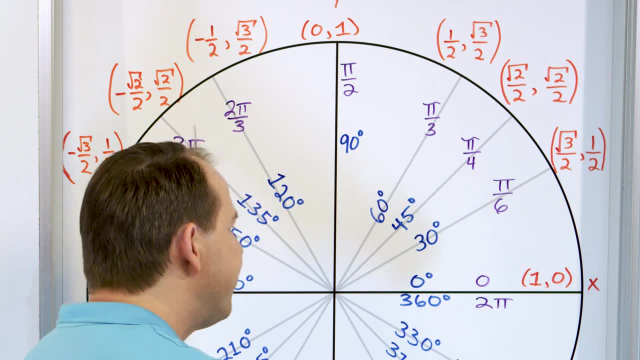 half. You see, I can play this game again and again Any time I land here. any time I land here, I'm going to get the sine of these angles. Both of them are going to give me one half. If I land on angles down here, all of these angles are going to project. 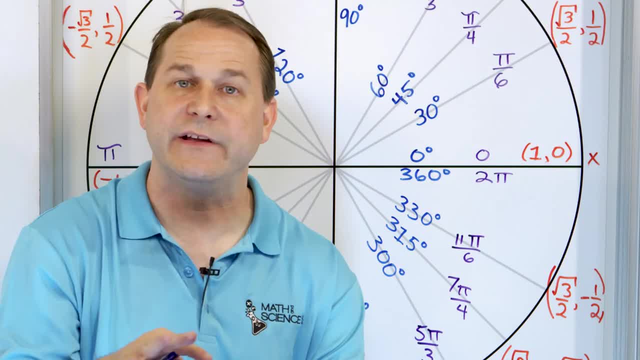 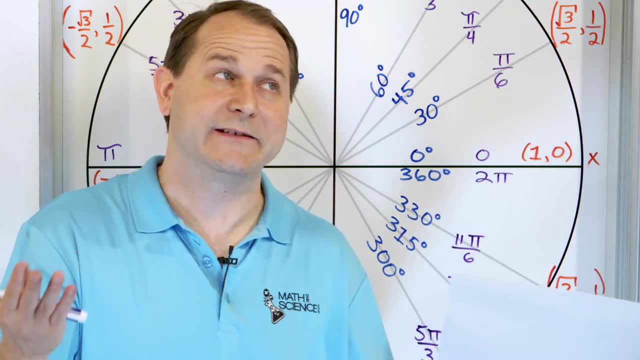 to negative one half. So the sine of those angles down there don't work. Only the angles in the upper half plane give me the same exact sine. with the same exact sine, the positive one half. Also, notice you can go in the negative direction. 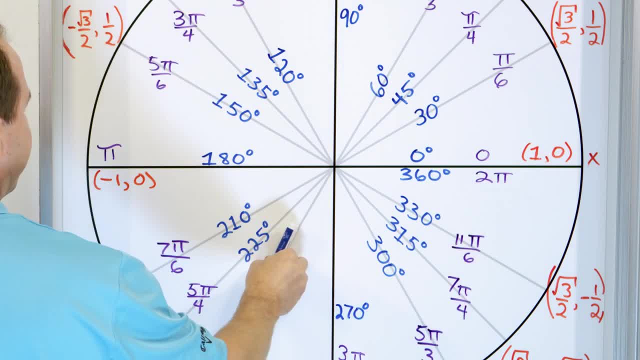 negative pi over 6, negative 2 pi over 6, negative 3 pi over 6, negative 4 pi over 6, negative 5 pi over 6, negative 6 pi over 6, negative 7 pi over 6 is right here. Negative: 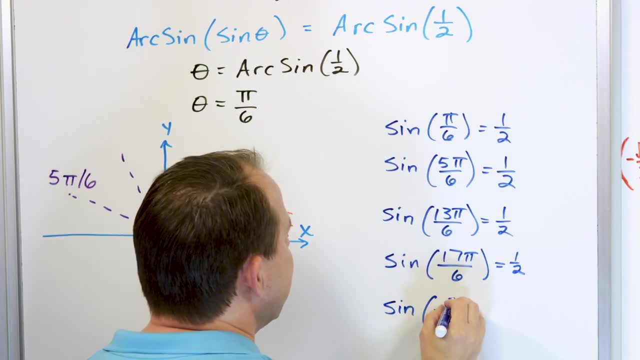 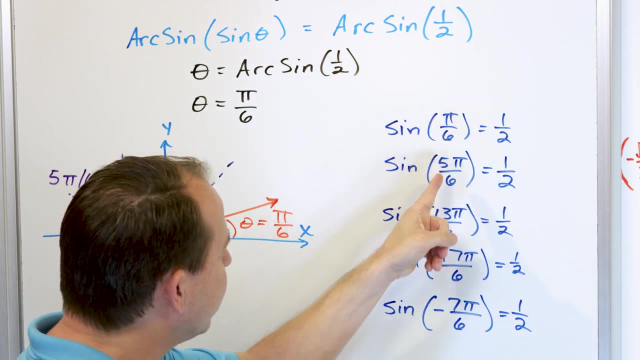 7 pi over 6 is the same location. So the sine of negative 7 pi over 6 is also equal to one half. I encourage you to get a calculator or a computer and put all these angles in there and then hit the sine button. It's going to give you the same thing- one half. And that's because it's a unit. 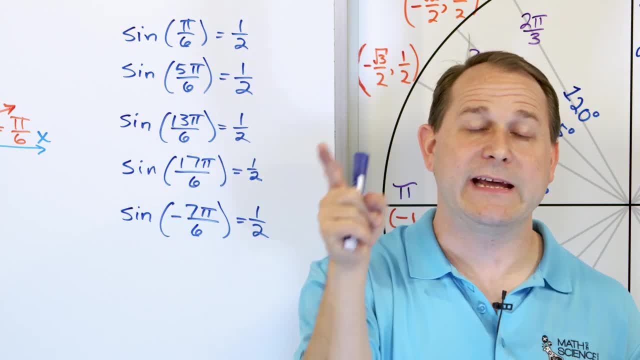 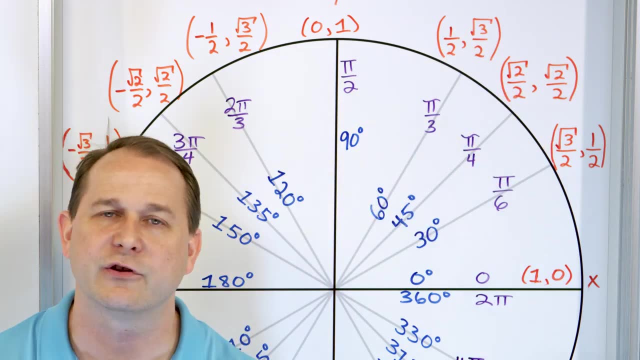 circle, and I can keep counting over and over again. Not only can I keep going in circles to land on the same place, but there's actually two different kind of fundamental angles that also give me the same sine. So the question is, whenever I take the arc sine of one half, which is what I'm 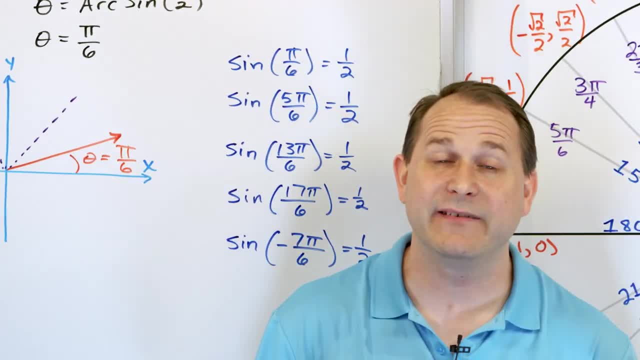 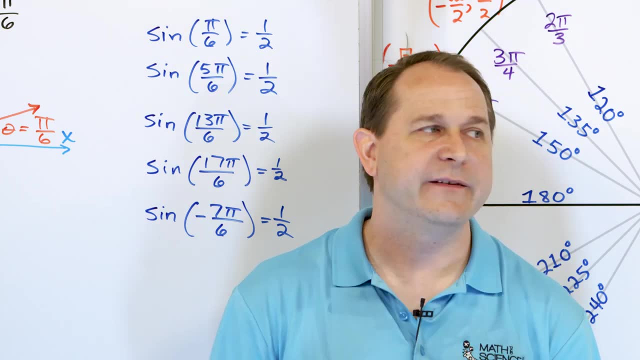 doing to solve this equation? what angle should I get back? It seems like they're an infinity number of angles. They're an infinity number of angles. What angle should the calculator return? And this is where we come back to what we talked about in the beginning. 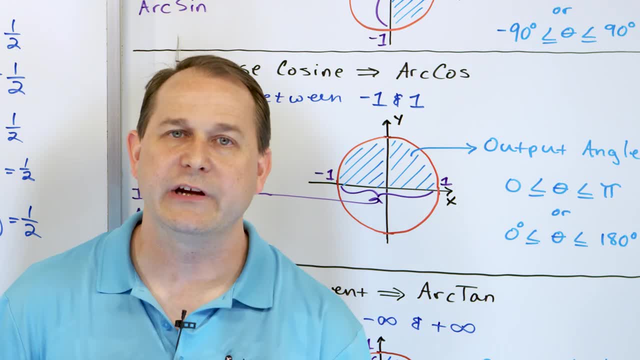 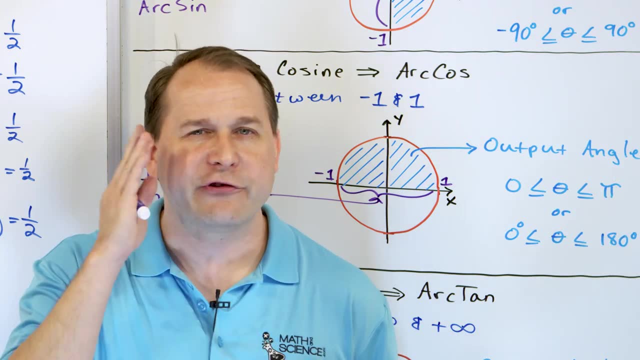 That there's only a certain range of angles that the calculator will return. So I need to walk through why. But in the back of your mind, before we jump into all this stuff that we have to talk about, just remember: when I take the arc sine of anything, I can get an infinite number of angles. 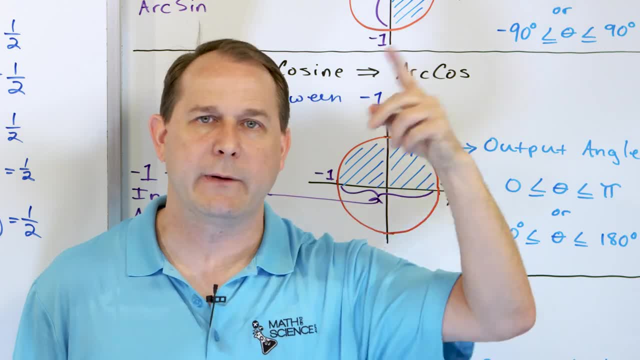 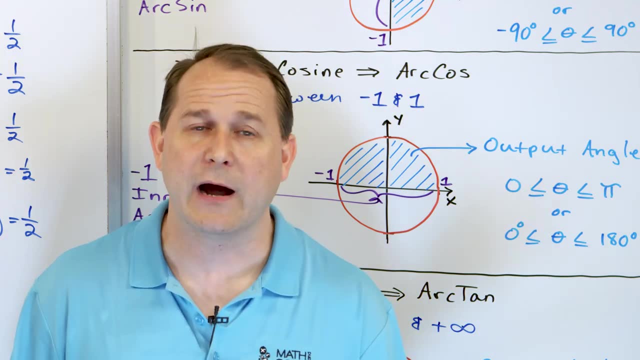 because all I have to do is figure out the fundamental ones And then I can keep spinning around the unit circle finding an infinite number of additional angles for any arc sine or any arc cosine or any arc tangent of any number. I can find tons of angles that all work. 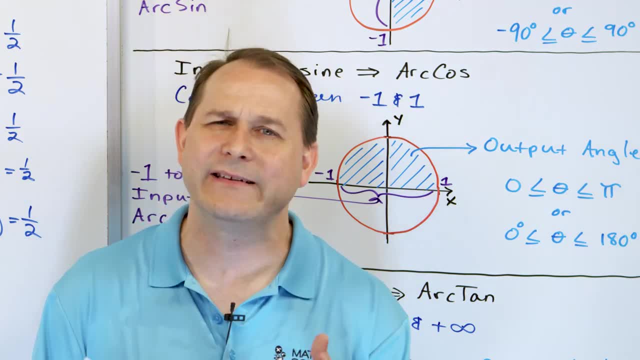 So the calculator is not going to give me the same thing. I'm going to have to find the infinite number of angles that all work. So the calculator is going to have to find the infinite number of angles. So let's first talk about what is the inverse sine of an angle, And it's not going to give you an infinite. 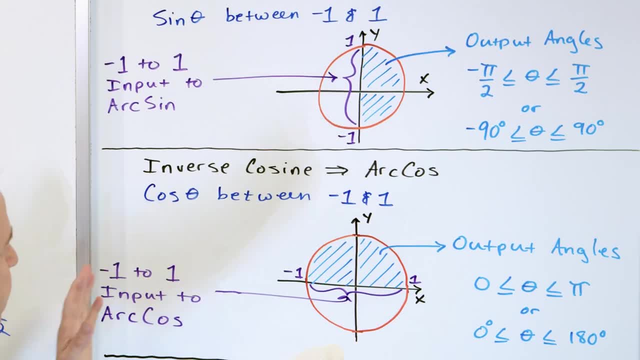 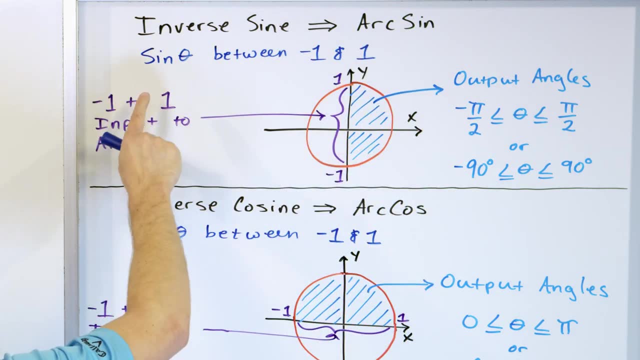 number of answers. So how does it know what to give you? This is what we have decided by convention in math, the way it's going to work. Let's first talk about only the inverse sine. It's called the inverse sine. It's important for you to know that the sine of an angle always lies between negative. 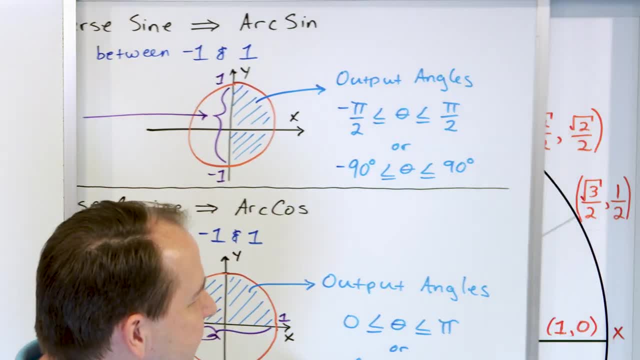 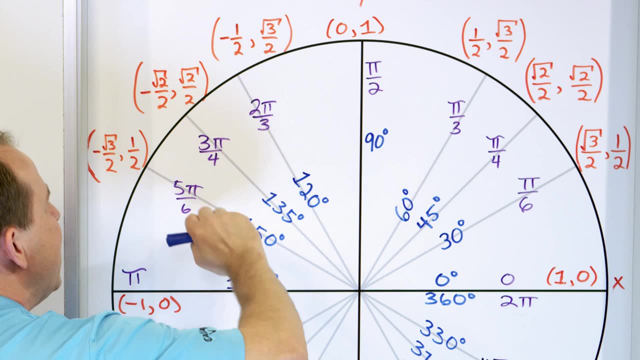 one and one Always. How do you know? Because it's a unit circle. The circle only has a radius of one, So if I take the sine of any number around here, it can only give me a maximum of one. That's one. 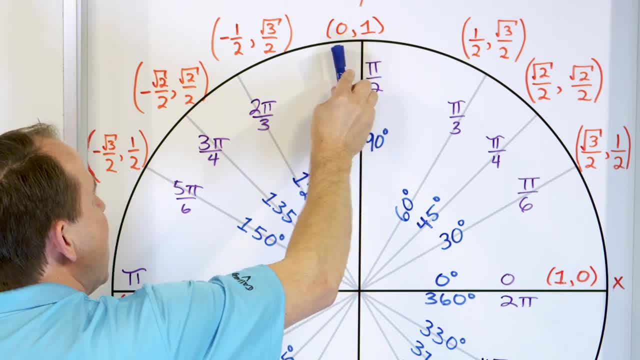 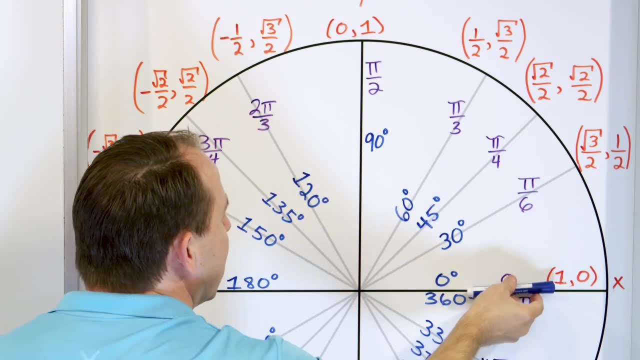 up here. the sine up here would be one positive one. any angle over here will just be a fraction of that. projecting onto this axis, it'll be a fraction of that. the sine over here is zero. the sine over here is also zero. the sine over here is positive one and the sine down here is. 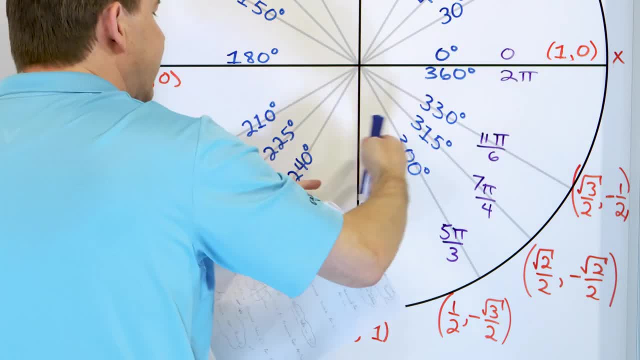 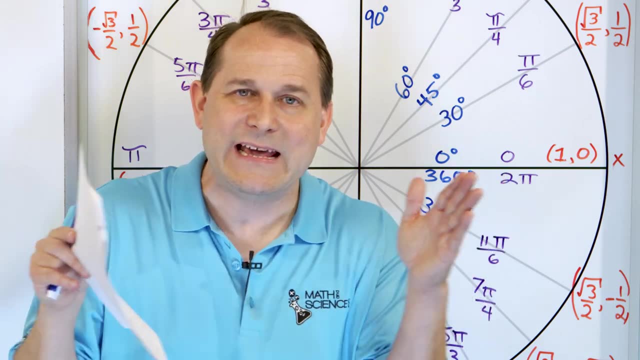 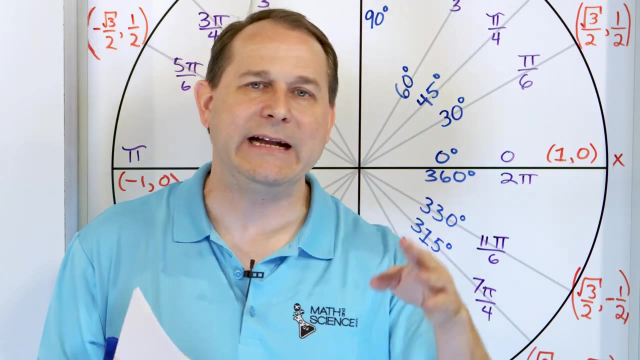 negative one. any angle down here is going to be projected here, it'll be less than well larger than negative one, basically anywhere between plus one and minus one in that range, larger than negative one and smaller than positive one. it's impossible to get a sine go type in any angle. you. 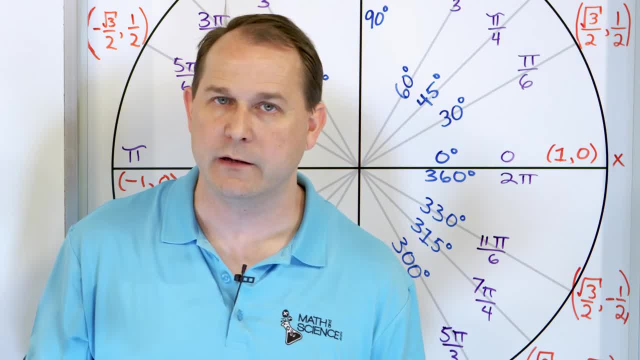 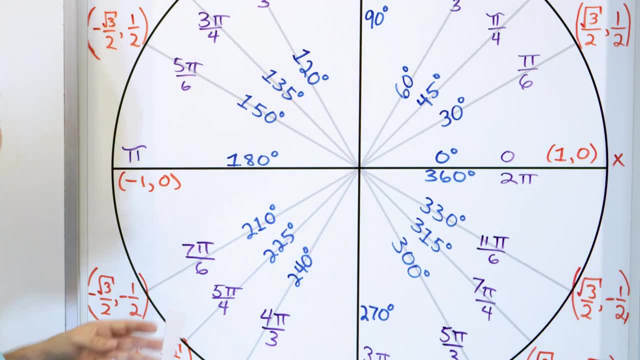 want in your calculator, hit the sine button. you will never get a number larger than one or smaller than negative one, like you'll never get negative two or negative three or negative four, because it doesn't work like that the way the projections work. okay. so it's important for you to know. 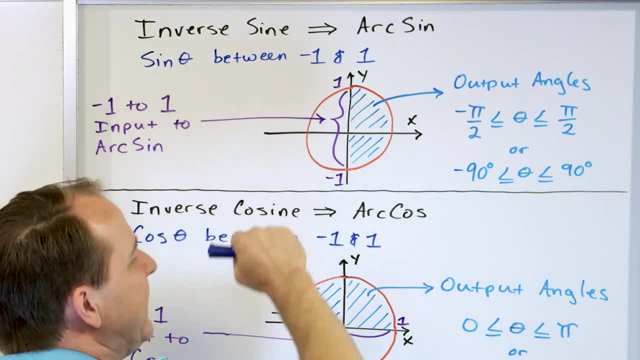 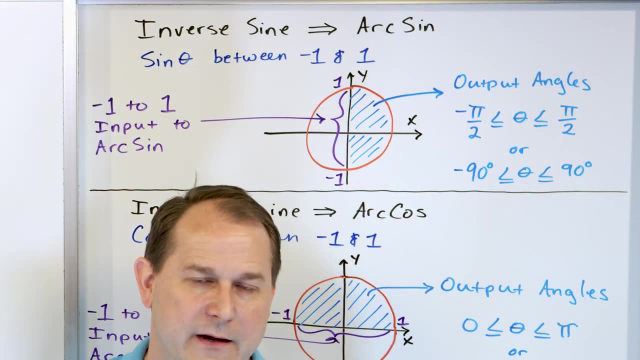 that the input, that the sine function can only spit out numbers between plus or minus one. that means that the arc sine, which is the opposite of the sine function, can only spit out numbers between plus or minus one. the opposite inverse, the opposite function of the sine can only take as inputs to the bit: 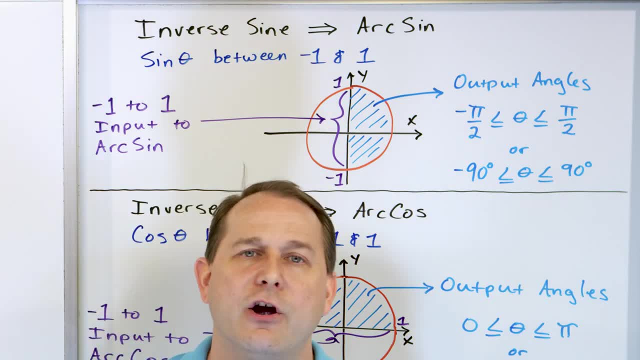 numbers between negative one to positive one. why? because the arc sine is going backwards. i'm feeding numbers in from the outside of the unit circle and i'm getting angles back. so because the sine can only give numbers between plus and minus one. then feeding numbers into the arc sine, remember, 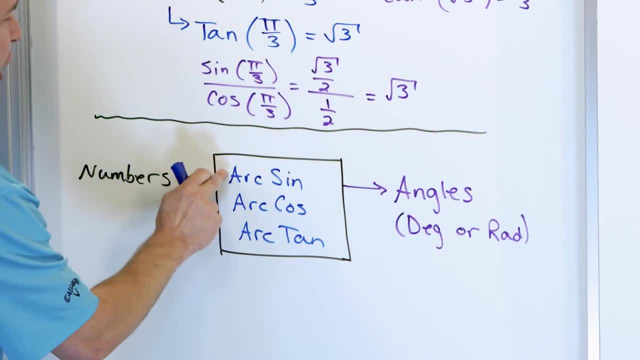 this picture i drew for you, feeding numbers into the arc sine can only be between plus or minus one, because those are the angles that the sine can only give to the arc sine and the arc sine can only be between plus or minus one. those are the only values that the sine function can give out. those 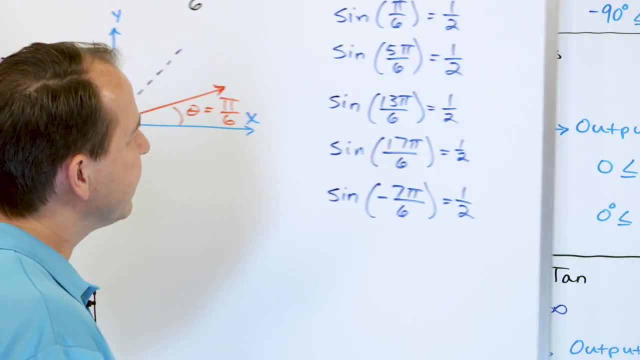 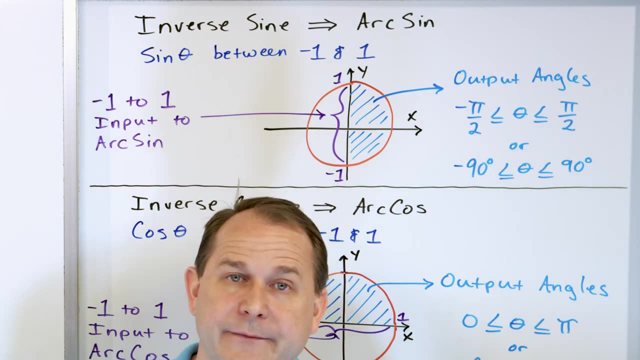 are the only numbers on the outside of the unit circle. so because of that the only numbers that can go into this arc sine are actually between plus or minus one. if you go press, let's say, five, that's way outside that range- and hit arc sine, you'll get an error. it won't do it because there. 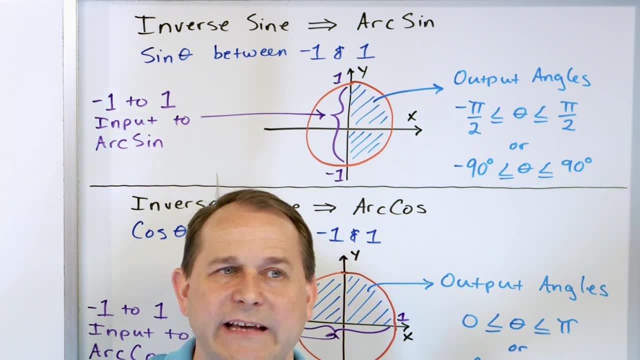 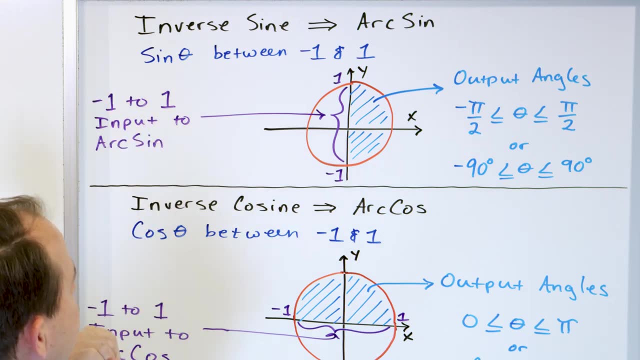 is no angle that has a sign that gives you a five or something, because sine can only go between plus or minus one. So the point is the inputs to the arc sign can only be between plus or minus one. But what I'm trying to show here is the sign is a projection on the y-axis, So the numbers between 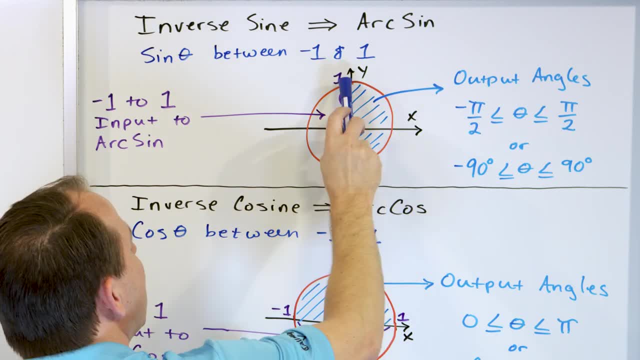 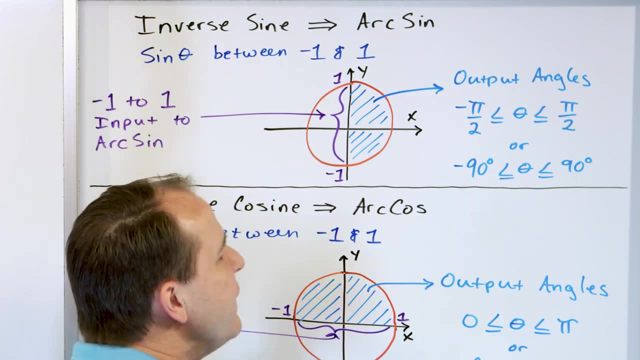 negative one on the y-axis down here and positive one on the y-axis here. any number that I give into this function is only going to be on this part of the y-axis between here and here. So the fundamental angle, the basic angle that is returned from a calculator, is going to be the smallest. 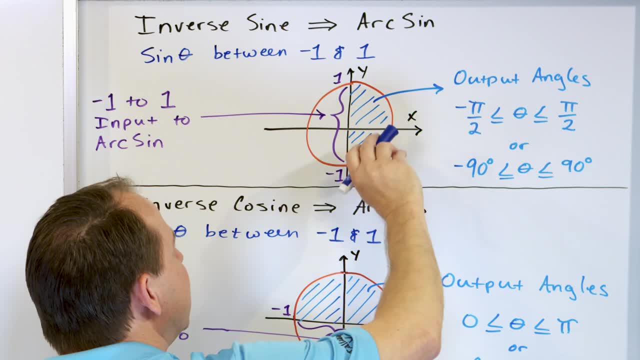 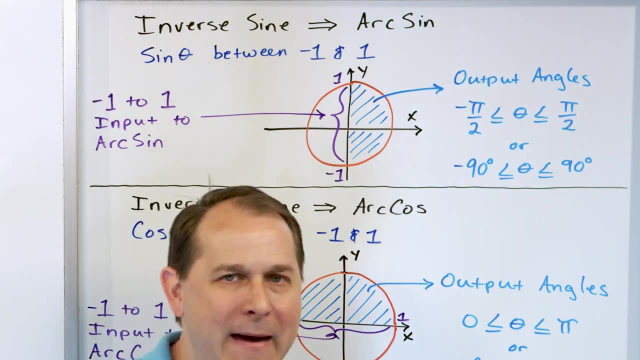 angles that have that as a sign, And so the smallest angles would be from zero up to pi over two and from zero down to negative pi over two. That is, by mathematical definition. those are the only angles that are going to come back, and that's going to cover all possibilities. 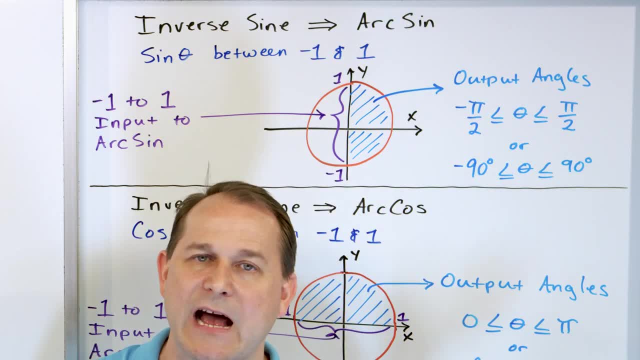 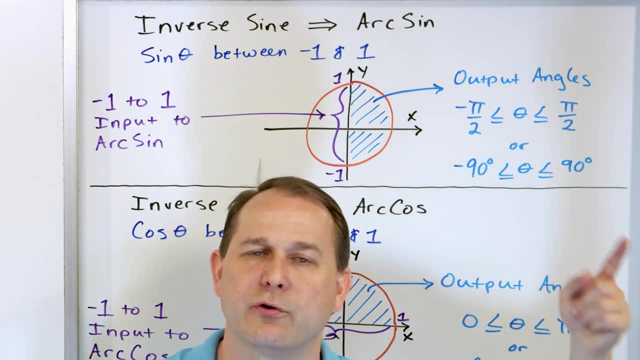 Well, there are still other angles around the unit circle that will give you that sign. but what I'm saying is the calculator is only going to give you the fundamental angle back. We all know that we can spin around the unit circle and get additional angles that have the same sign. but 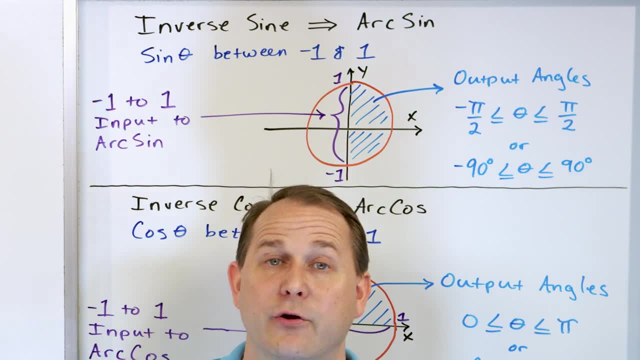 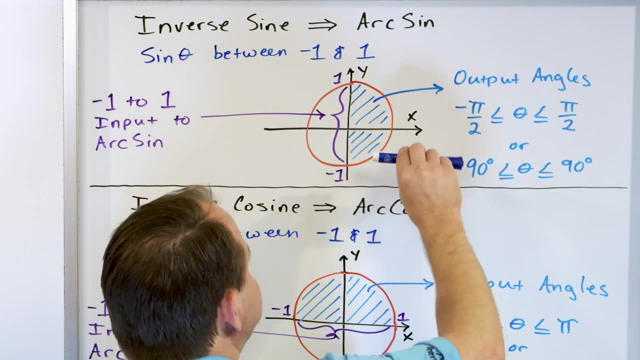 as far as what is that fundamental angle that the calculator will give you back, or the computer, or, by definition, what the function is able to give you back is always going to be in this range, Because, if you think about it, the sine of- let's take some angles here- the sine of pi over two is: 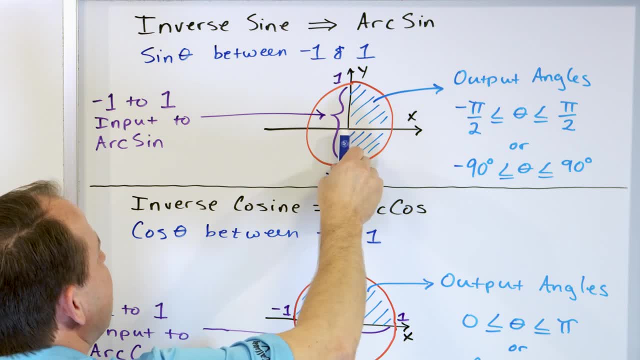 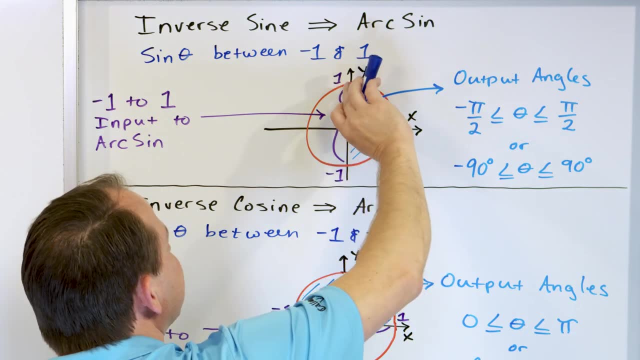 going to give you one, and the sine of negative pi over two is going to give you negative one and the sine of zero is going to give you zero. So any angle that I pick in this shaded blue region is going to give me a sine up here at one, or a sine at negative one, and the sine only goes. 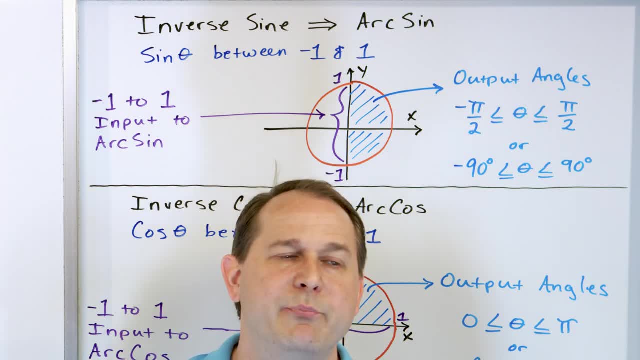 from negative one to positive one. So by convention, when I put negative one, positive one in the calculator, it's not going to give me an infinity of angles back, It's going to give me the smallest angle possible that satisfies the thing. So when we go back over here and we said, hey, 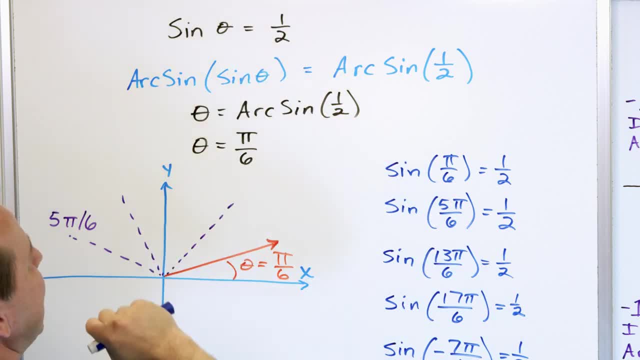 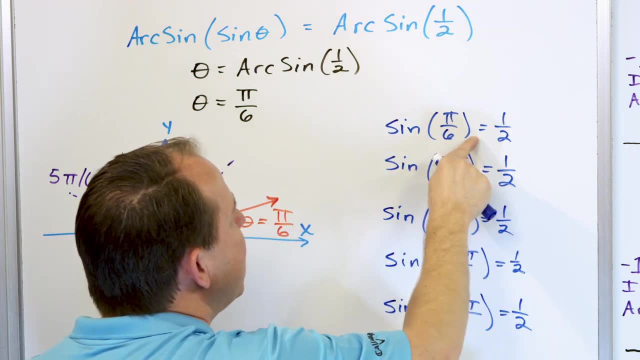 we're trying to find what angle gives me. so the sine is one half. it is true there's an infinite number of angles, but there's only one fundamental angle and that's going to be an angle, this first one. It's going to be between negative pi over two and pi over two. So when you hit the inverse sine, 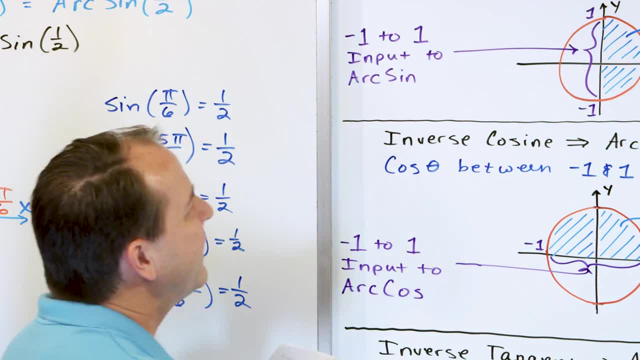 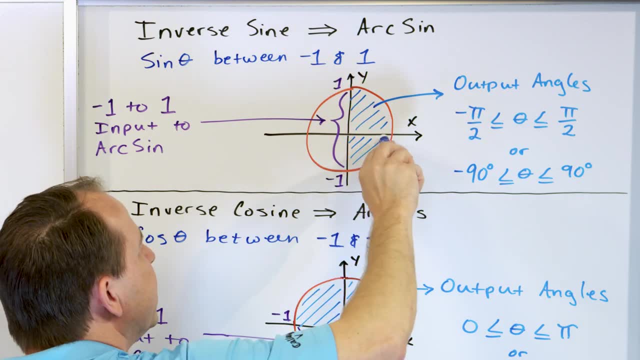 the angle you're going to get back. You're never going to get five pi over six because five pi over six is over here. One, two, three, four, five pi over six. it's outside the range over here. You're only going to get that fundamental back angle back. So that's the sine function. Let's 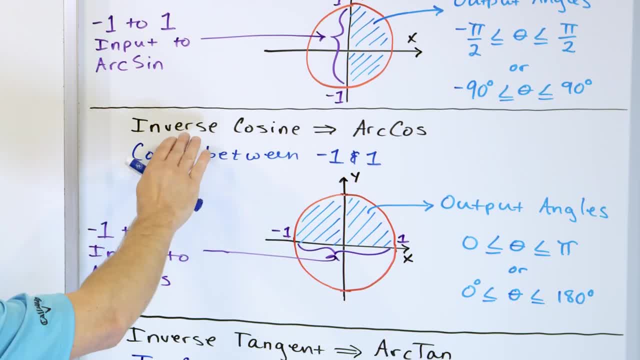 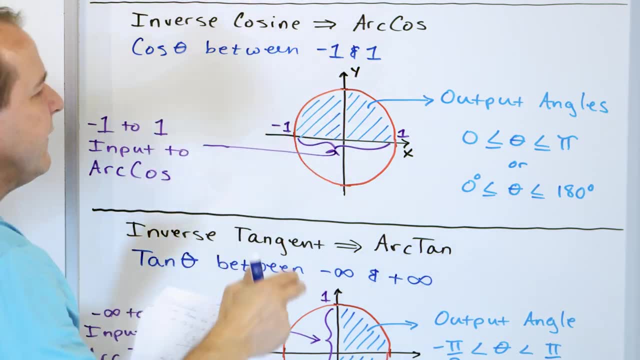 go have a similar discussion for the cosine function. The cosine function is an inverse cosine called arc cosine. It also can only give you values. the cosine function can only give you values between negative one and one. for the same exact reason, Any angle I pick. 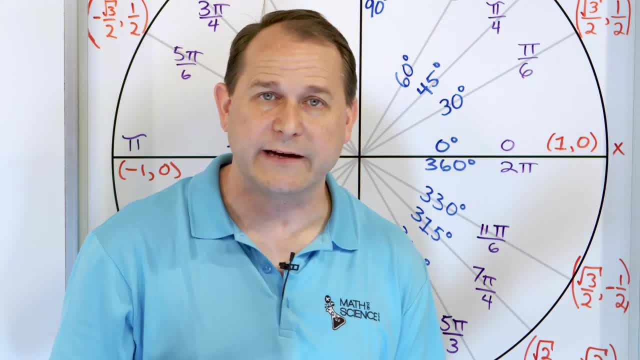 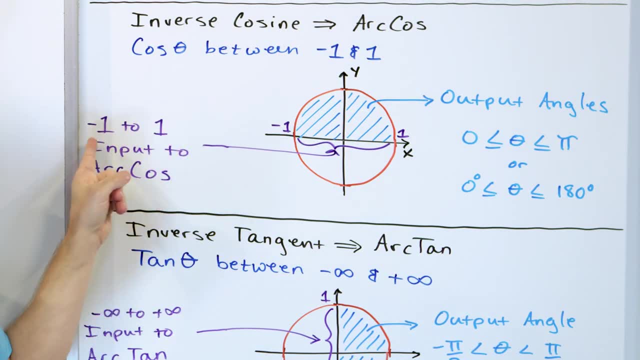 it's going to project onto the X axis, which can only go between negative one and positive one. So because of that the arc cosine, the opposite function, can only take as input values between negative one and positive one inputs to the arc cosine function, But those negative one. 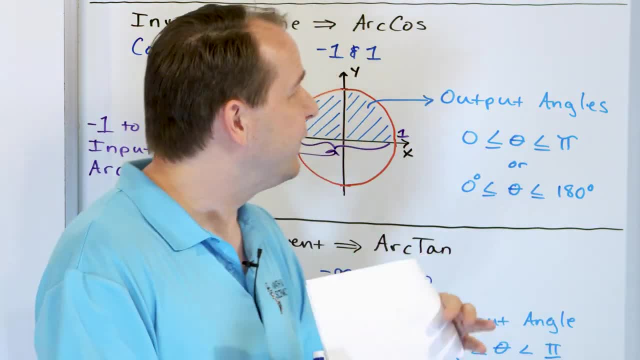 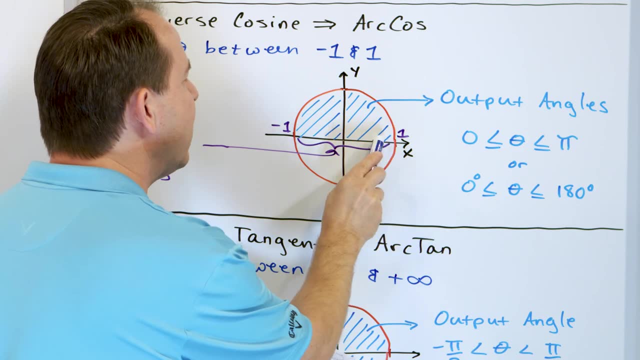 the positive one. those are projections on the X axis. Before it was projections on the Y axis, but for cosine is projections on the X axis. So those go from negative one all the way to positive one along the X axis. So these are. 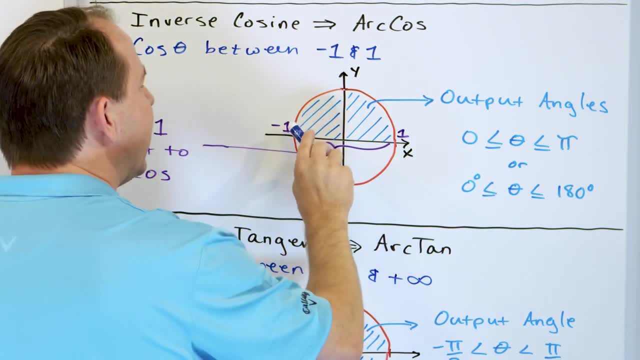 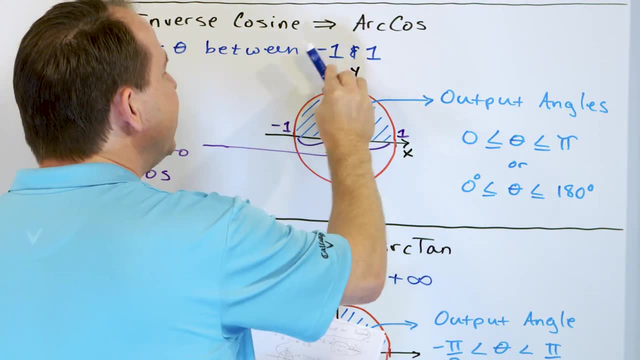 the inverse cosine. It's an inverse cosine. It's an inverse cosine. So we're looking at what you're inputs to the function. The output angles then are going to be the smallest angles that give me that projection, And the smallest angles there is going to go from zero to pi. right These down. 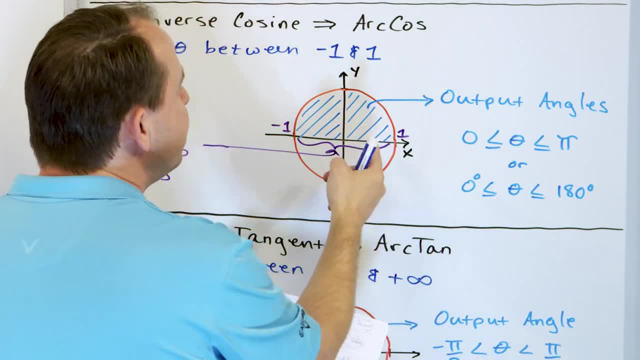 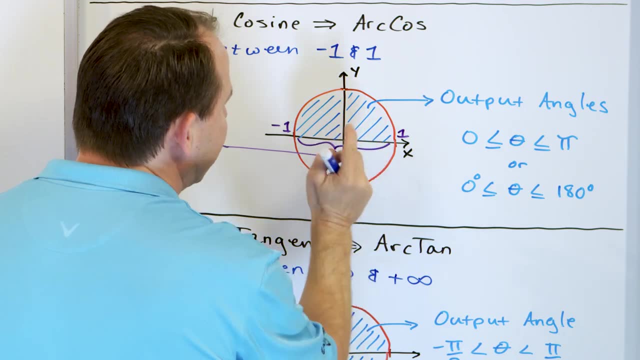 here. these angles aren't going to ever give you a return of value because, well, you see down here, any angle down here would project to the same axis as this angle projecting down here. So you have to have unique angles. I mean, think about it If you sweep angles through here. 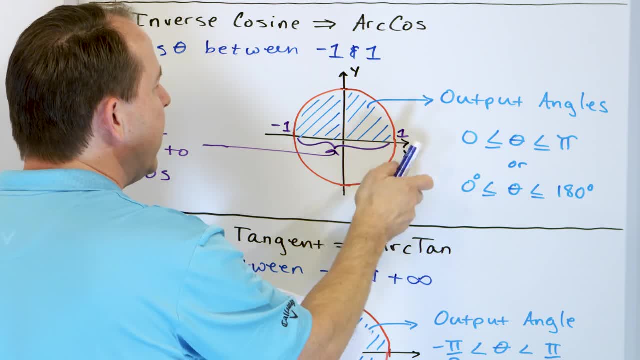 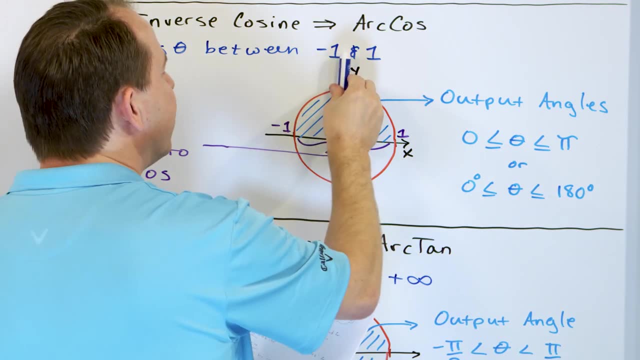 what's the cosine of zero? It's going to be a one. What's a cosine of pi? It's going to give you negative one, right. What's the cosine of pi over two Zero? So you see, I've already said that. 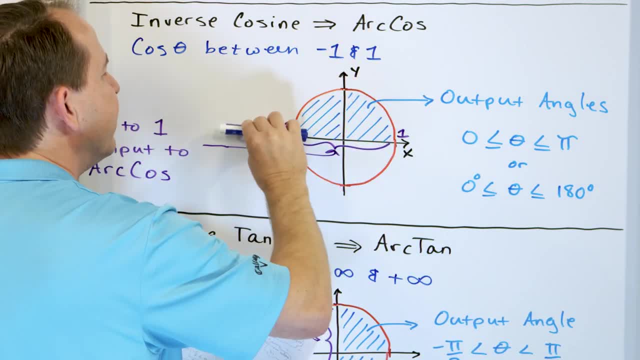 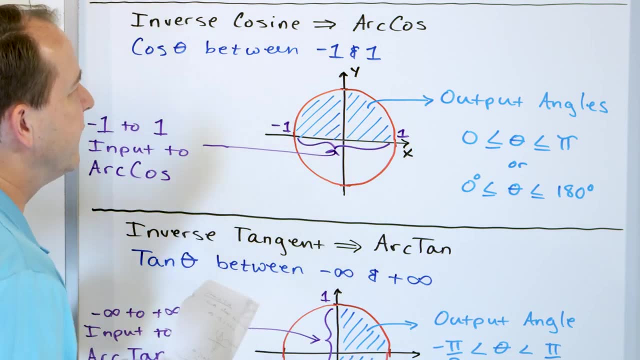 the cosine can only go between negative one and one. So all of the angles required to do that are up in the top here, because the cosine of any of these angles here are going to go between negative one and positive one. So the punchline is you can only feed negative one, positive one in. 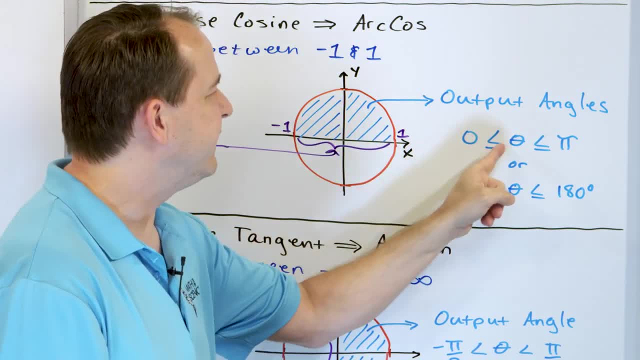 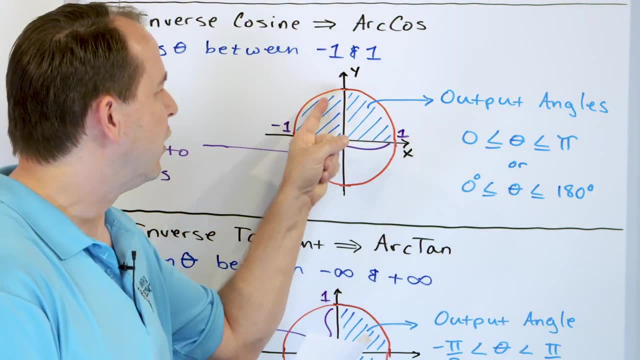 but the angles that come out are going to be in the upper half plane up here, between zero and pi. It's important for you to realize: when you take an arc cosine, hit the button on your calculator, you will always get an angle up here. You'll never, ever get an angle down here, Even though those angles down there can still give. 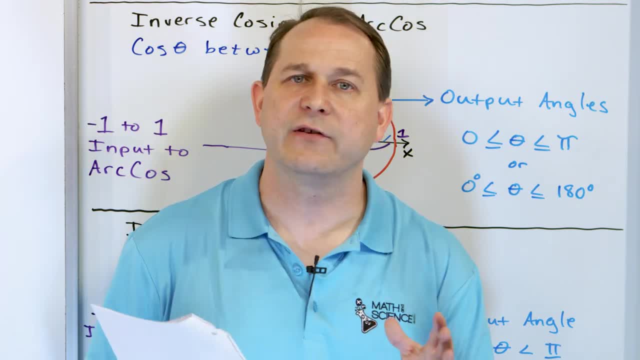 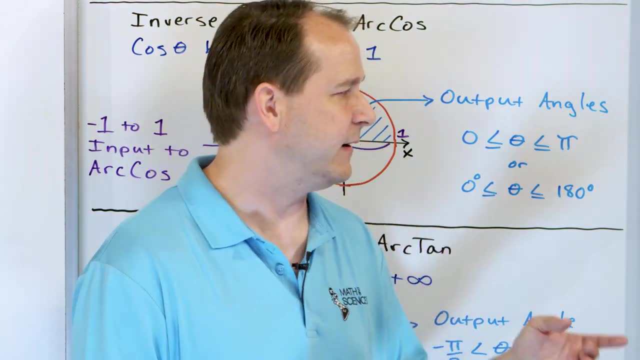 you the same cosine. we kind of lock the function down into like a base angle return. It's like the base angle that comes back, the most fundamental, the smallest angle that satisfies it will be up here. So so far, arc sine always going to give you negative one, positive one, negative one. 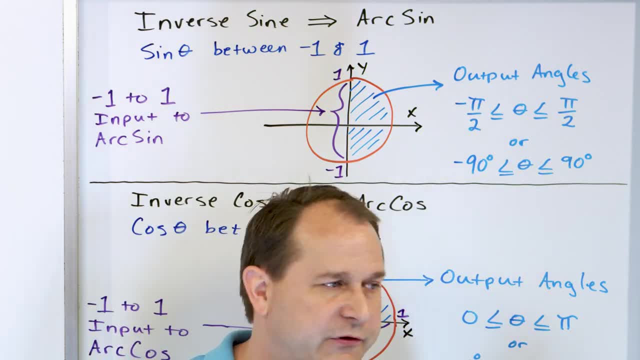 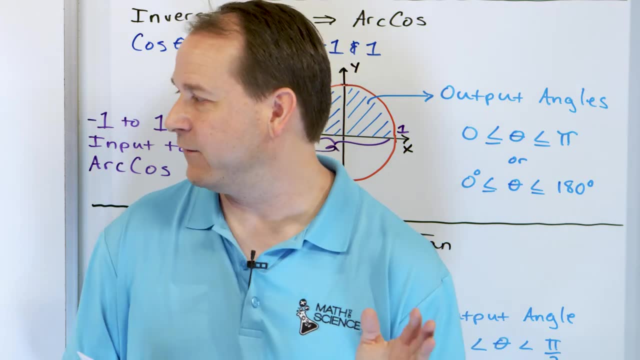 positive, one, negative one, right? So the tangent is going to give you angles in the right half plane like this: between negative, pi over two and pi over two. Arc cosine is always going to give you angles back between zero and pi. Okay, Now the tangent function is the one that's hardest to. 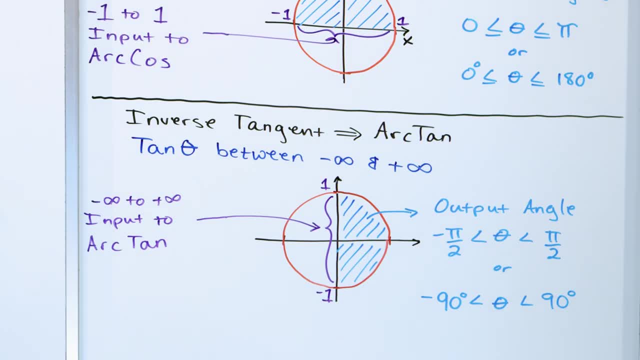 understand, and I really want you very much to understand it, So I'm going to have to do a little bit more talking. Now, what's going on here with the tangent is that the tangent can actually go between negative and positive infinity. In other words, the, the sine and the cosine. when you take 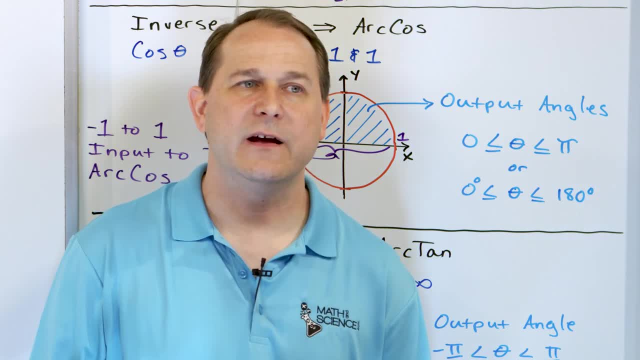 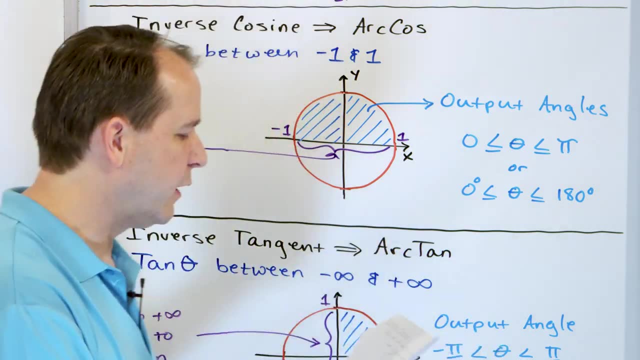 plus or minus 1.. However, with tangent you can get numbers way outside of that. Why? Because the tangent is the sine divided by the cosine. It's the sine divided by the cosine. So let's go through a couple of quick examples to. 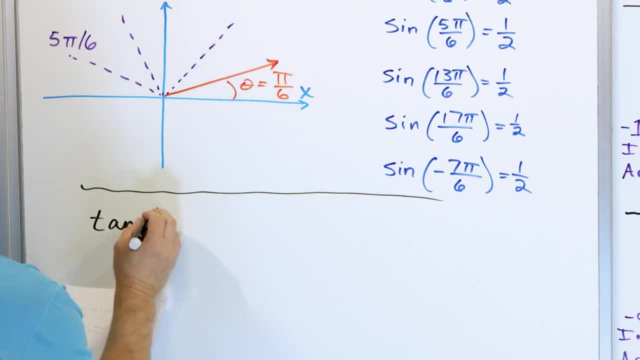 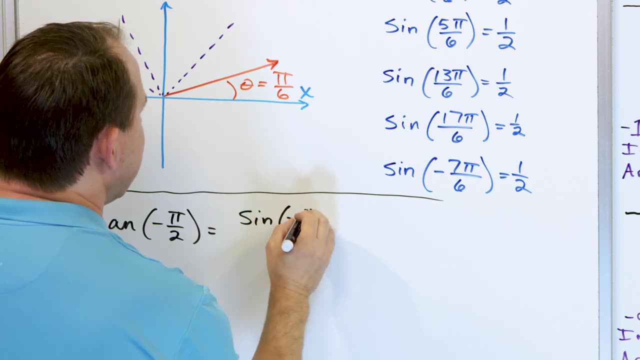 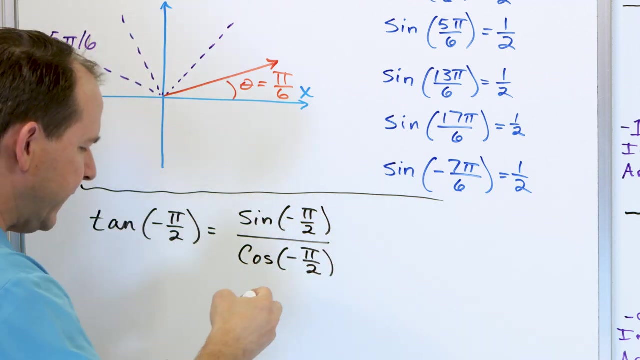 remind you of this. What is the tangent of negative pi over 2? Negative pi over 2.. It is the sine of negative pi over 2 divided by the cosine of negative pi over 2, right. So negative pi over 2 is down here, right Down here on the unit. 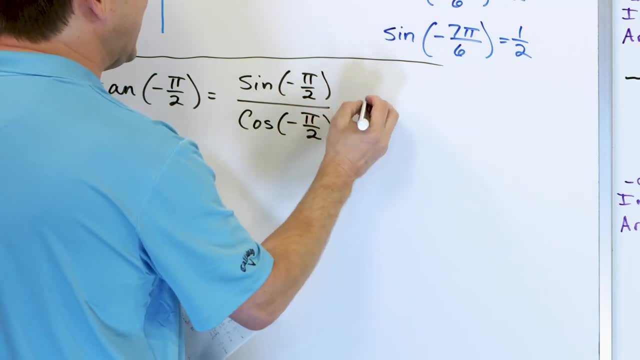 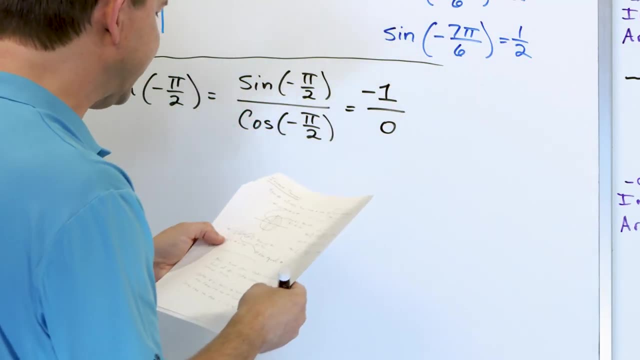 circle. So what is the sine of that? Well, the projection onto the y-axis is negative 1.. What is the cosine down here? Way down here, the cosine is 0.. Okay, so what do you have? You have negative 1 over 0.. And so what happens is the tangent. 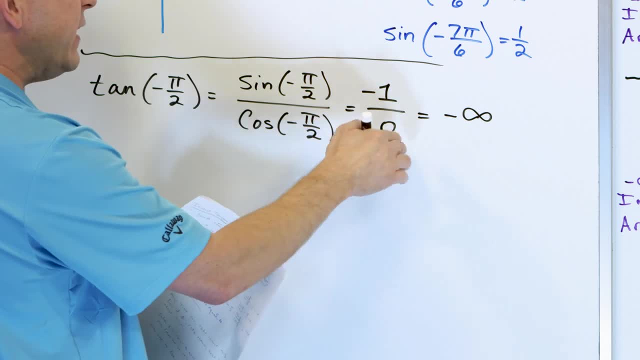 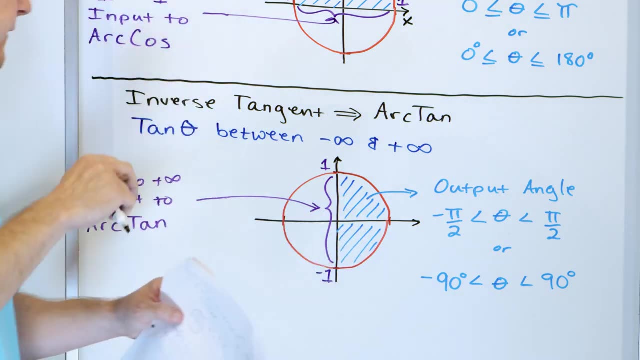 of this angle is actually negative infinity. And if, as you get away, as you get away from this negative pi over 2, like angles really close, what happens is it gets really, really, really big because of the denominator is getting really, really close to 0. So go ahead and do it, Go. 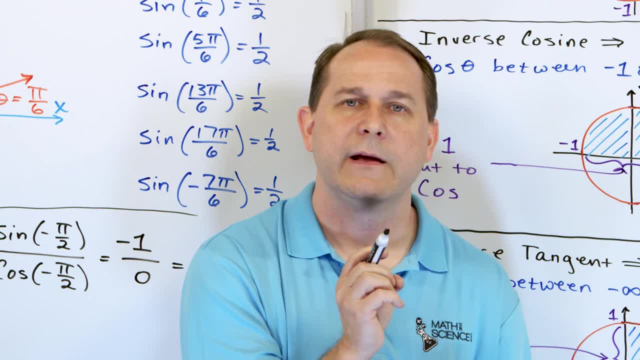 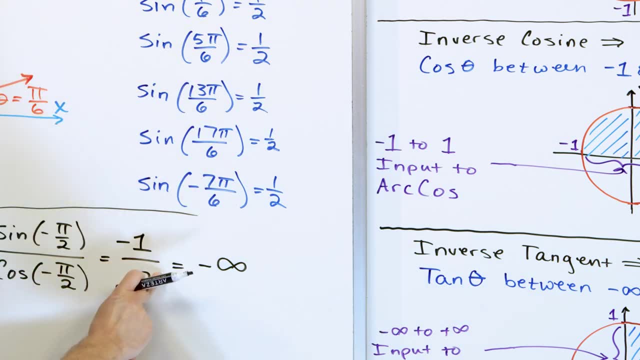 ahead and put an angle very close to negative pi over 2 in, but not quite there, And you'll see the tangents like you know: a hundred million or something. It's because the top part is approaching negative 1 and the bottom part is 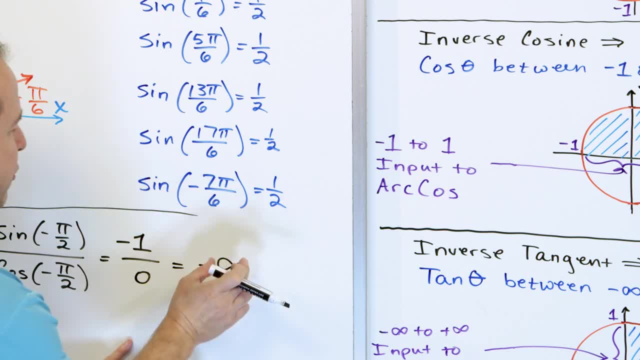 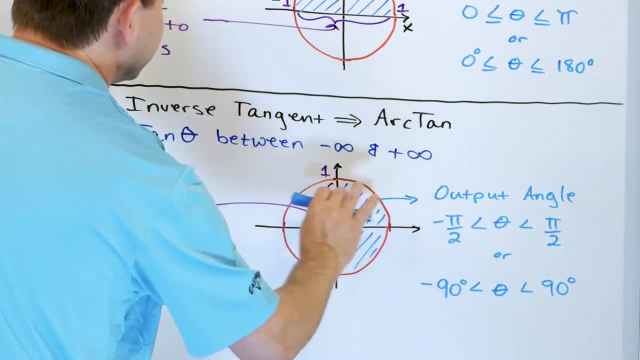 getting closer and closer to 0. So we say at negative pi over 2 you actually get negative infinity there for the tangent. Now let's take another example. We took an angle down here. Let's take the angle 0. The tangent of 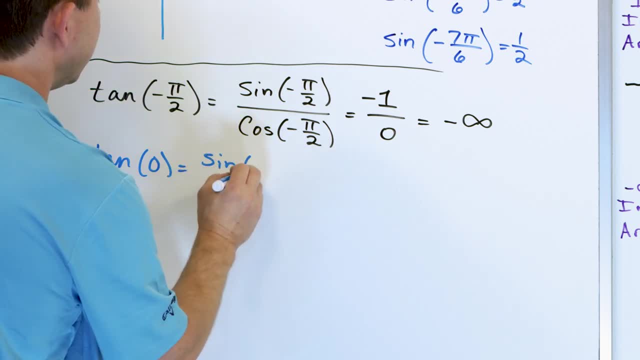 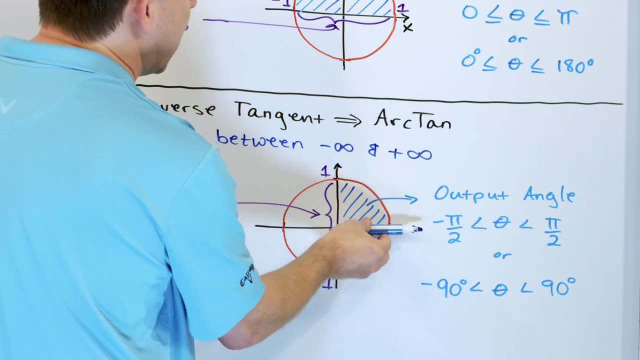 0 radians or 0 degrees. whatever is the sine of 0 divided by the cosine of 0.. What is the sine of 0? At 0. here there's no projection on y, so the sine of 0 is: 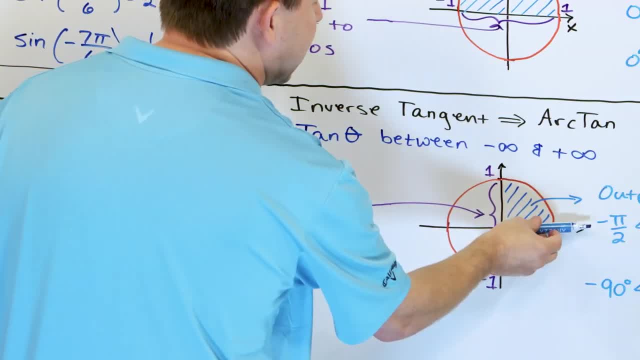 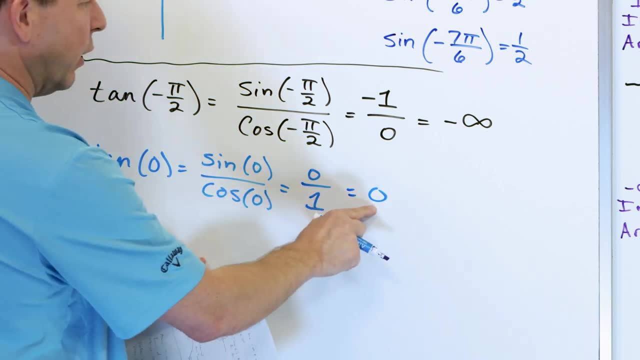 in fact 0.. Okay, and what is the cosine of 0?? The projection is on the x-axis, The cosine is 1.. So because it's 0 over 1, actually the tangent of 0 is 0.. Certainly. 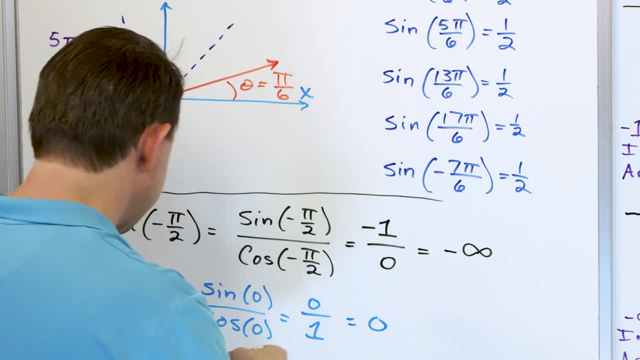 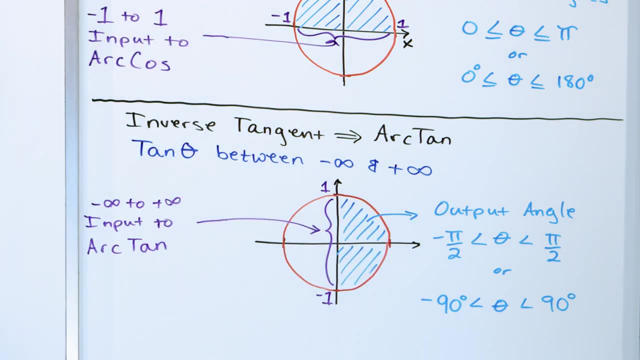 it's not infinity or anything, It's just a number. It's, it's 0.. Right Now, let's go back to the upper part. So we said: this is negative pi over 2, this is 0, this is positive pi over 2.. 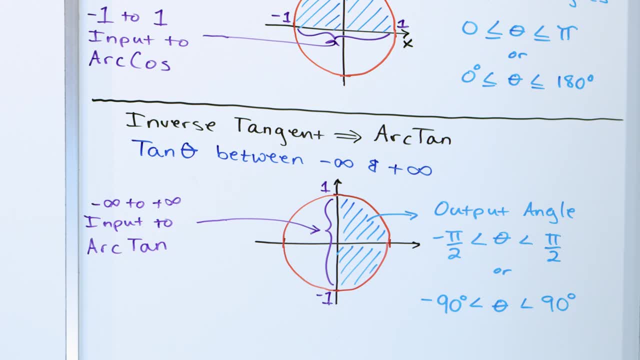 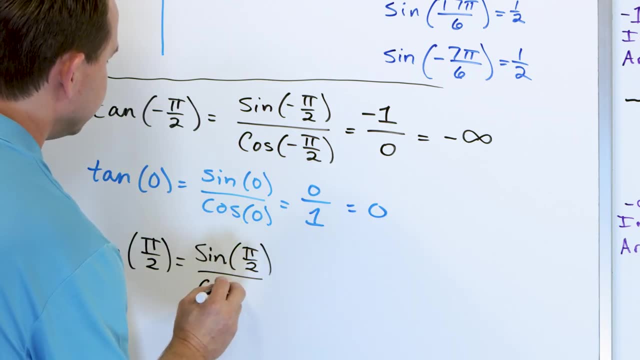 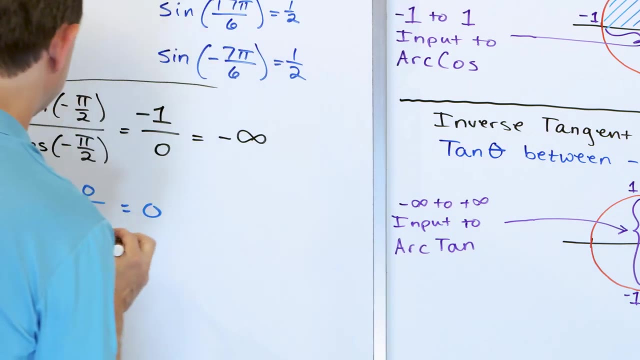 Let's take a look at what the tangent of positive pi over 2 is. It's the sine of pi over 2 divided by the cosine of pi over 2.. What is the sine of pi over 2?? Well, up here, the sine is positive 1. Positive 1.. What is the cosine of pi over? 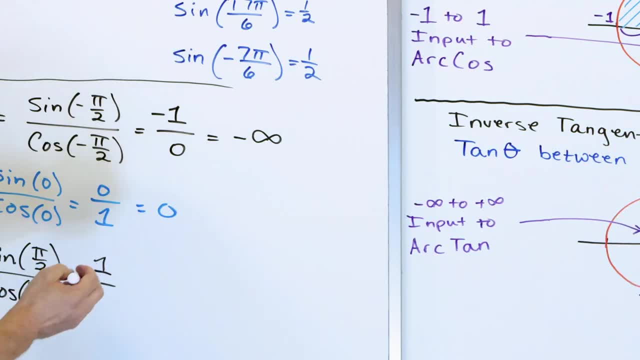 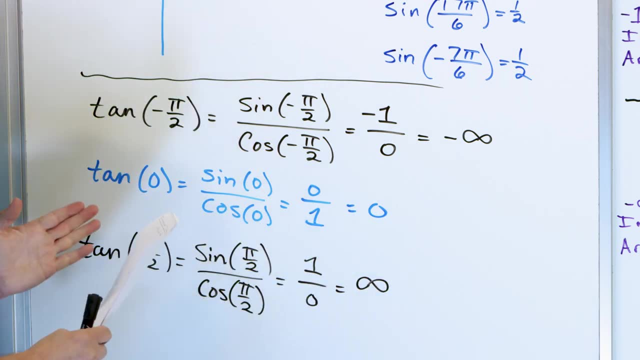 2?? Well, up here the cosine is 0. No projection onto the x-axis, so you get a 0. Positive over 0 gives you a positive infinity. So what I'm trying to prove to you through an example is the first time. it seems weird. students say: well, how can tangent 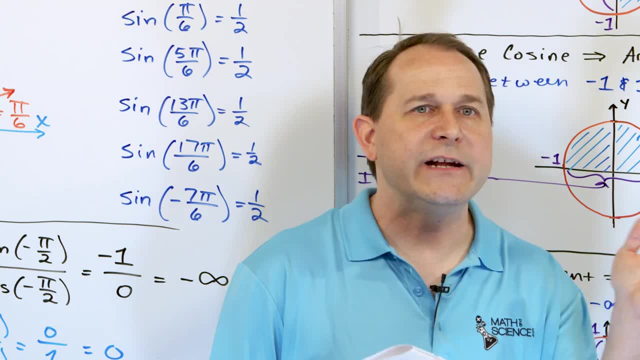 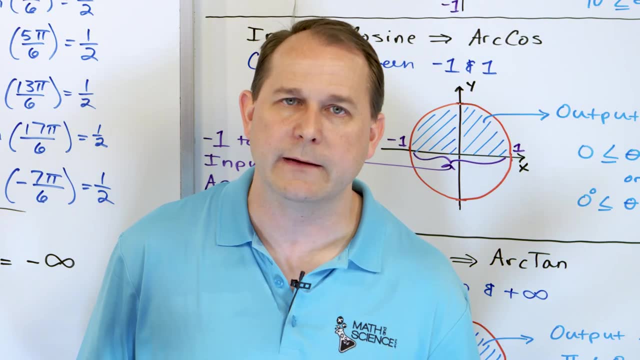 go to positive and negative infinity, but sine and cosine can't. Sine and cosine are pure projections on the x and y-axis of the unit circle, So they can never be bigger or smaller than plus or minus 1.. But tangent is not a projection. Well, it is kind of, but it's. 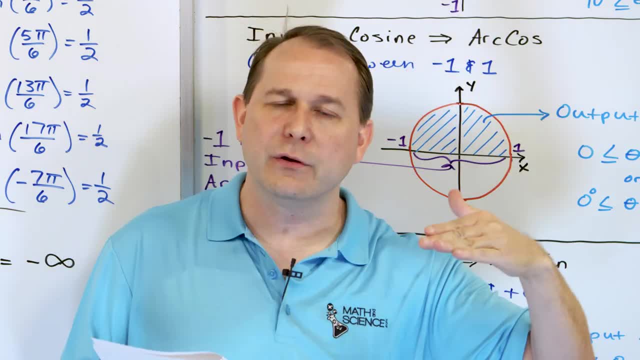 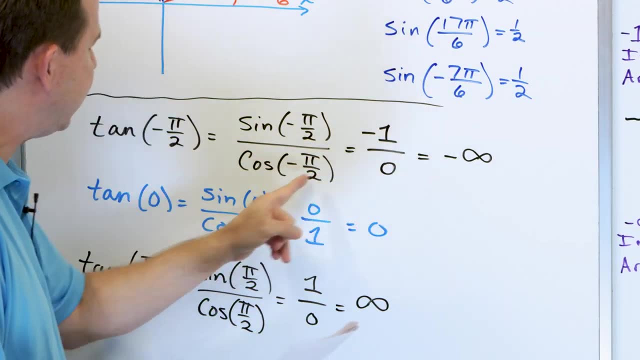 the division of two projections. So because it's sine over cosine, sometimes the cosine on the bottom can go to 0. And because of that it can drive the tangent sometimes to negative infinity and sometimes all the way up to positive infinity. So because of that I've proven to you the tangent function. 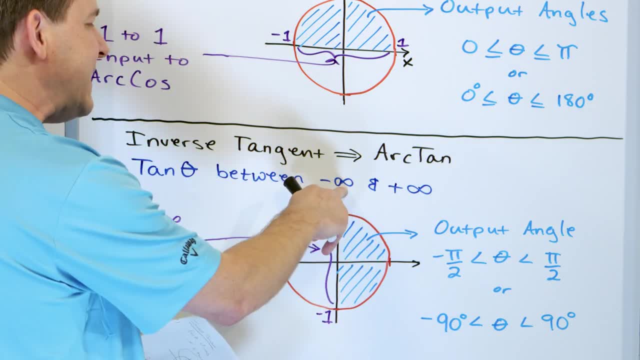 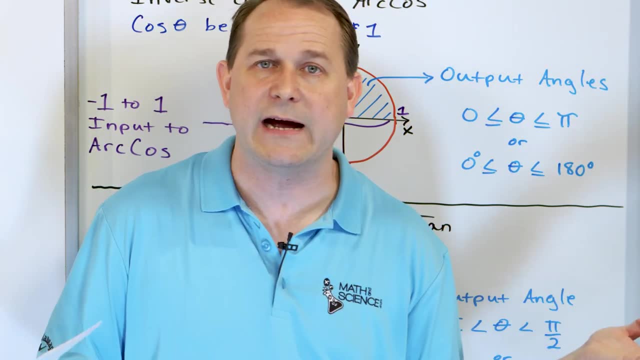 doesn't go between negative 1 and positive 1, it goes between negative infinity and positive infinity. Start typing in angles into your calculator. hit tangent over and over to different angles. you'll see that they go way outside the punya. voluntarily, Because 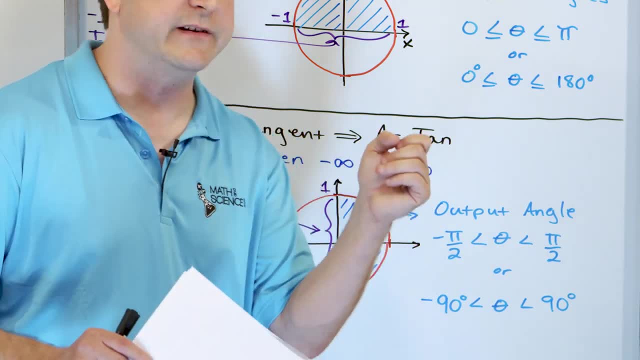 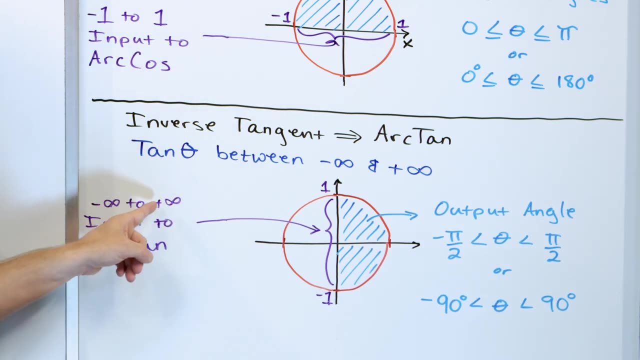 tangent can actually give values between negative infinity and positive infinity. what it means is the arc-tangent- the opposite operation- can accept as an input value values that are between negative infinity and positive infinity, And those values are going into the function. And then what I'm telling you? 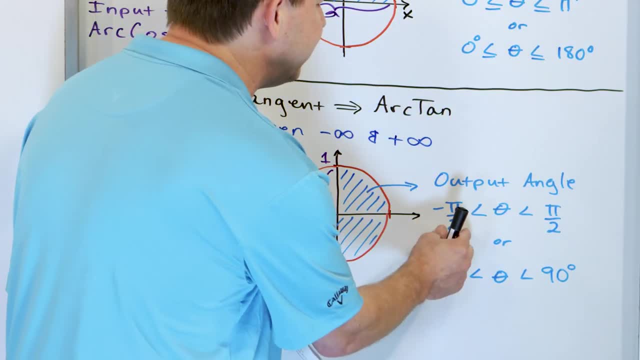 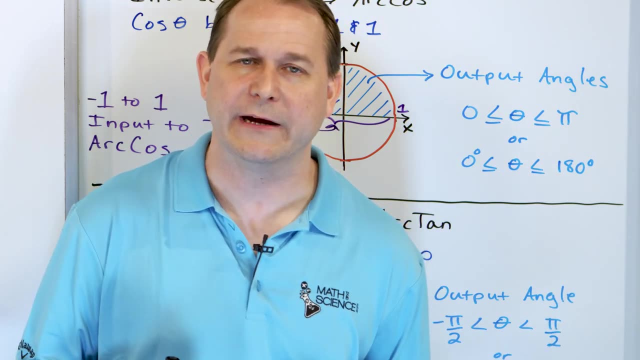 here is that the angles that come out of the function are also limited to between negative pi over two and pi over two, or negative 90 and positive 90. Why are those the special angles? Because remember the calculator or the computer or whatever is going to give you the smallest. 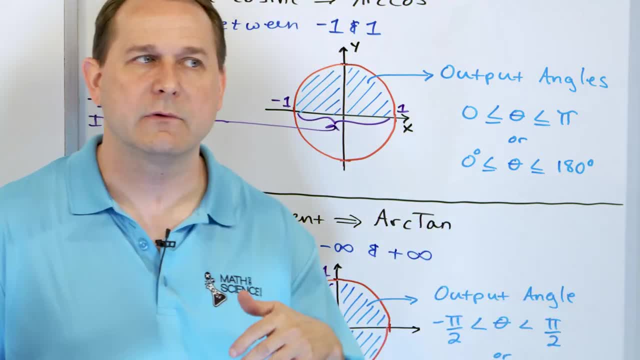 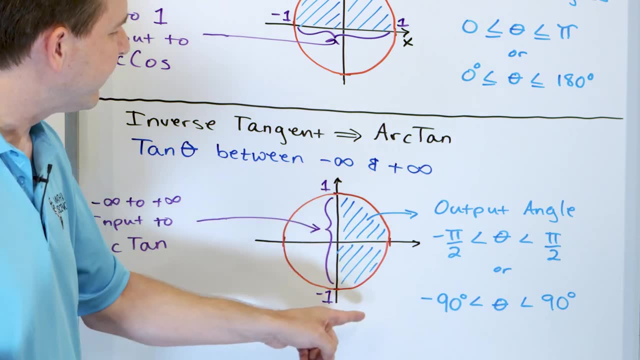 range of angles possible to satisfy the input, kind of like the input values possible. So if I put negative infinity in or positive infinity in, what are the range of angles that work? I actually just proved it to you. If we put a negative pi over two in for the tangent we actually get. 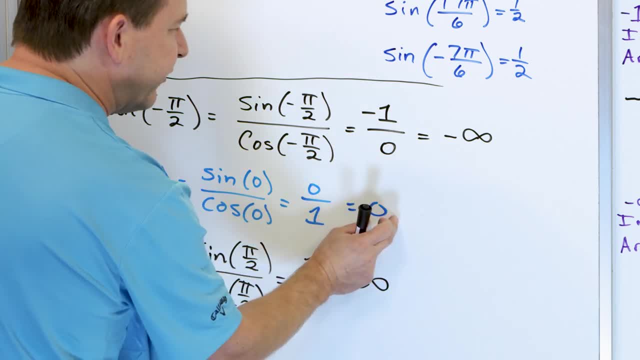 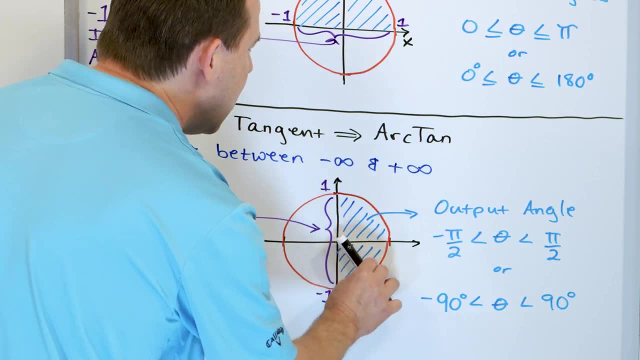 negative infinity, And if we put a zero in, we get something in the middle which is zero. And if we put a positive pi over two in, we actually get a positive infinity. So these angles here, from negative pi over two up to positive pi over two, cover all the possibilities. 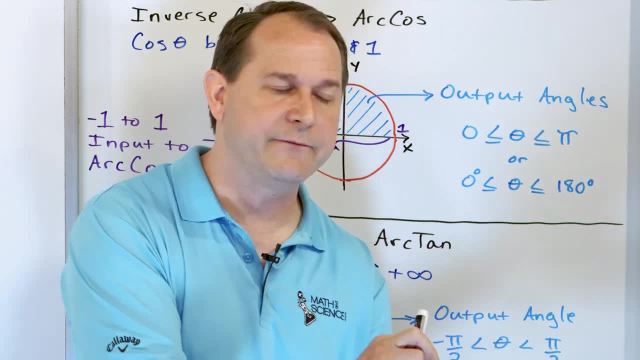 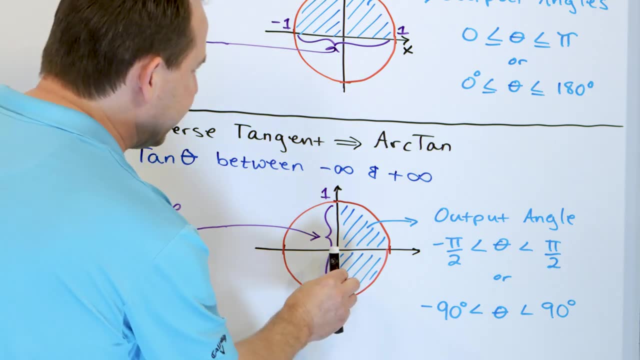 Derek, such a genius of where tangent can go from negative infinity up to positive infinity. Think about it. anything from here on up to here, the tangent here is negative infinity. make sure I'm right here. The tangent here is negative infinity, The tangent here is zero and the tangent 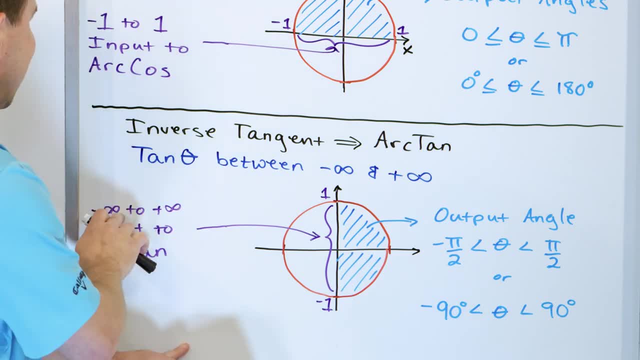 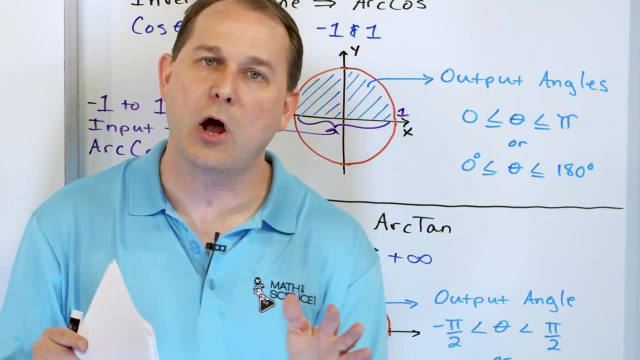 here is positive infinity. So these angles cover all the possibilities. any number you can think of Sticking into a calculator hitting inverse tangent, These angles will cover it and they're the smallest angles that will cover that range. So we say the inverse tangent. 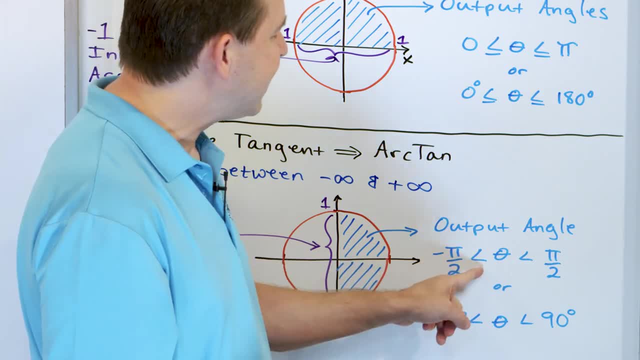 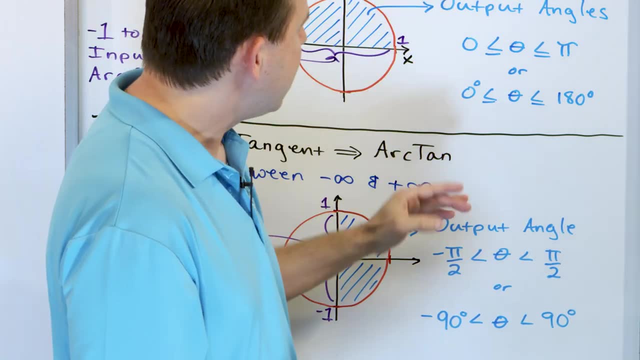 take as an input any number you want to put in, and they can spit out as an output anything between negative pi over two and pi over two. now, usually you see up here, i have the equal signs and i have the equal signs, but for the tangent. we don't usually put the equal signs because we don't. 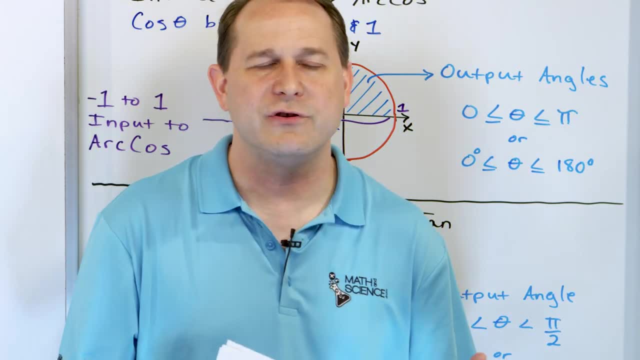 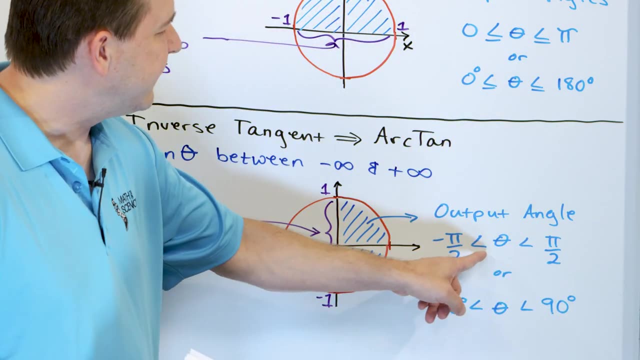 like to deal with infinities in real life. so we say the inverse tangent. i mean your calculator is really never going to give you infinity back. i mean infinity is an infinite number, it never stops. so we really say the inverse tangent goes between negative pi over 2 and pi over 2 as its output. 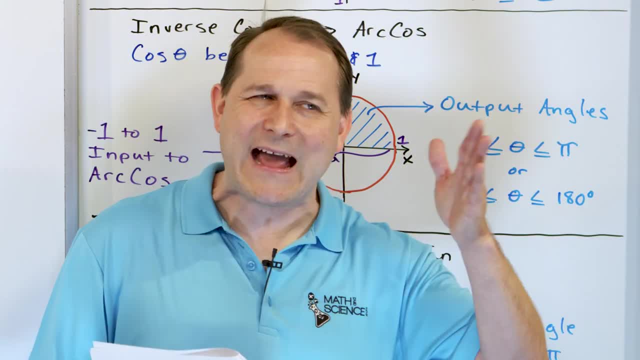 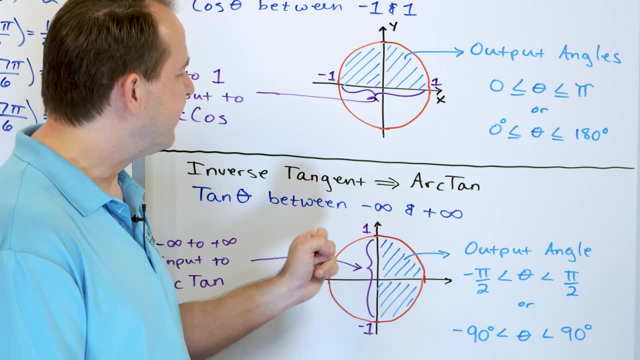 functions as its output angles, but not exactly including like it gets incredibly close to negative pi over 2. it drives it up super high, basically to infinity, all the way up to positive pi over 2.. so let me read my notes and make sure i didn't forget anything anytime you take the 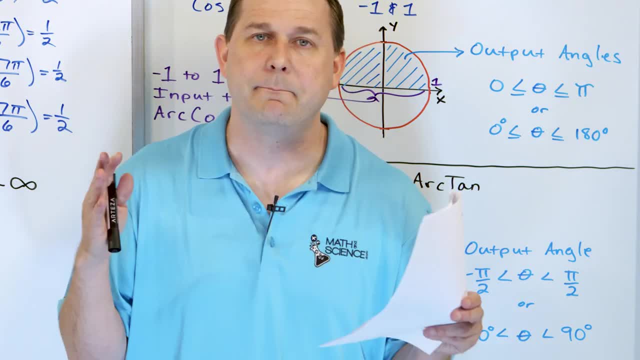 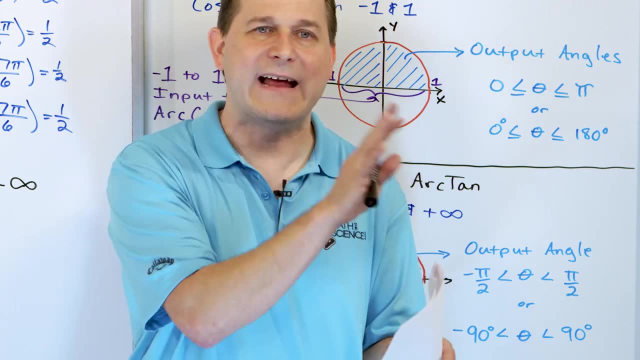 inverse trig function of a number. the calculator returns a base angle which is like the smallest angle possible to satisfy, uh, the smallest angle possible to satisfy what you gave it as an input. okay, other angles exist around the N. sug teseク shenы йогоa au Drag. 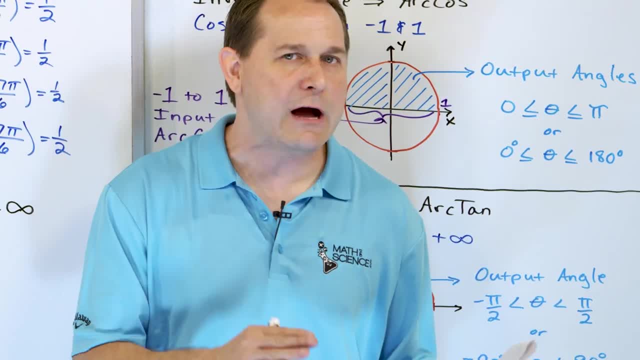 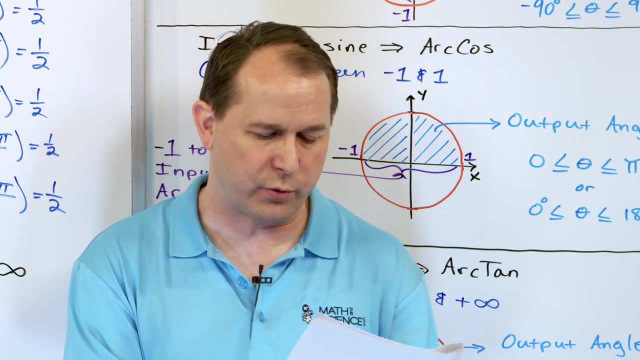 usb circle that have the same sine or cosine or whatever. but the calculator doesn't return all those angles because there's an infinite number of them. It returns the smallest angle possible. which are these ranges? I've written on the board here, So sometimes when you're 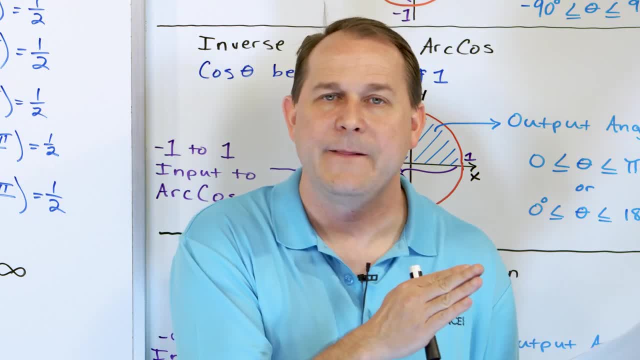 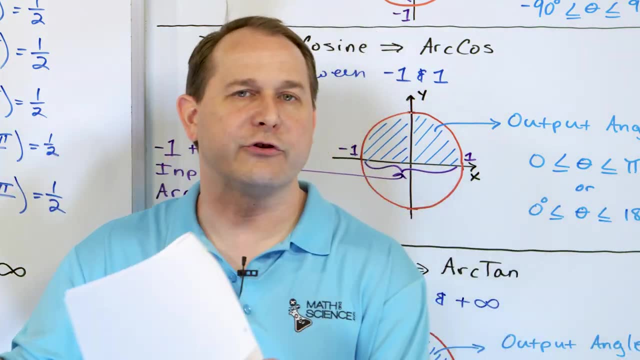 solving equations. what you'll do is you'll get the base angle back, the fundamental angle, and sometimes you might have to add or subtract 180 degrees or 360 degrees to go into another quadrant, depending on what the problem is telling you to do. And we will solve problems like that. 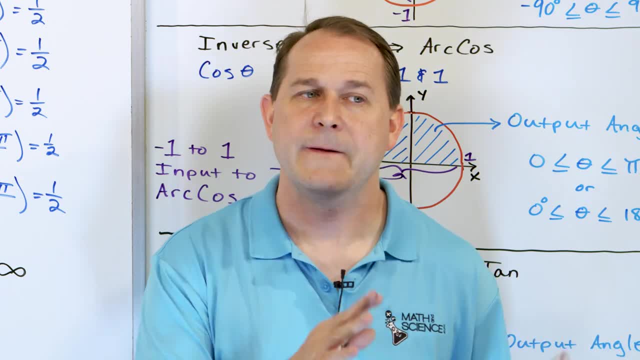 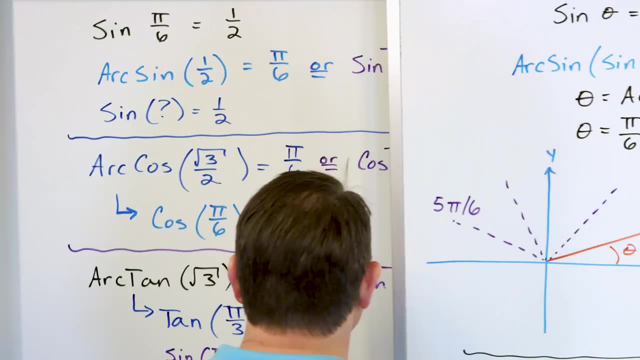 later, but the fundamental base angle of what your calculator will give you is going to be given by these terms here. So what I want to do? I think this was a really long lesson, but I want to go through it all real quick at lightning speed, to make sure we're all on the same page, okay. 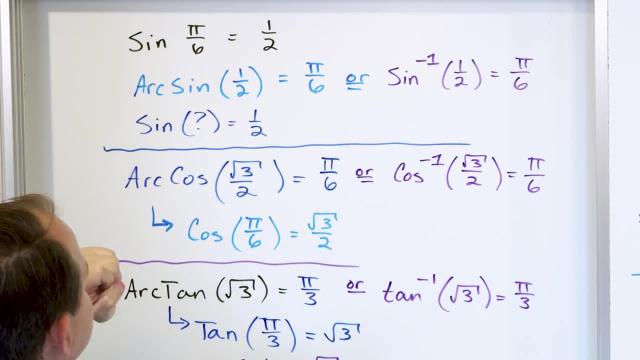 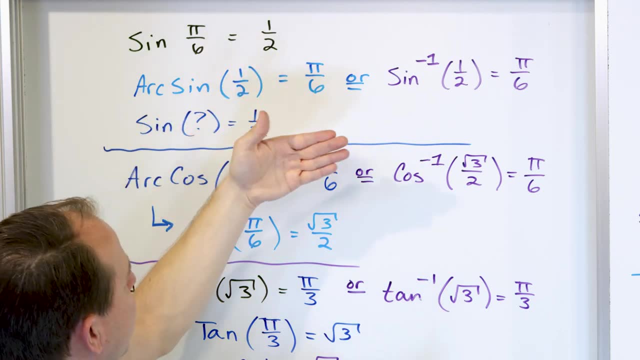 So we know that the sine of 30 degrees pi over six is one half. So we define an inverse going backwards, where the arc sine of the right-hand side gives us an angle back, And so it gives us an angle back and we can also write it as the inverse sine with the negative one, but that is. 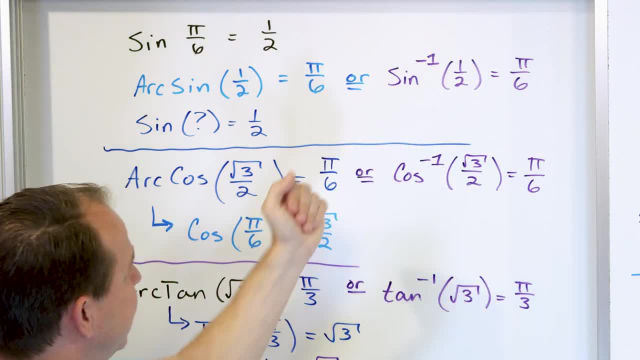 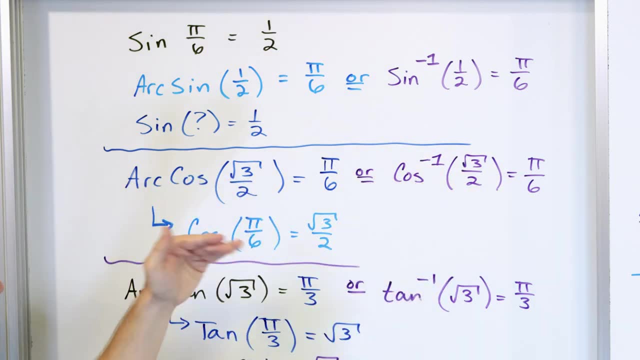 not an exponent. Don't treat it like an exponent because it's not, but you might see it in books like this. The arc cosine of a number gives us an angle. back can be written in a similar fashion. So numbers come in, angles come out. Same thing with the arc tangent numbers come in. 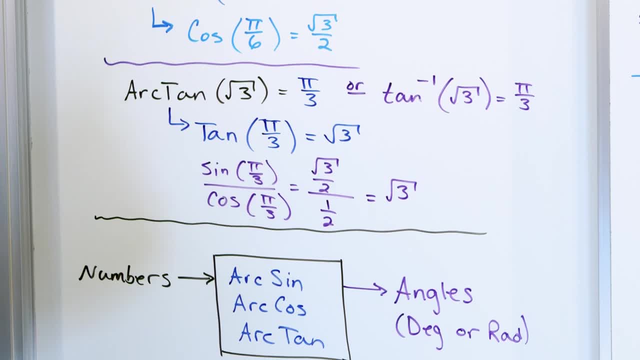 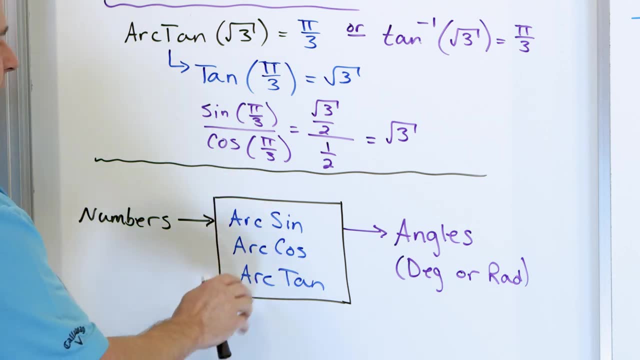 angles come out, and we can write it with the minus one up there just like before. So graphically, numbers come in arc inverse sine cosine tangent, arc sine cosine tangent are in here, and angles come out- degrees or radians. So then we start asking ourselves the 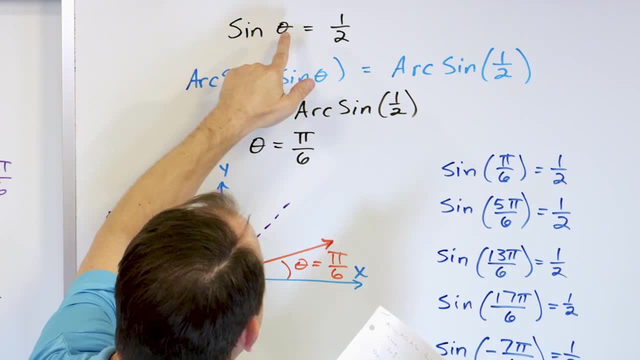 question. going back to our first question, what is the inverse sine of the right-hand side of the right-hand side of the circle? And we have a fundamental example: Sine of an angle is one half. What angle works? So we apply the arc sine to both sides, solve and we basically want to. 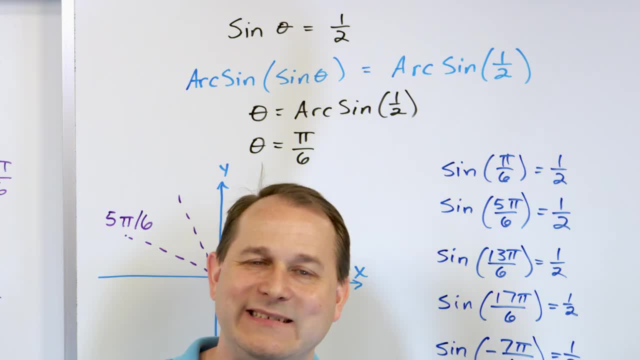 figure out what the arc sine of one half is. That means what angle exists, so that I take the sine of that angle and I get one half. Well, you know it's 30 degrees, You know it's pi over six. so we put. 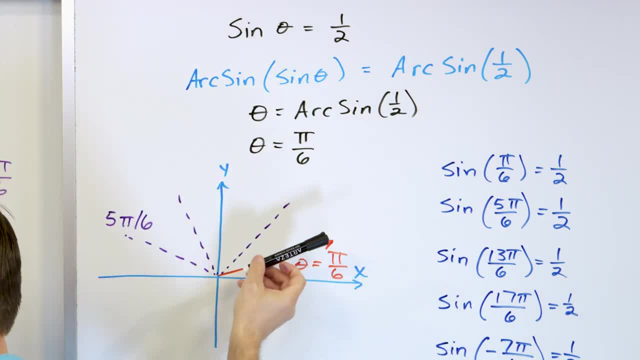 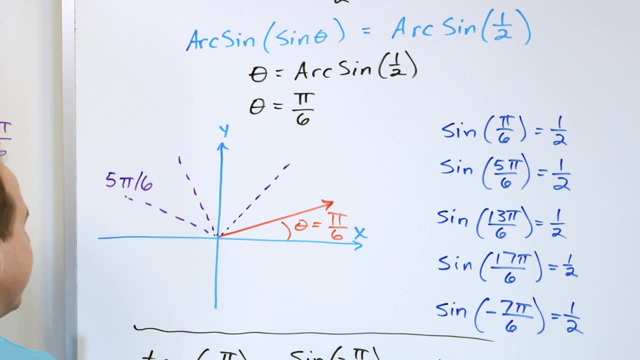 pi over six there, which is right here in the unit circle. But then we realize, wait a minute, there's other angles, because this angle also has the sine equal to positive one half. And then we go even further and say, well, wait a minute. 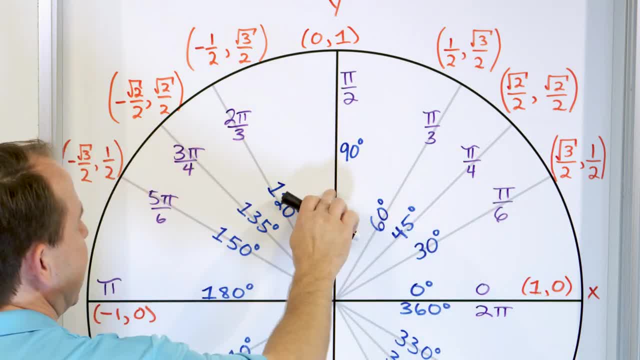 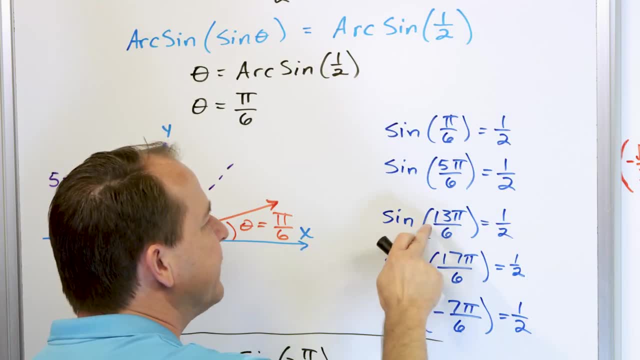 Not only Is the sine of pi over six equal to one half And the sine of five pi over six also equal to one half, But if we spin around the unit circle to here, then we see the sine of 13 pi over six is. 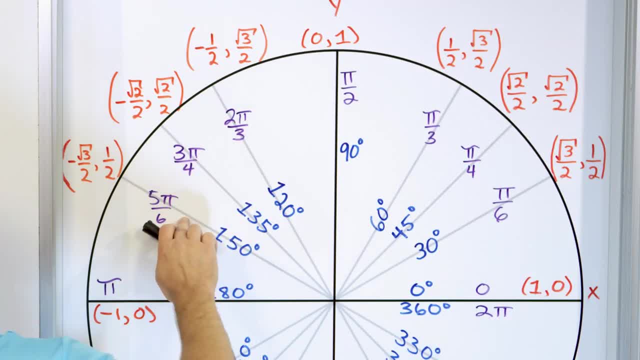 one half. And if we spin around the unit circle to here- another revolution- we see that 17 pi over six, the sine of that's one half. Even going negative to negative, seven pi over six, the sine of it, the projection is always in the same place: one half. So what angle does the calculator give? 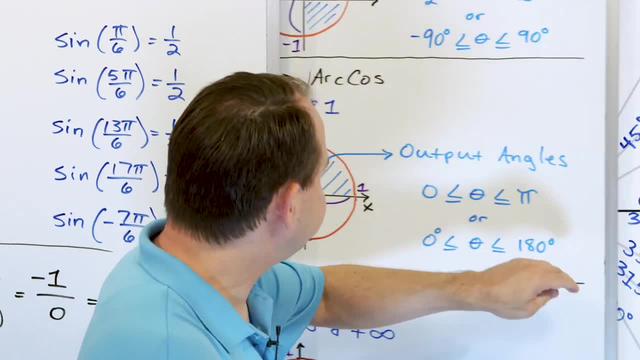 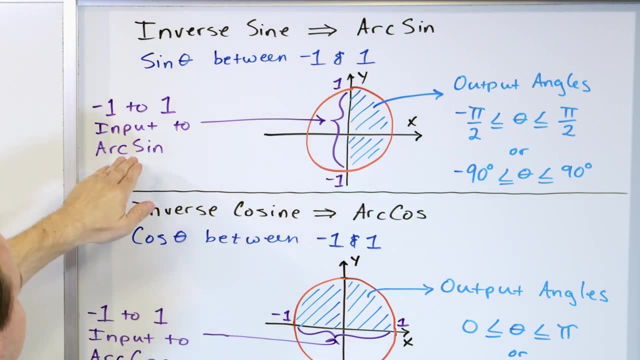 you. That's what the rest of the lesson was about, And we said That for the sine function it only gives values back between negative one and positive one, So the inputs to the arc sine can only be from negative one to positive one, which are projections on the. 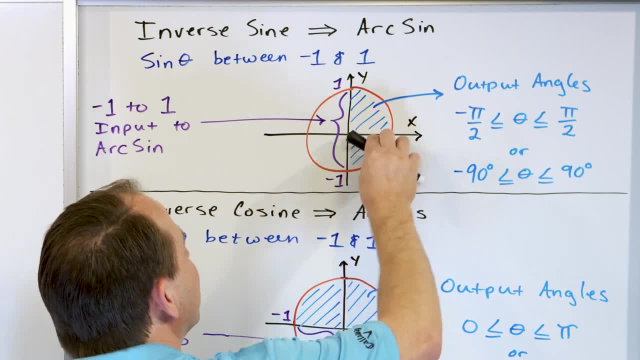 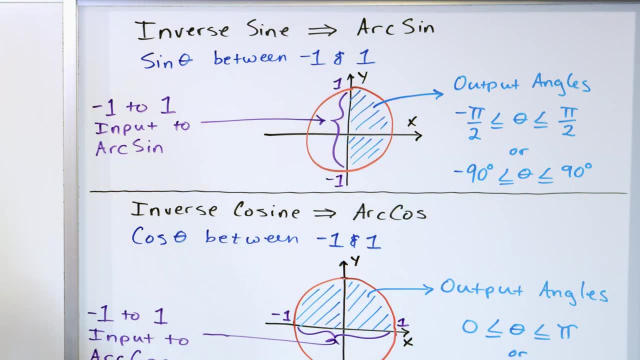 y-axis between negative one and positive one. That means the angles- the smallest ones that will work for this projection- are always going to be between negative pi over two and positive pi over two, just like this For the arc cosine. it also gives numbers between negative one and. 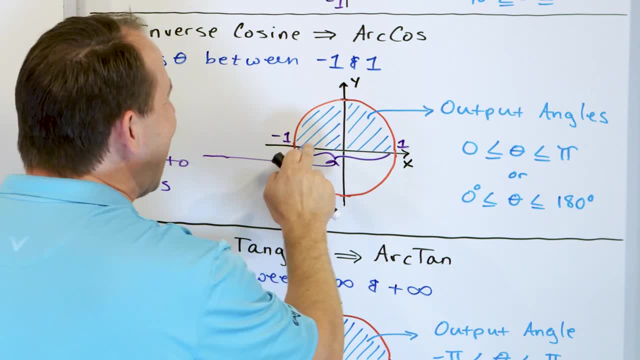 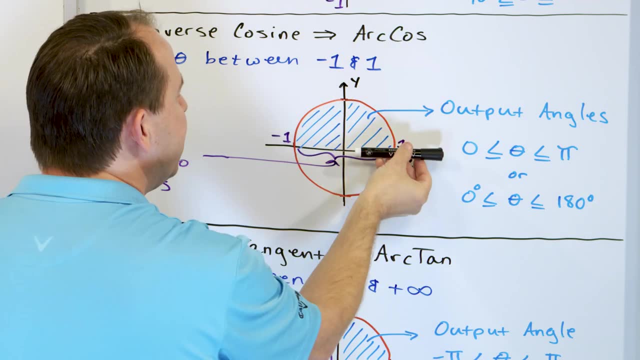 positive one. So the inputs to the arc cosine is on the x-axis and the inputs to the y-axis is on the y-axis, between negative one and positive one. These are the projections on the x-axis, And the angles- the smallest set of angles that work, are going to be between zero and pi, which is zero, and 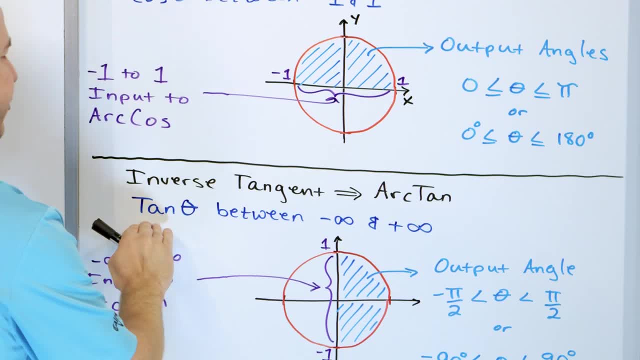 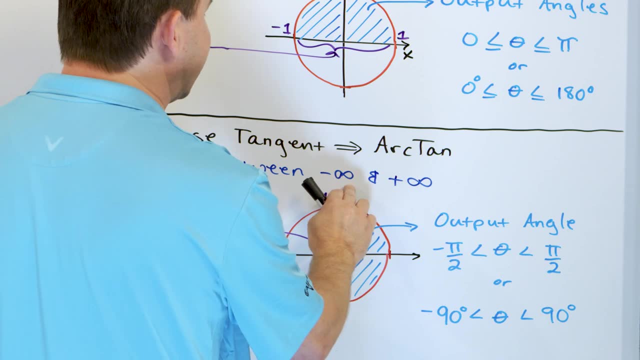 180 degrees. Then we said the tangent's the weird one. It actually can take values as inputs between negative infinity to positive infinity. or I should say the tangent gives values back between negative infinity and positive infinity. So the input to the arc tan can be numbers from negative. 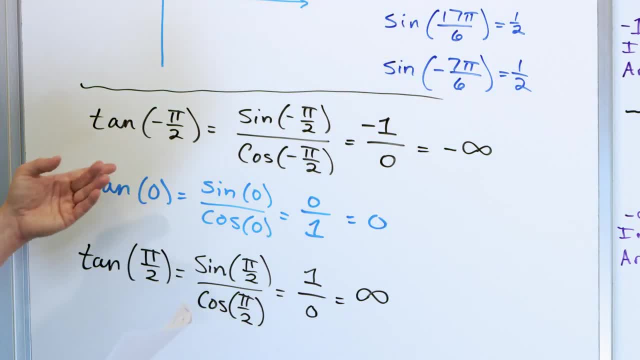 infinity to positive infinity. And we've already described why here. It's because it's the ratio of two trig functions. so the input to the arc tan can be the input to the positive infinity. So the input to the arc tan can be the. 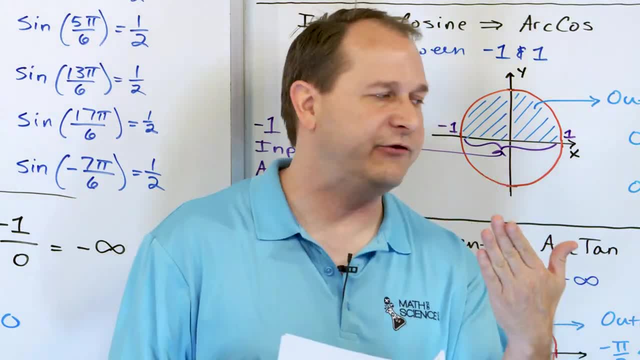 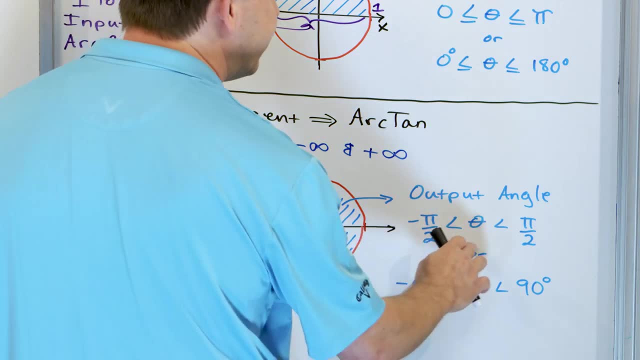 So sometimes that denominator goes to zero, which drives the tangent to infinity. So if the tangent can go between negative infinity, positive infinity, it turns out that the set of angles that allow that to happen are also between negative pi over two up to positive pi over two. 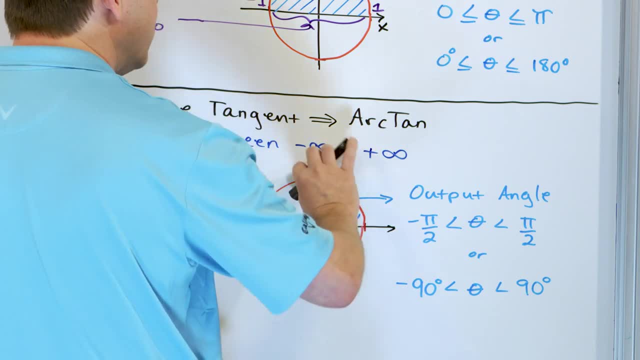 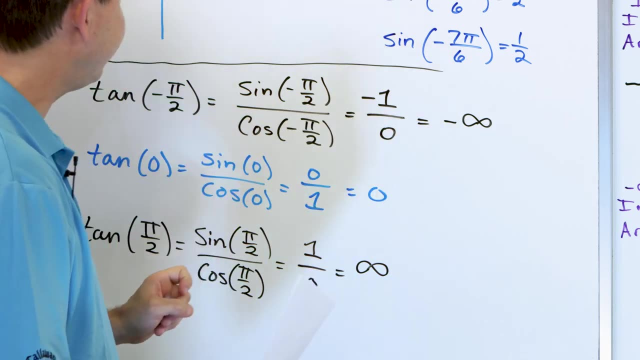 Not inclusive, because we really don't want to get to infinity, But anyway, those are the boundaries there. Why is that? Because the tangent of negative pi over two is the sine over the cosine which is negative infinity, and the tangent of positive pi over two is the sine over the cosine which 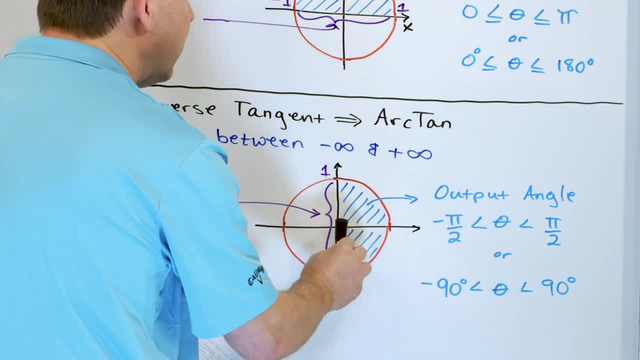 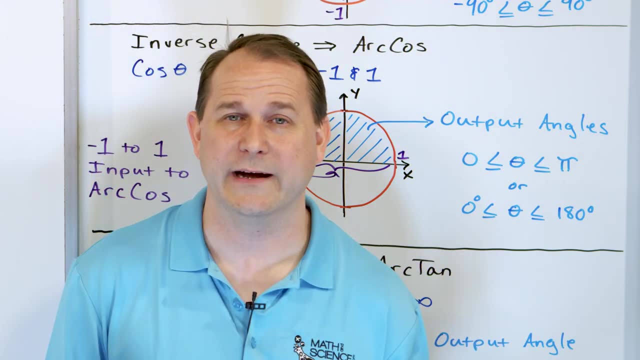 is positive infinity. So this set of angles from here to here is the smallest set of angles, such that the tangent goes from negative infinity to positive infinity. Now, that is a ton of talking. It's a lot of talking, And that's why every book I've ever opened it makes it incredibly hard to understand. 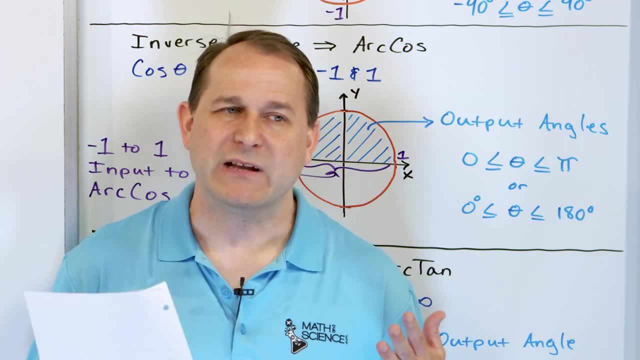 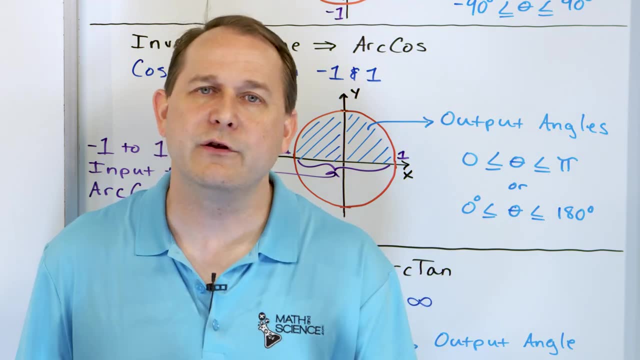 what they're doing, because it's hard to describe in words, But fundamentally that's what we're going to do. So, as we solve problems with the inverse sine or the inverse cosine or the inverse tangent, What we're going to do is try to figure out the angles that make the equation work. 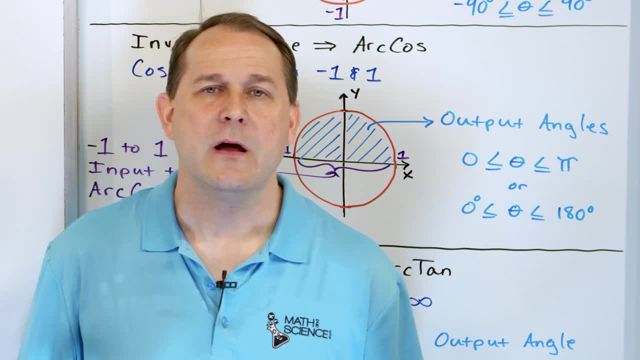 We want to solve for the angle, because the angle is what comes out. But the angles that come out of an arc sine are only going to be in this range And the angles that come out of an arc cosine are only going to be in this range. 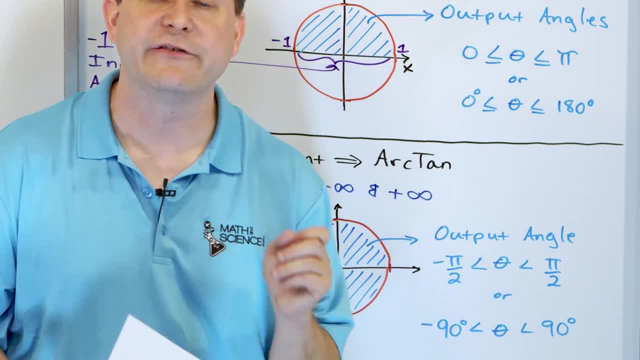 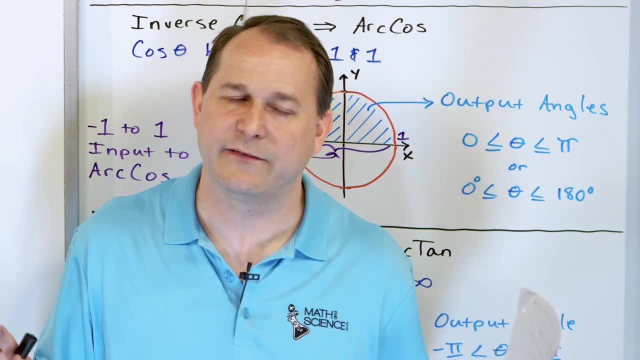 And the angles that come out of an arc tangent are only going to be between this range, And so we're going to have to keep track of that as we solve our problems, And we will be doing that in the future lessons, So make sure you understand this as well as you can.